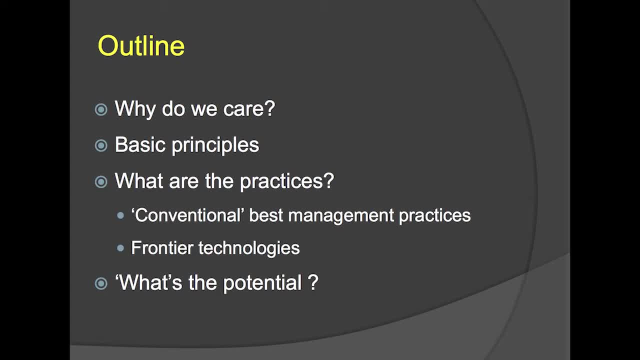 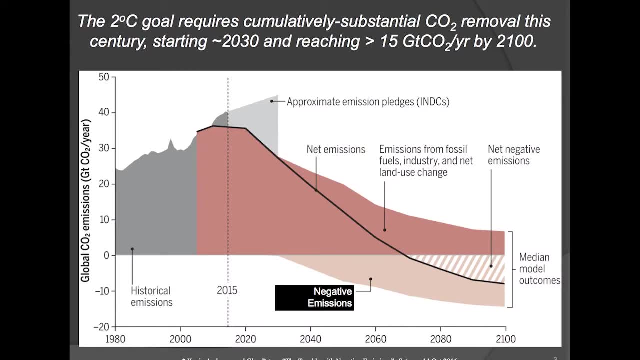 And then I want to sort of finish up really saying, well, what do we know about the potential and and what does that mean kind of going forward? So this, this graph here is is intended to kind of illustrate the potential or the issue of why a lot of the soil is going to be generated. 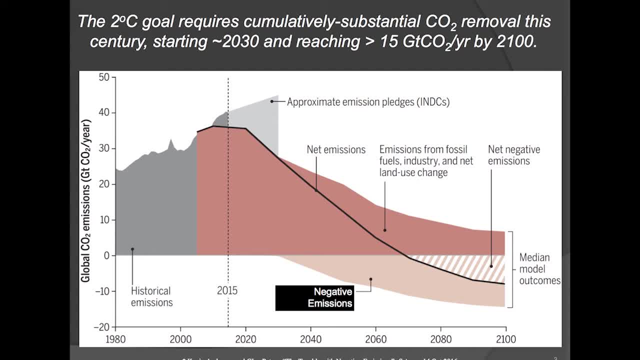 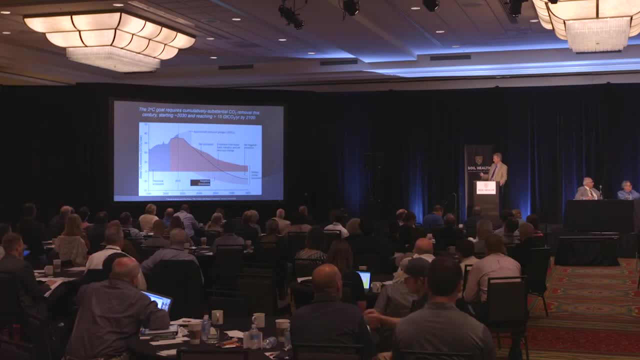 lot of people now who really hadn't thought a whole lot about soil, carbon and agricultural soils in general, are really interested in this topic now, so I'll see if I can point over here. and so basically this looks at global emissions in co2 equivalents gigatons, which are billions of tons per year, and and then 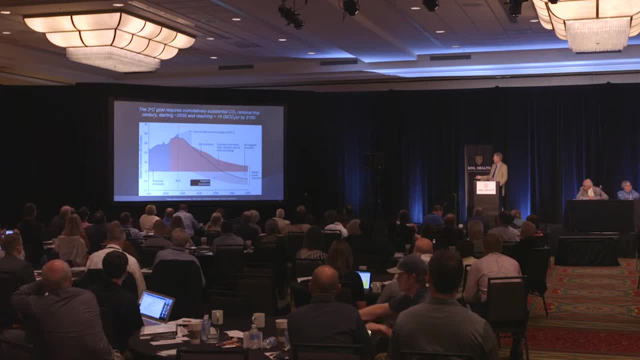 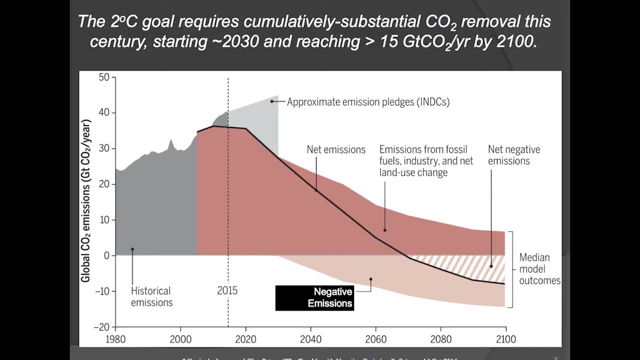 down here on the x-axis. we've got time so we can see where we're here right now, a little bit after, I guess two years after 2015- when the slide was made in a science article, and this black line here represents the, the emissions profile. 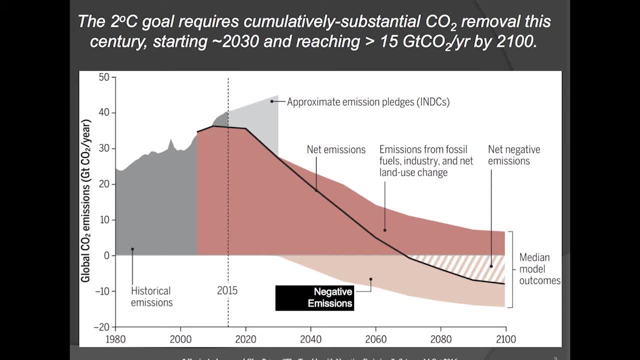 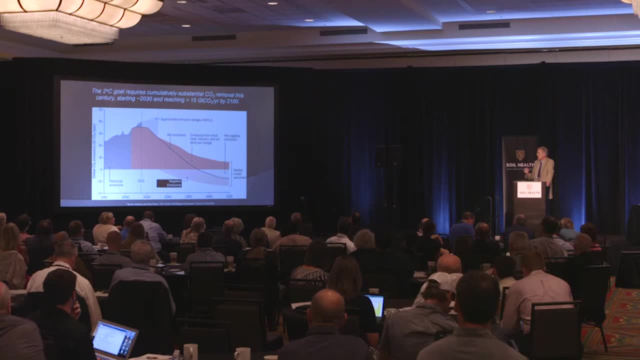 that we will need to to attain in order to meet this Paris, less than two degrees warming of in terms of the, the mean global temperatures. so what? what really came out in the, in the, in the IPCC fifth assessment a couple of years ago, when they started looking at all the kind of integrated assessment models to say, gee, what if we? 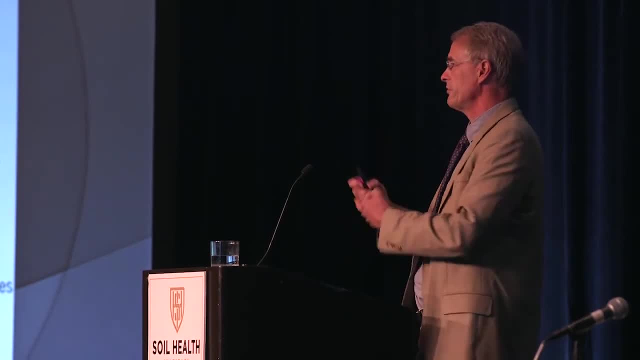 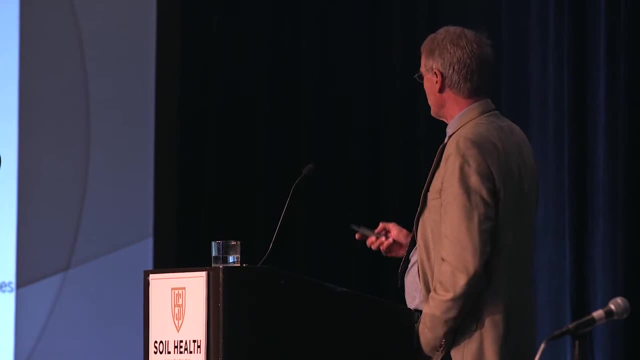 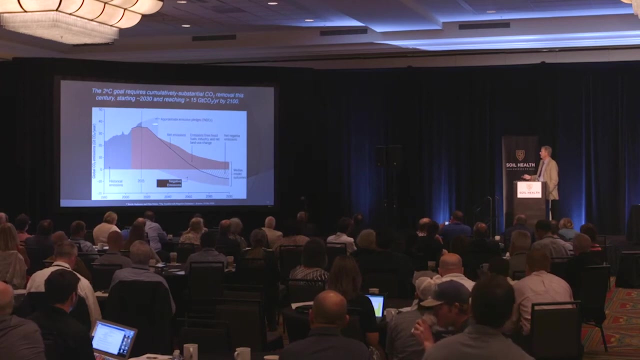 do this to to decrease fossil fuel emissions and and looking at all the greenhouse gas sources, etc. what are the emissions profiles look like going forward in time? and this is kind of a an aggregate of that, and the bottom line is that, if you look at this so 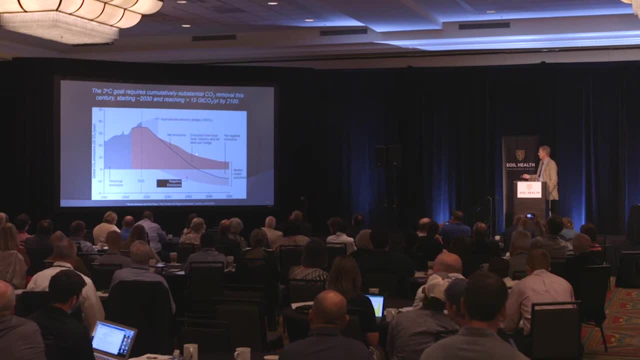 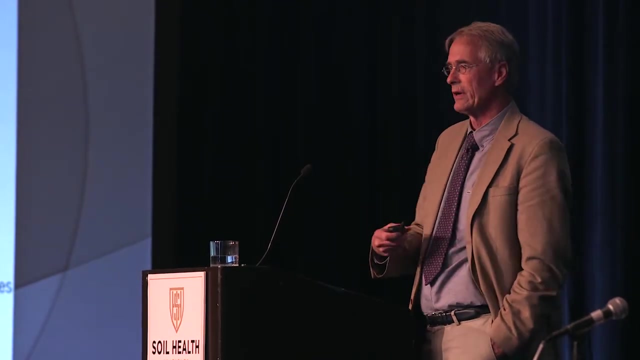 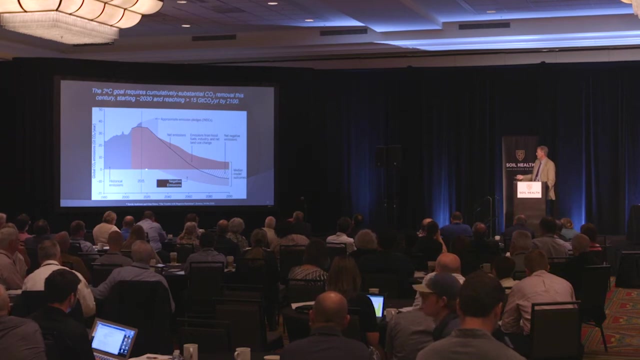 yeah, we need to decrease emissions of fossil fuel, co2, but in order to follow this trajectory, that's not enough. so we need to actually have carbon dioxide removals from the atmosphere in order to not overshoot this goal, and so this idea of negative emissions come in. and you see that, in order to meet this goal, 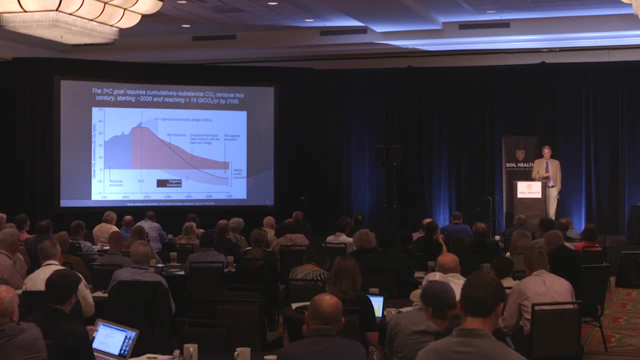 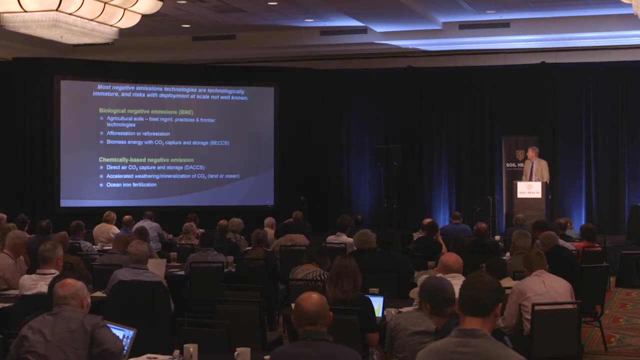 basically all the models said we can't really do it with just emission reduction. we've got to have negative carbon emissions, okay. so there's a couple different ways that you can do this. you can do biological negative emissions or carbon sequestration. you can do chemical. 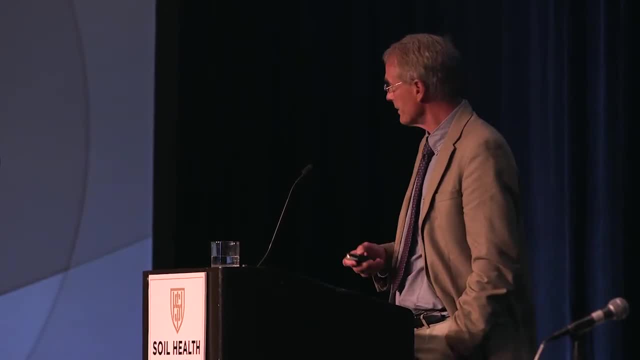 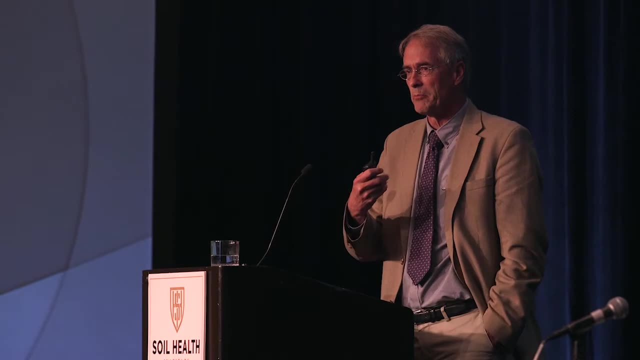 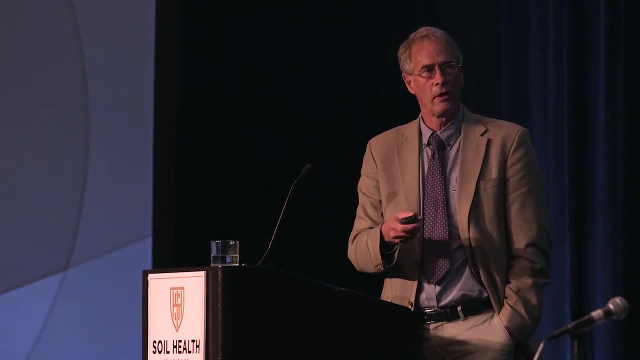 reductions and and and. there's different ways. you know, if we look at the biological, you can have a forest baby, you can. you can use biomass in power plants and capture the co2 and then put it down into geologic reservoirs, chemical-based things. 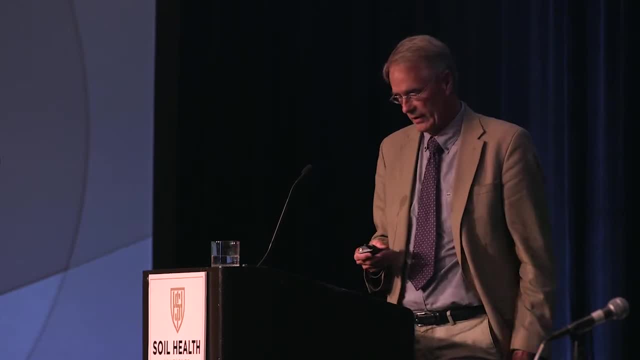 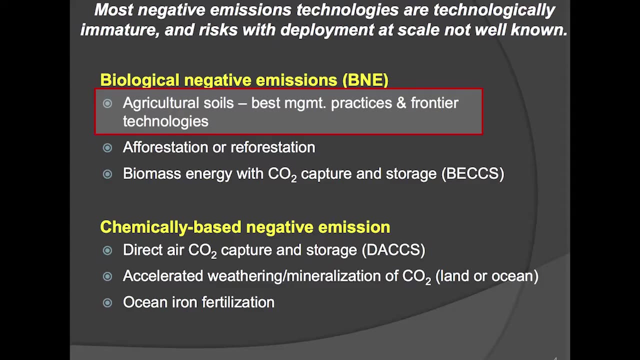 We can have direct air capture and storage, et cetera. But I think the key point now is: a lot of people have said, gee, agricultural soils are one of the opportunities to remove CO2 that's out there, that is cost-effective, that we can potentially move on now. 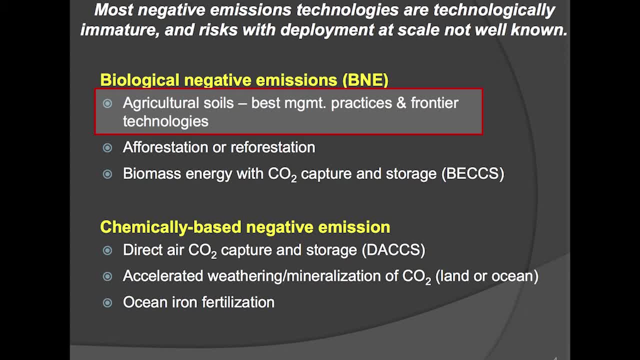 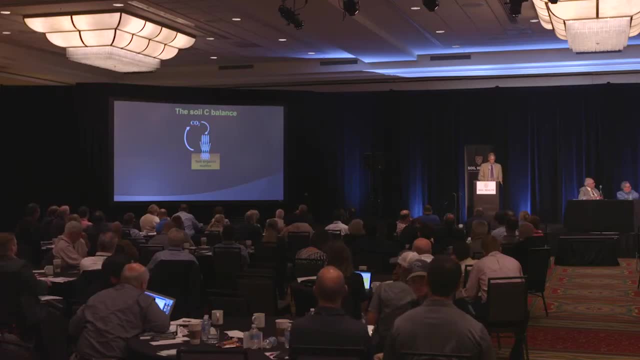 So there's a lot of interest now in the global climate change community if you will looking at agricultural soils and carbon sequestration. So that's a little bit of the background on the why. why the intense interest now. So just kind of reviewing the soil carbon balance really quickly. 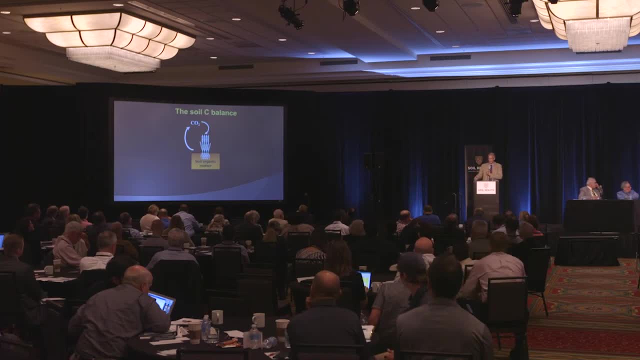 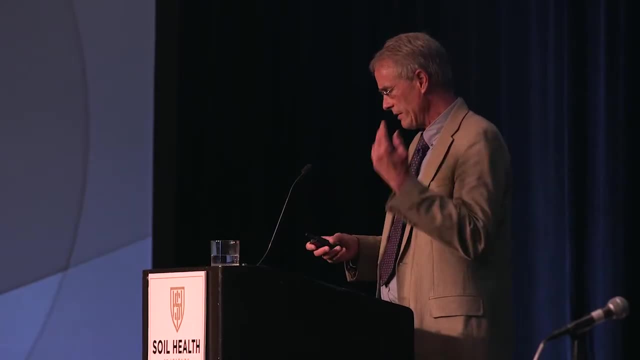 And it is a balance okay. So we've got carbon coming into the soil through fixed-by plants and the plants die and there's crop residues or plant residues, And then there's respiration and CO2 emissions by the soil biota. 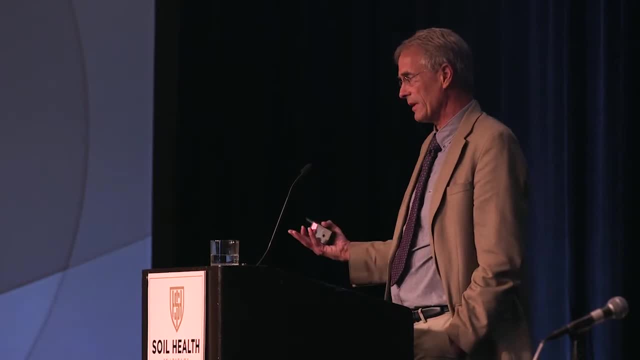 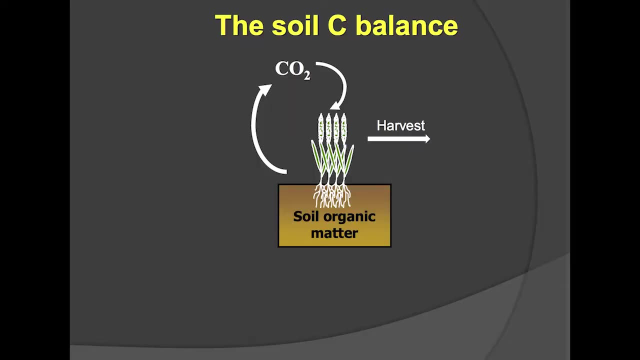 And of course, if we're looking at agri-ecosystems, we affect this carbon balance in a big way by removing a lot of that fixed carbon in the harvested product. So we want to sequester carbon here. What do we do? 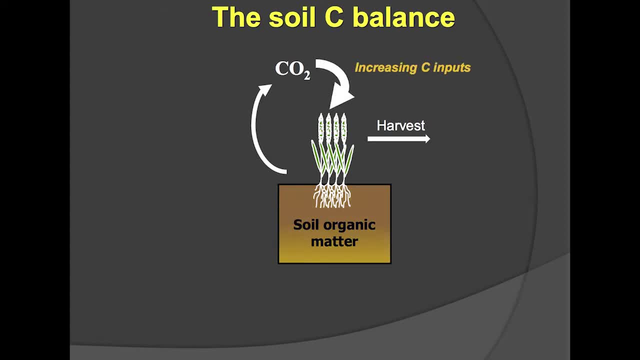 And the answer is fairly simple. On the one hand, we can increase carbon inputs, you know, fix more CO2, get more of that, That is, organic matter, into the soil, And we can try to reduce carbon losses through respiration and other sources. 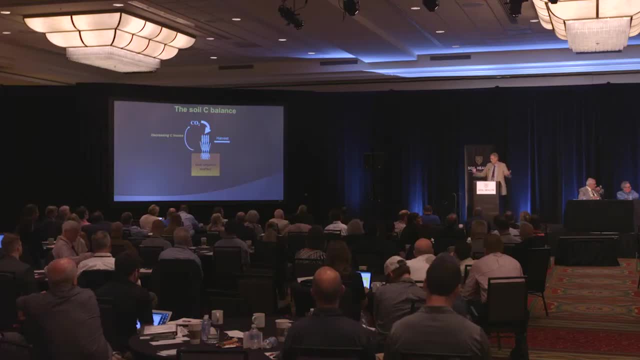 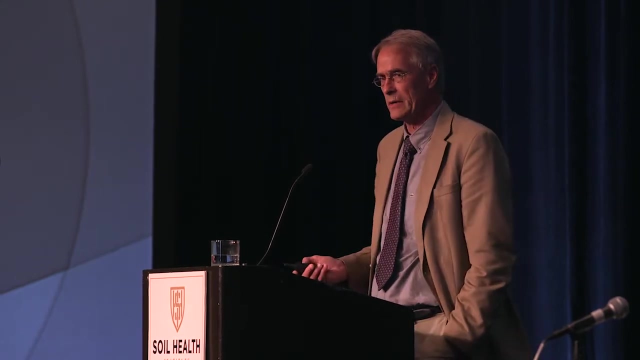 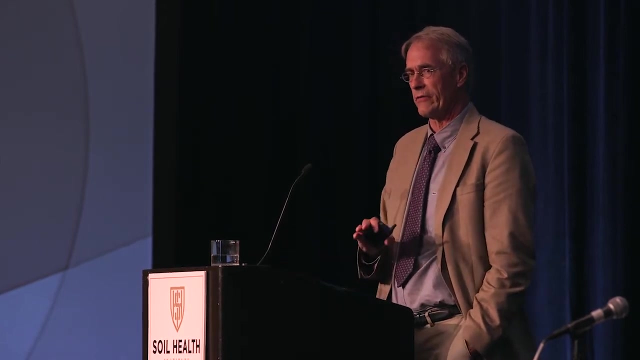 So, as we change that balance of inputs and outputs, that box that represents the soil, organic matter storage, that gets bigger, And if we can maintain that, then we're effectively removing carbon dioxide in the atmosphere. Okay, So some key principles. The first one is that the duration of carbon sequestration is finite. okay. 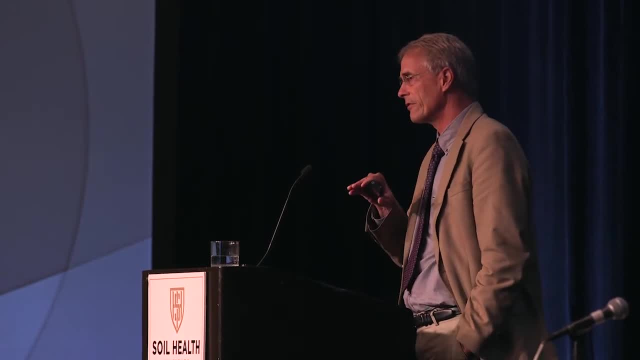 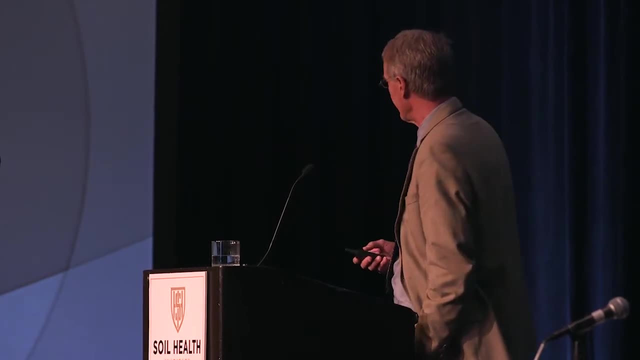 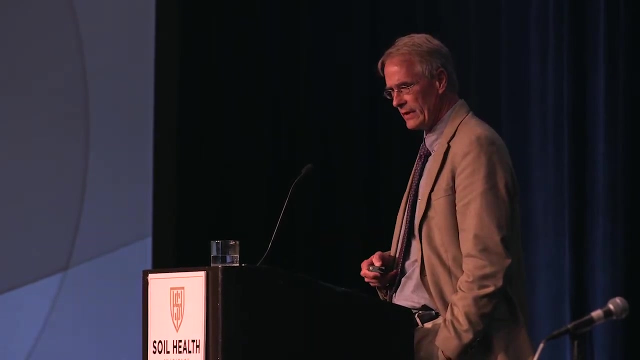 So as we change that soil carbon balance, the stock of carbon in the soil tends towards a new equilibrium, So we can have an effect over several years, but eventually that increase that we might have attenuates. The other point is that the total amount of storage is limited. 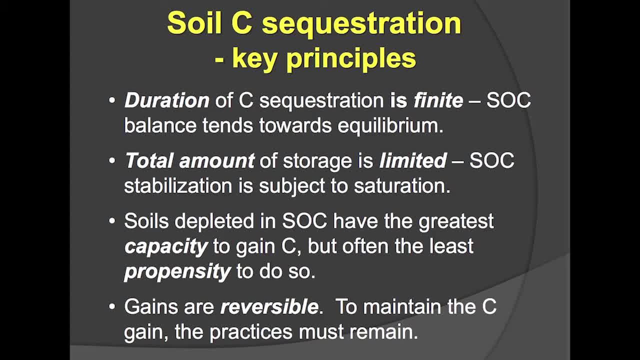 So we can't just add infinitum, Add more, Add more, Add more and more carbon. certainly, to most soils, to most mineral soils, we eventually receive, or get to a kind of a saturation limit, if you will. And the other point, another important point, is that soils that are relatively depleted in soil, organic carbon. 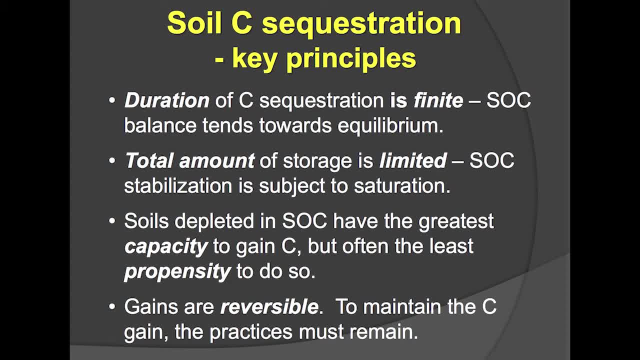 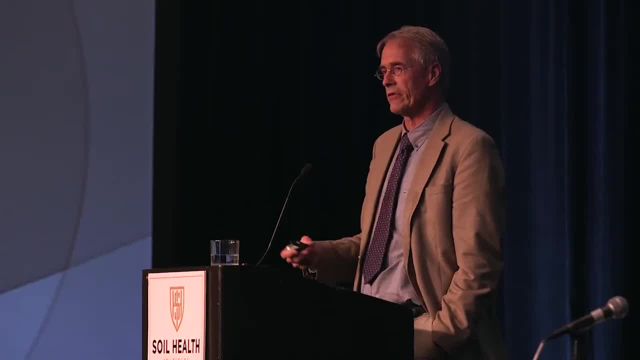 particularly from past land use, probably have the greatest capacity to gain soil, but often they have, they have the least propensity to do so. In other words, if you have a low carbon soil, it has the capacity to increase its carbon content significantly. 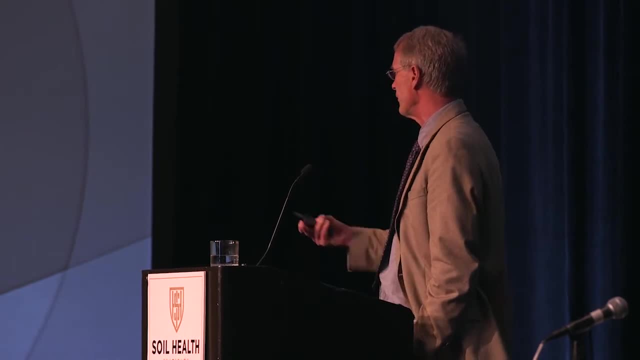 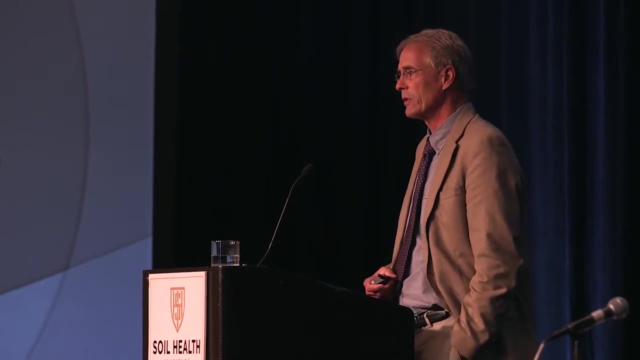 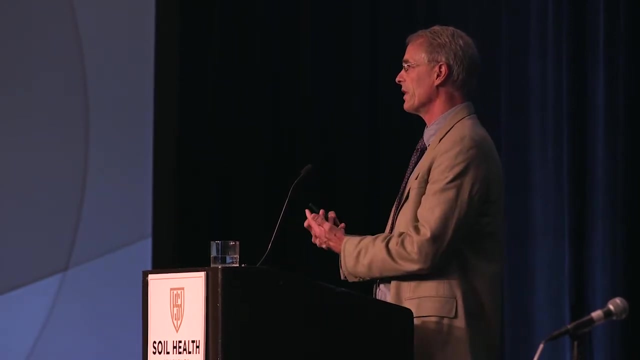 but because of feedbacks to soil fertility and other things, those soils may be the hardest to lift up. And then finally- and this is a really important point that I think everyone here probably gets- is that the gains are reversible. So we've got a soil carbon balance where, for the most part, we're not adding carbon into the soil. that's inert. 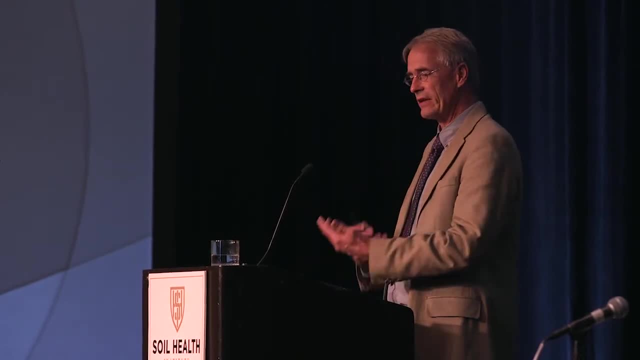 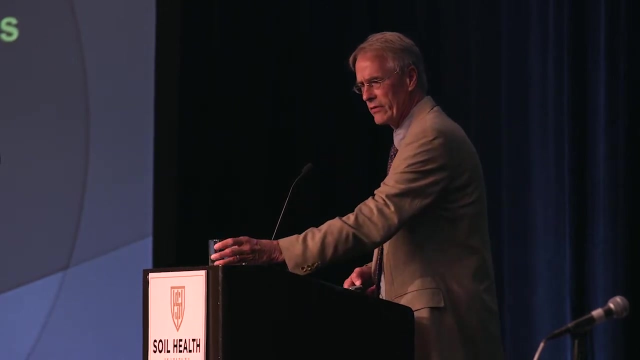 it goes in, it comes out again. so it's maintaining this, this carbon balance, that we're trying to do. So if we're going to implement practices to to increase those stocks, we have to maintain those practices over time. Okay, just want to quickly go through sort of some of the conventional technologies, if you will. 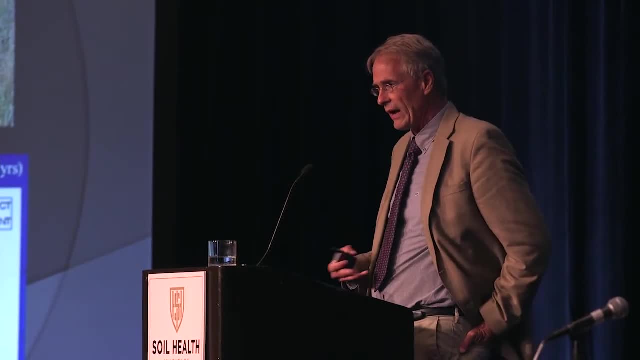 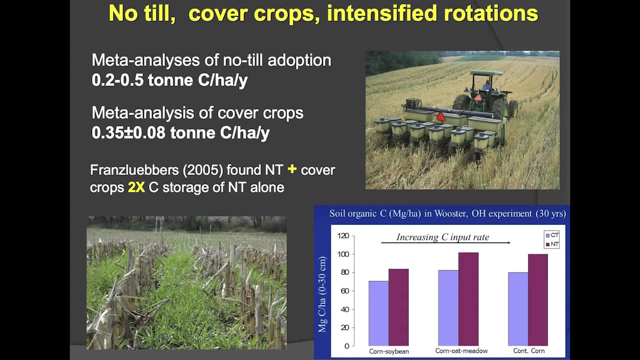 These are things all of us you know know about. So how do we manage our annual cropping systems? Things like no-till cover crops intensification Can? will we even find these resources that allow us to finish cropping through those tweaked processes? Like, how could we modify them? How could we make a bet with other, different technologies that aren't those you have to make an estimate of to get to any of those lower levels? and then, how would you consider these resources that you've found, these resources that are extremely non-essential? 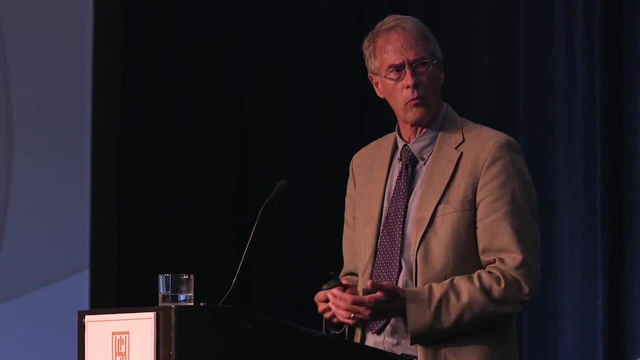 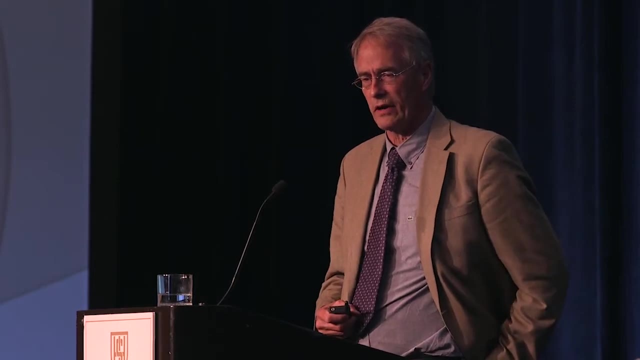 can gain carbon. not every soil is going to do it but, on on the whole, most do cover crops. again, you know fairly reasonable numbers of, of. you know a third of a ton of of carbon per hectare per year. i think one of the interesting uh things too is the synergy between these different things. you 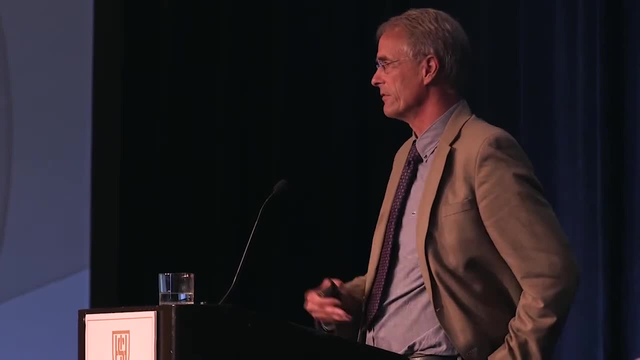 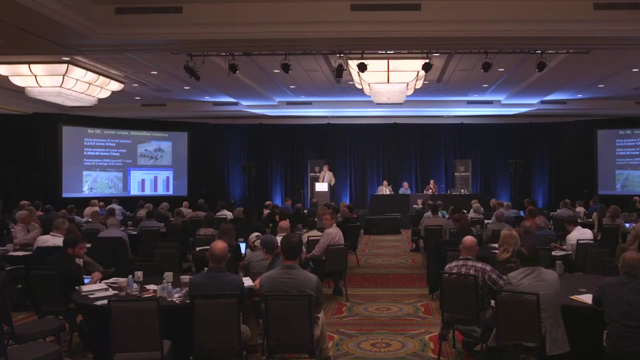 know if we, if we, combine no-till with cover crops. alan franz louver had a paper a number of years ago and he showed some really nice results about that kind of a of a synergism, and then you know. another example is: is data from the, the wooster long-term sites that, looking at at conventional 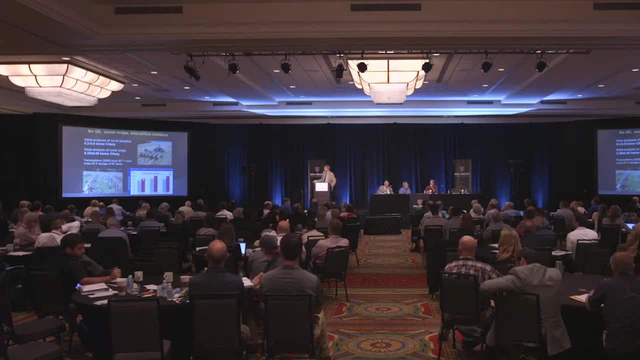 till and blue and no-till here. you see, yeah, okay, different rotations, uh, no-till is- is showing higher carbon storage. but you also see a, you know, an interactive effect: as you increase the carbon input rates in terms of more residues coming into the system, then, you know, the total increases as. 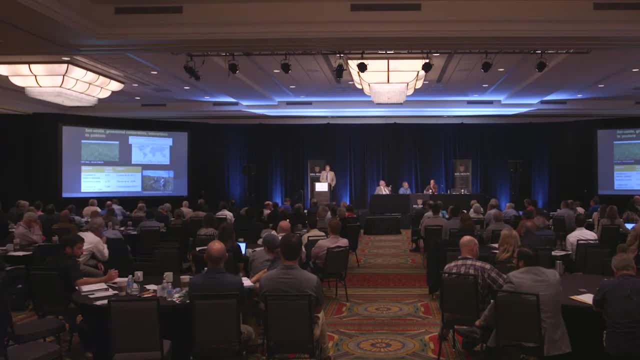 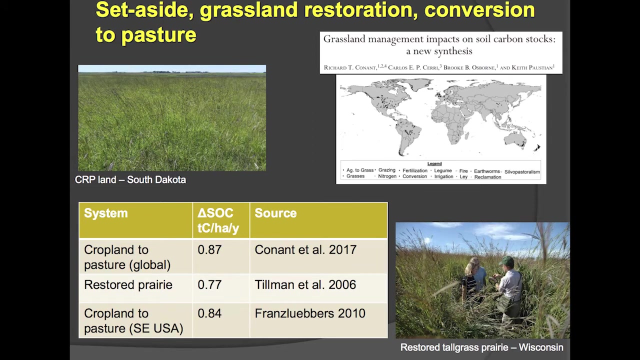 well, um, so if we, if we take, uh, marginal lands, uh, or or lands that are maybe not well suited for annual cropping, and we put those back into, say, grasslands, set asides- you know, we know really well how this works right- and and we convert back to perennial grasses, you have a lot of carbon input through the. 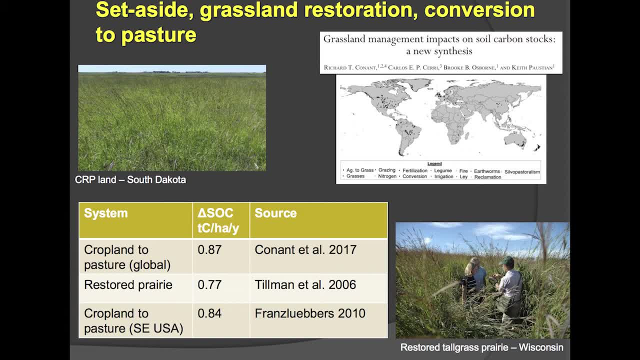 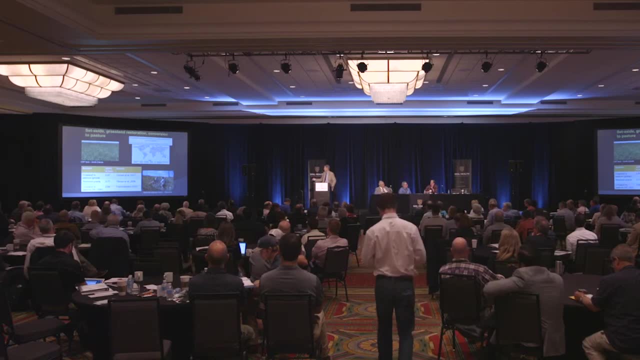 roots, you have the absence of of tillage, you have a a long-term, permanent uh vegetation cover there and and so those kind of systems you know show really quite high. you can get up to a ton of carbon or more per hectare per year. again, these are averages from a number 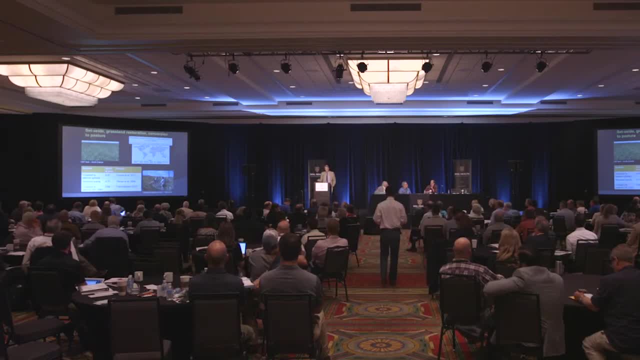 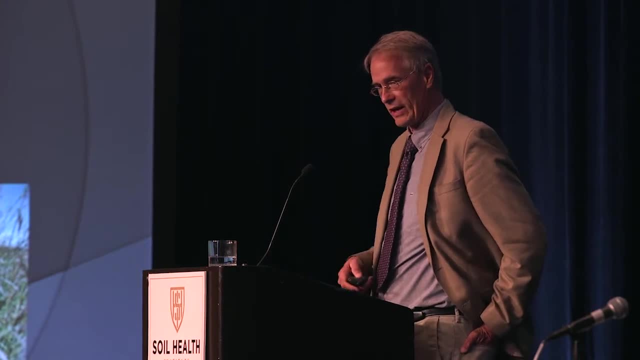 of meta-analyses, but it's a very effective strategy for for increasing soil carbon right, but of course you can't do it everywhere. uh, we've got to have annual crops to maintain our food systems, but you know, so we understand. anyway, this is a an opportunity. 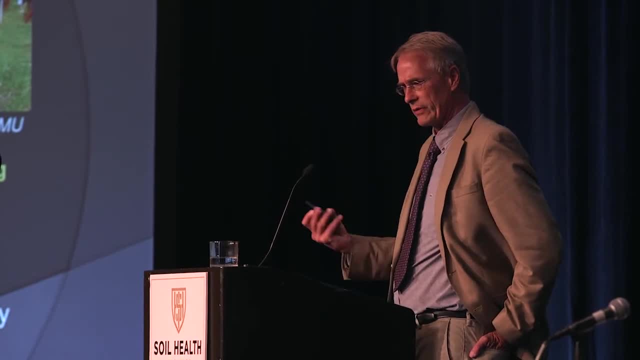 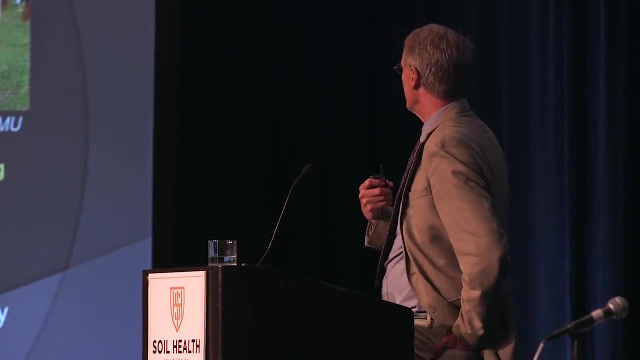 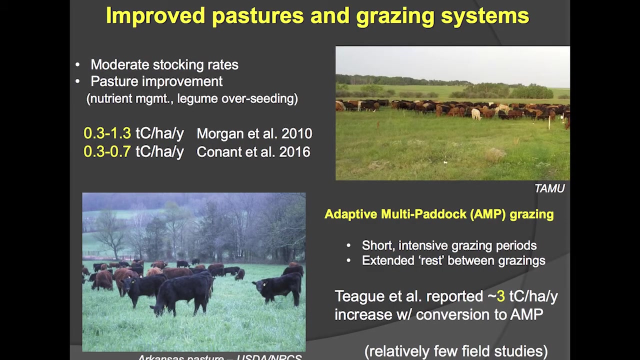 um, and if we look at our, our, our pasture and grazing systems, you know, again, there, to the extent that we can increase productivity, we can improve the, the health and of of the of the pastures through different kinds of- uh, you know, better stocking rates or pasture improvements. 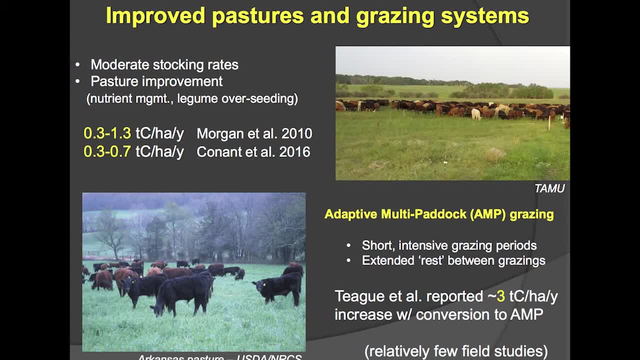 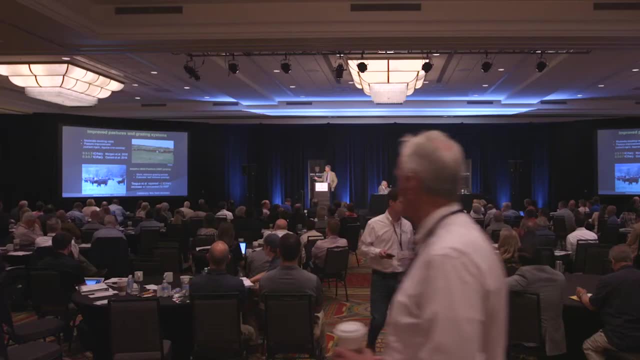 things like this: uh, you know, fairly modest but but significant uh soil carbon uh increases. there's a lot of interest now too, and and some other issues and some kind of potential. um, there's an um a large controversy, i guess, for things looking at things like uh, adaptive multi-paddock grazing, rotational grazing. 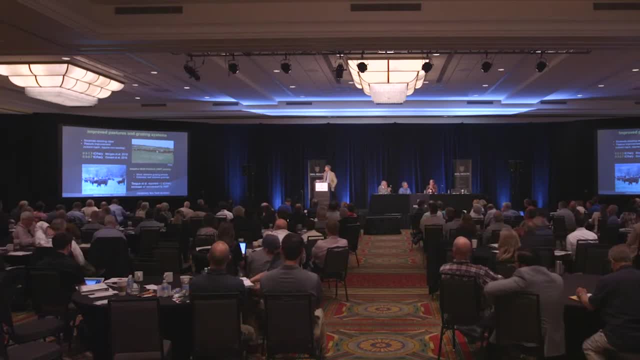 other things where you know we we change a lot the way in which, uh, we, the livestock, utilize the land and there's certainly some suggestions that those kind of systems in some cases can really lead to quite substantial uh increases in soil carbon. but there you know, we really need some. 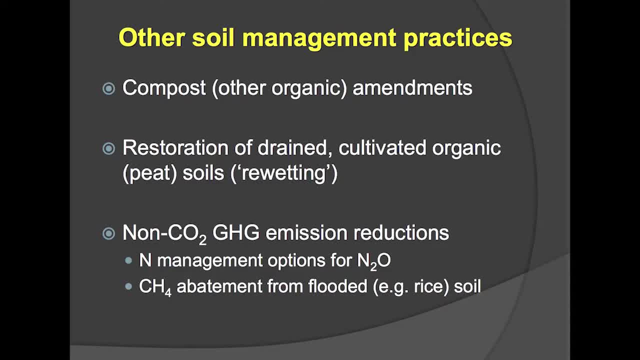 more field studies there and there's other other soil management practices. uh, you know, i'll talk a bit about them in a second. but uh, you know organic amendments and and and particularly looking at organic soils and and how we treat those, and of course i'm not really going to talk about. 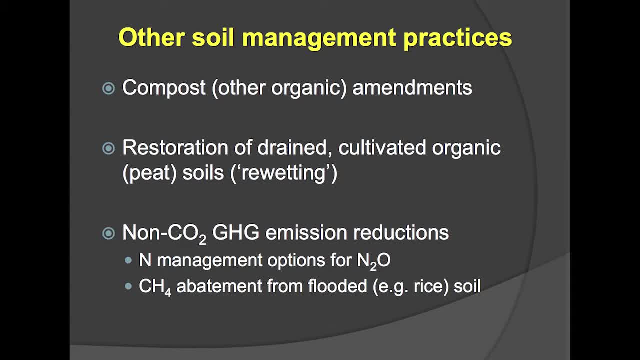 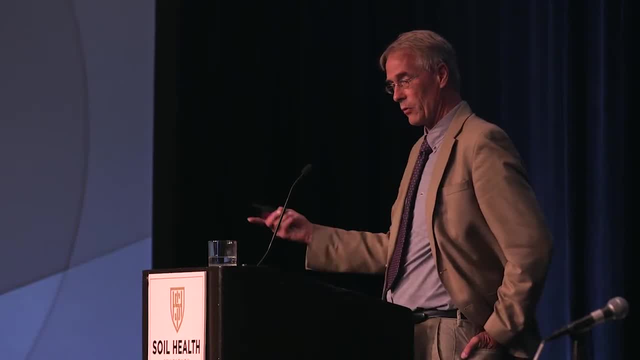 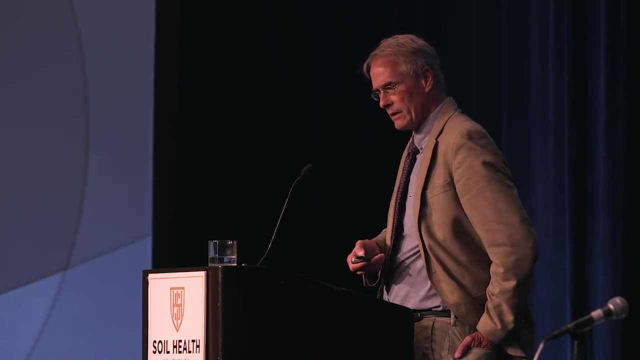 non-co2 greenhouse gas emission reductions. but that's a really important point for, you know, agricultural soils in particular, where the the really the biggest contribution of global warming or greenhouse gas emissions is really for these non-co2 uh emissions. okay, so, so that's kind of 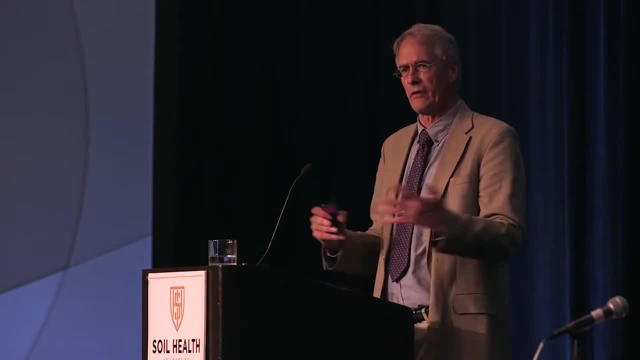 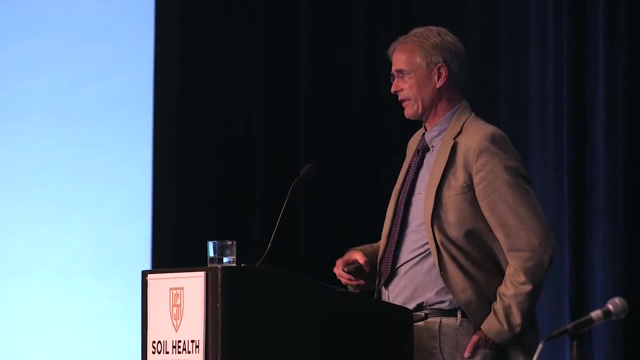 like the things that we know well and we've got, you know, quite a few studies and we can quantify that pretty well. and then there's what i would call frontier technologies, so things like, and there's interest in things like biochar, addition to soil. so what is biochar? so, probably most people. 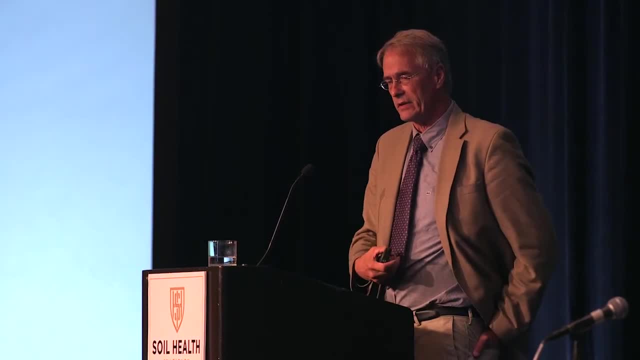 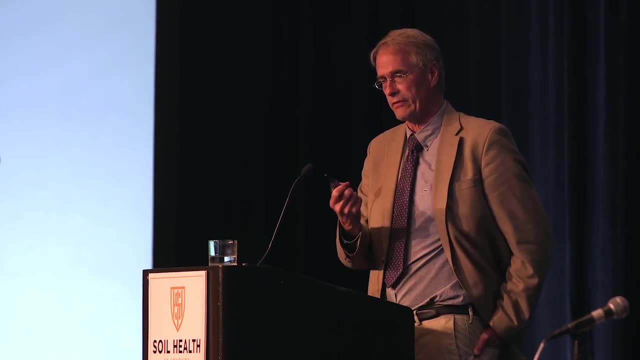 here know, it's a co-product of, of a you know, a pyrolysis pro process that could be used for bio fuel. it's a, you know, produces this, this charcoal, which is, uh, high porosity. it's. it's quite miserable. it's a high porosity, it's, it's quite miserable, it's a high porosity, it's, it's quite. 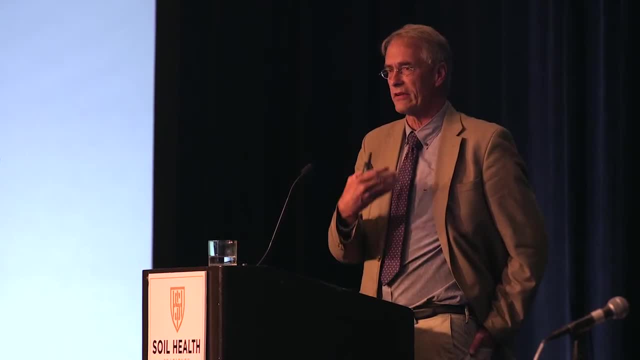 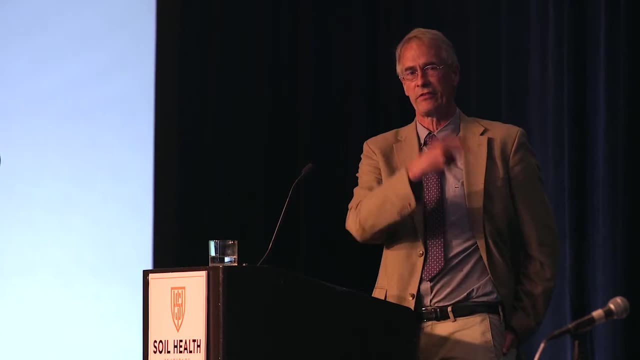 resistant to decomposition? it can be and it can persist in the soils for for a long period of time. so it's a little bit the exception to the rule. if you add lots of biochar it doesn't necessarily come out again very quickly and it in some soils. it increases plant growth. it also 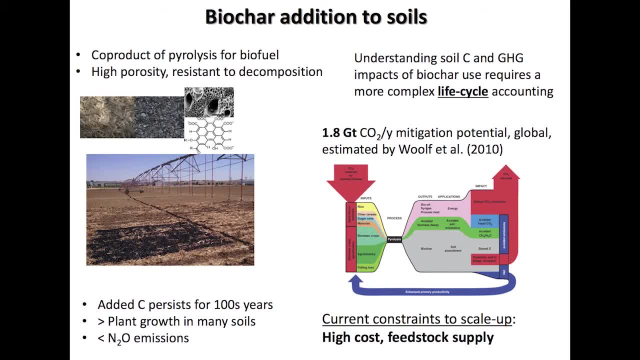 seems like it often uh reduces, uh nitrous oxide emissions. so there's a lot of interest in biochar. it's it's still, i think not, it's something that's kind of out there, um, and you know, we don't know exactly what's role it's going to play, uh, and one of the things in particular about 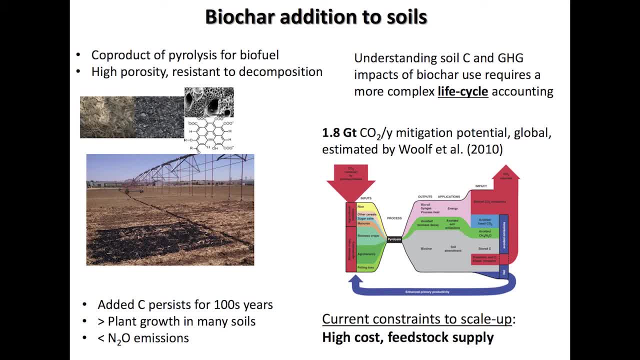 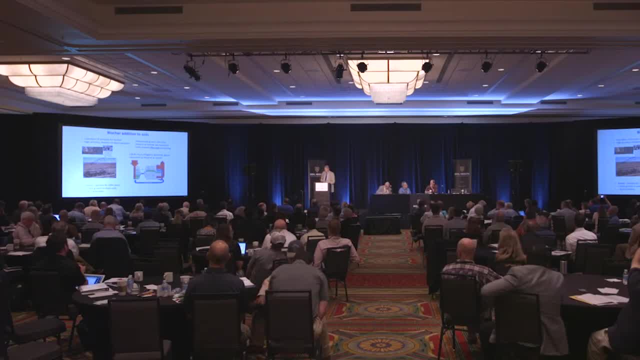 biochar though is, is that it's, uh, because we're looking at at bringing in feed stocks from elsewhere and there's there's the process of making it and adding it and transporting it. so to really understand the the net greenhouse gas impacts of practices like this, you really it's a. 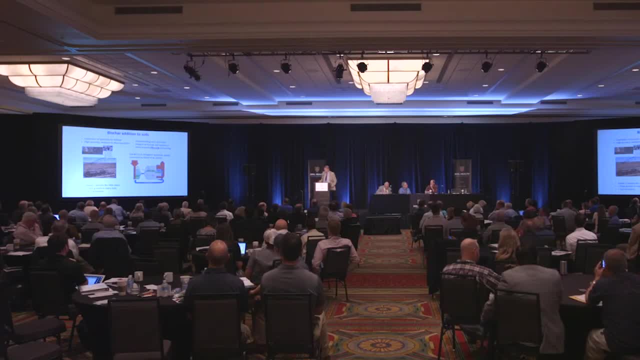 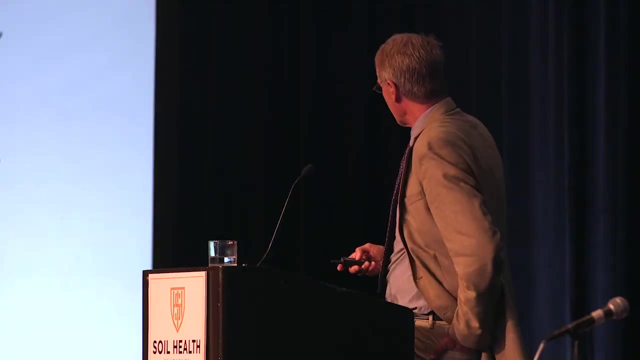 bit more complicated, i guess, and you need really a more of a, of a, you know, a life cycle assessment approach. uh, and, and you know, right now, i think that there's the biggest constraints to maybe scaling that up- aside from, you know, knowing a little bit more about how, how it performs in different soils- is 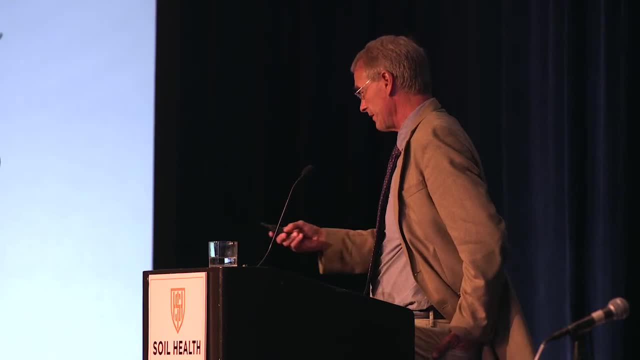 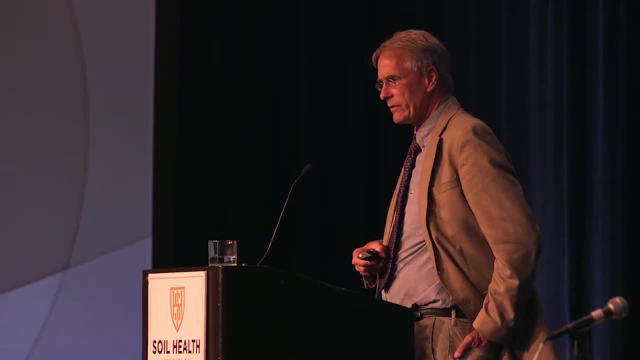 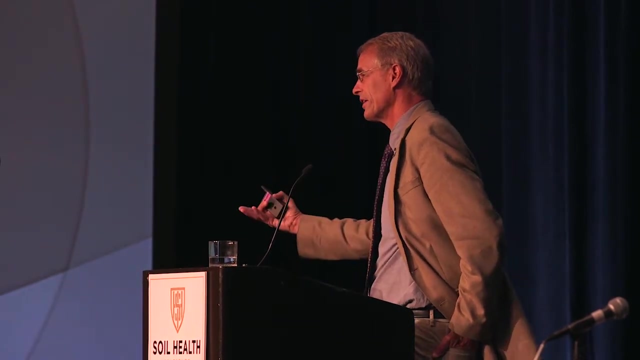 really, right now, i would say, the high cost and and you know where's the feedstock going to come from. but it's something that that i think there's a lot of interest in. another area is is, you know, looking at our crops. so so the crops we're growing have certain 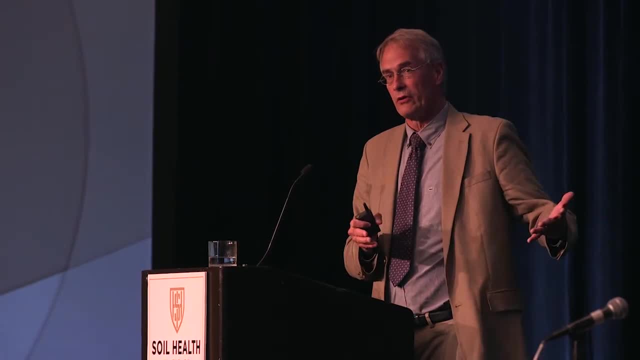 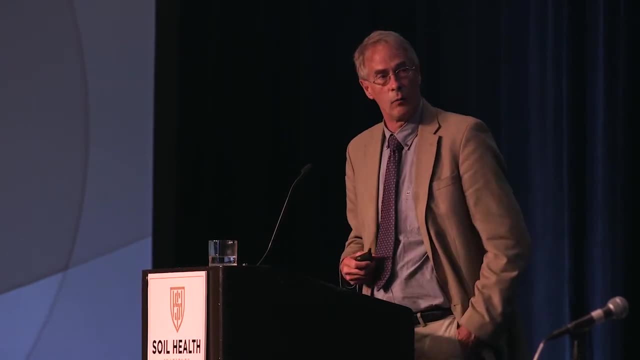 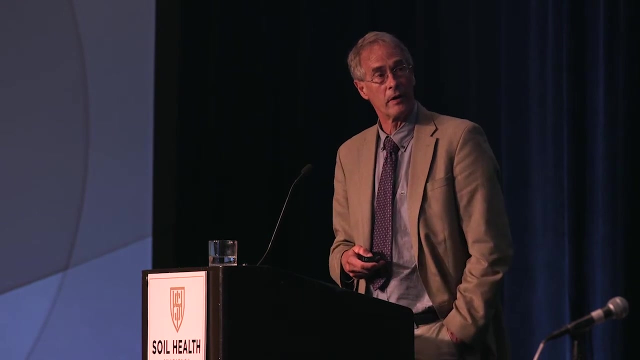 things that they're going to need to grow, and so what if we change those things? so, for example, what if we start trying to use annuals that have more and more more roots and deeper roots? uh, we did a kind of a quick and dirty analysis for arpa e here last year, for their, uh, their, their. 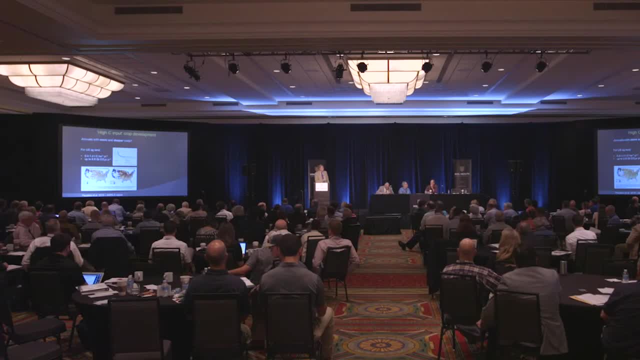 program that they're initiating, uh and and kind of did an assessment for for us ag lands and and really there's a potentially, if we're able to have these crops, that we're going to be able to grow, and we're going to be able to grow these kind of crops. there's a really a large amount of of soil. 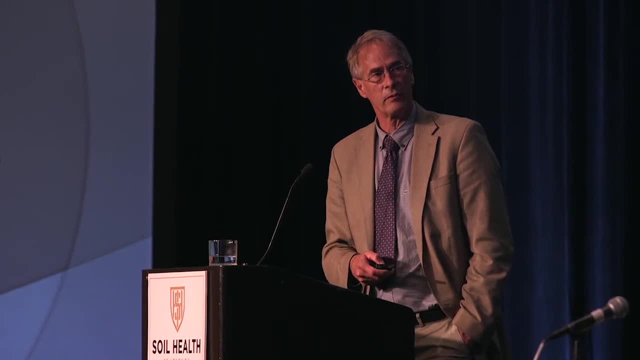 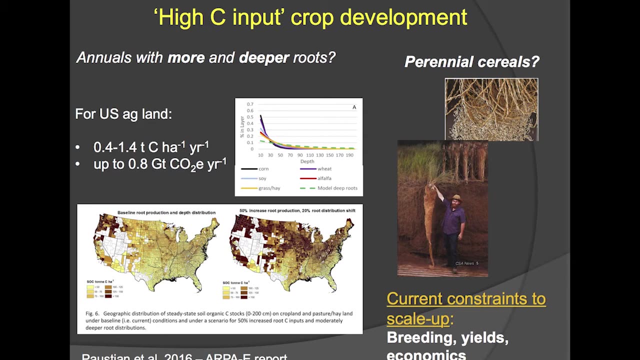 carbon that potentially could be, uh, stored and increased with. with this kind of an approach, another one could be kind of going the other way. we've got perennial plants. can we, you know, can we develop perennial cereals? and, of course, the folks that a lot of people know the work at the land. 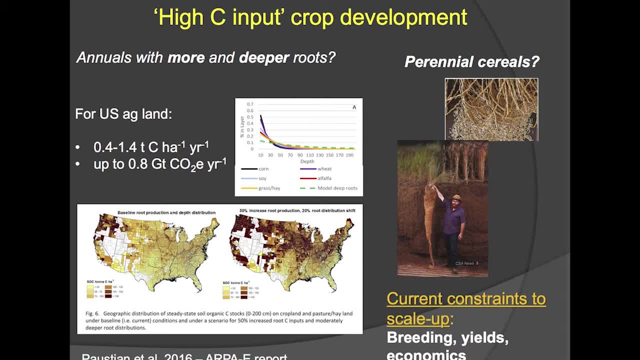 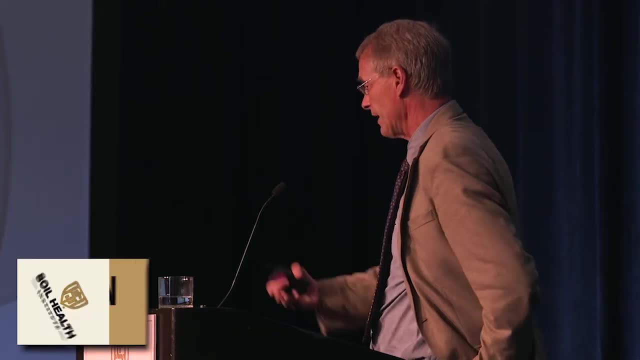 institute and other places are a lot of interest now in in doing this and and uh, and, obviously, if crop plants that look like that, uh, that are also producing grain, uh, it's, it's a, it's a potential game changer, but there's, you know, constraints. we're not ready to scale that up now. there's. 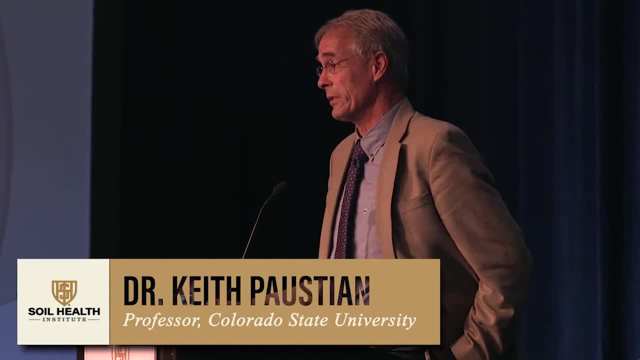 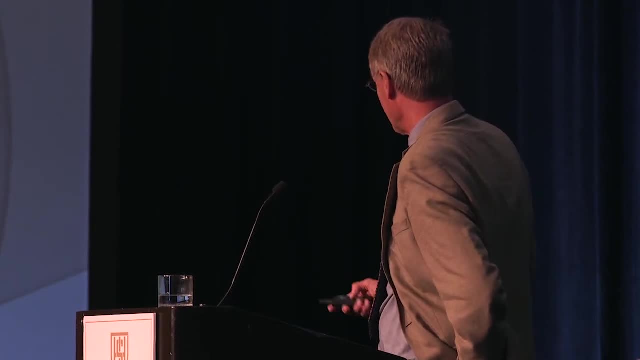 yeah, there's uh. actually last week i had uh kern's a beer and and kern's a uh salad and uh, but it's, it's not really quite ready for in terms of the yields and the economics to to plant across the midwest, but again, potentially, you know, think about. 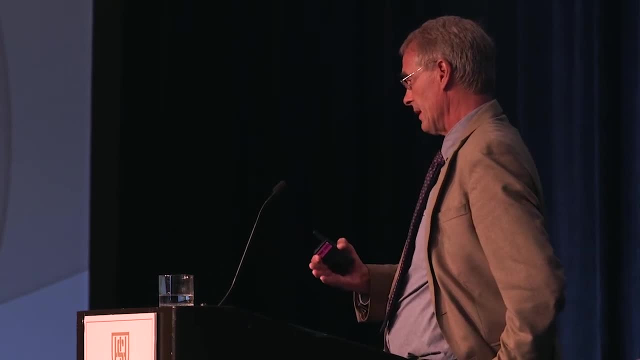 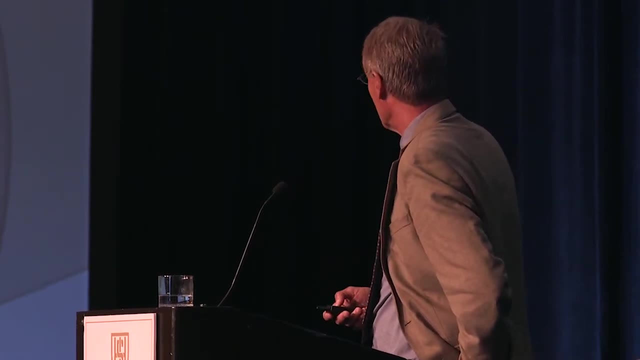 what i said before about perennial systems and grasses, uh, and the carbon sequestration potential that they have. so so this could be potentially be a big deal, but it's, it's down the road. so then kind of get into the final question is: is really what's this aggregate potential then? 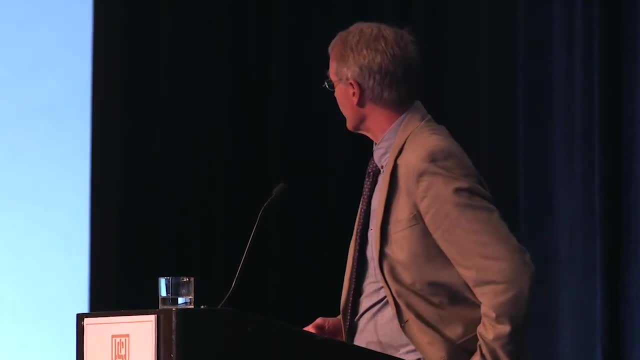 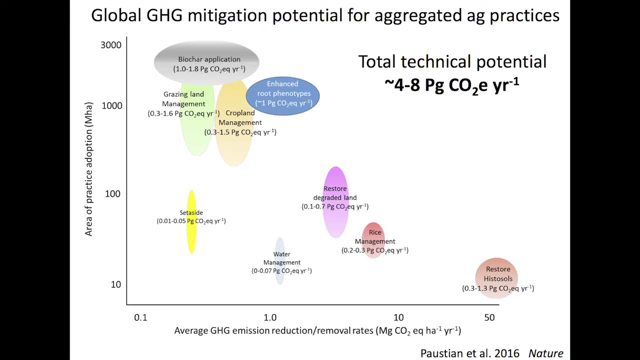 and a year ago. so we had a paper in nature that that got quite a bit of attention and and this is is is kind of a of a summary graph from that, and i guess i'd want to point out a couple of things here. on the one hand, it's like if you look at the x-axis, here you've got. 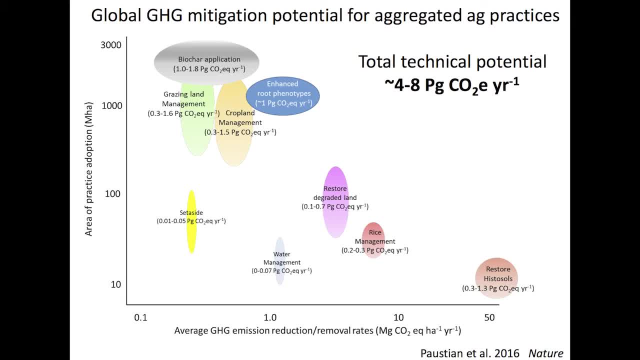 this is the rate of carbon removals or co2 uptake in in storage per hectare per year. so it's again, it's a log scale here, going from, you know, 0.1 ton of co2 equivalent per hectare per year to to up to 50 and over. here on the y-axis you've got the area that the practices. 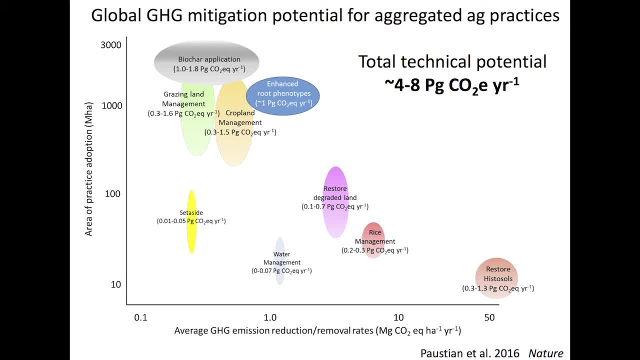 were adopted in, and so you see a couple things from this. this figure one is that that there's a lot of there's a lot of different things that you can do a lot of different things that we can manage the soil to increase the carbon storage, but they're all a little bit different and they 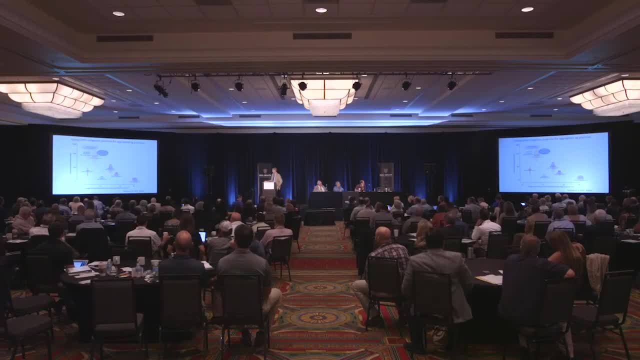 kind of array themselves in this way that there are some practices, such as restoring peach soils and re-wetting cultivated organic soils that have a very high rate per hectare of carbon removals, but there's not really that much land that we can apply that at, whereas over here 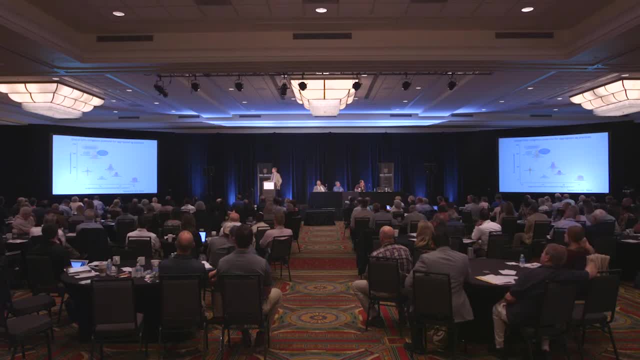 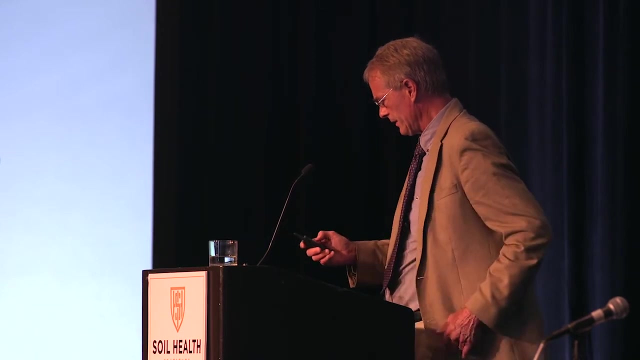 you know you've got fairly modest per Hector emission reductions or or carbon uptake, but there are a lot of land area that they can be applied to, so you know you can. so those are really the, the two kind of of components of this uh and- and we came up with this- this uh estimate of anywhere. 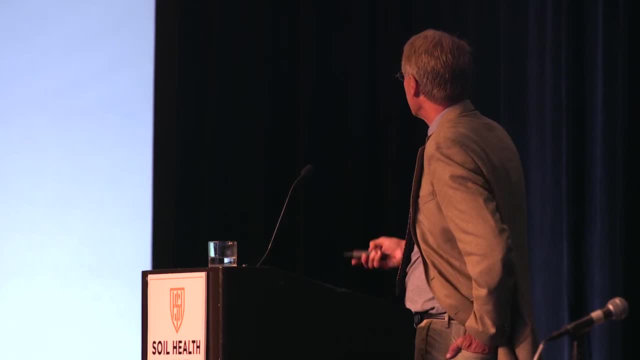 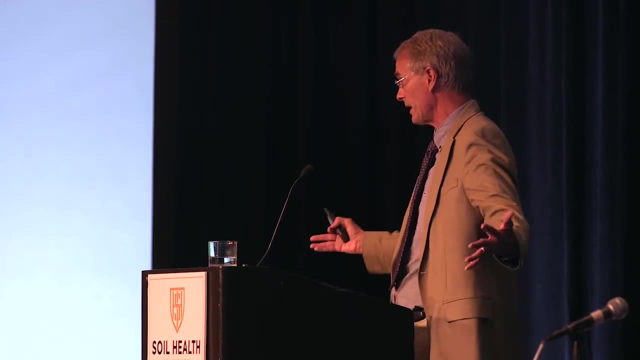 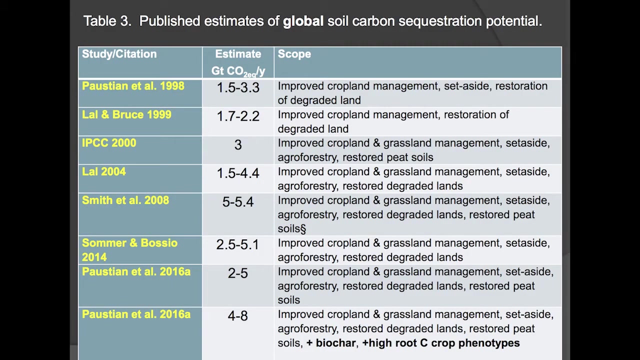 between eight to two or four to eight uh billion tons petagrams, the same as gigatons of carbon dioxide equivalents per year, if there was really wide adoption of these different practices. okay, and so that this wasn't the first, by any means, uh estimate, and and we've got some, some. 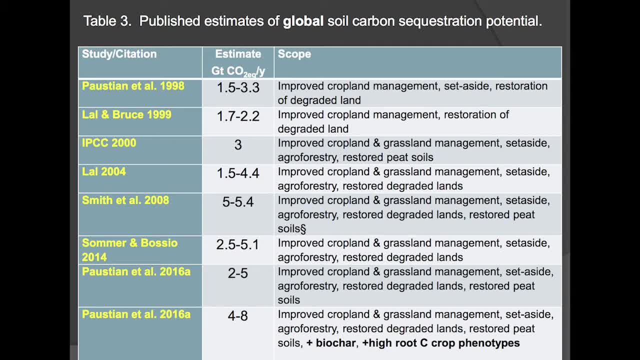 uh, some other ones here and I won't have a whole lot of time there to to discuss these, but and and they look like the, the numbers are sort of you know, across the board, but actually if, if you, you know, if you, if you look at it, there's 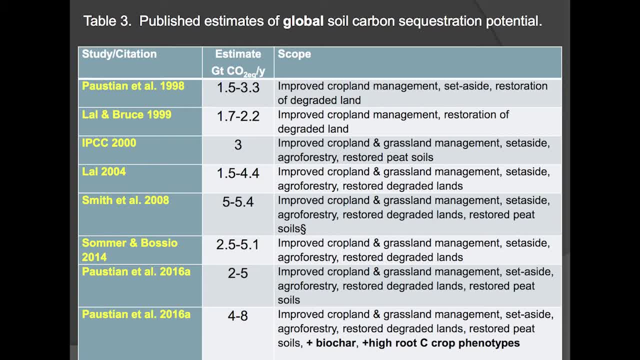 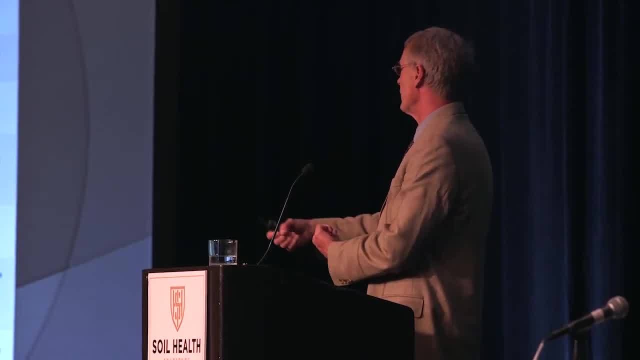 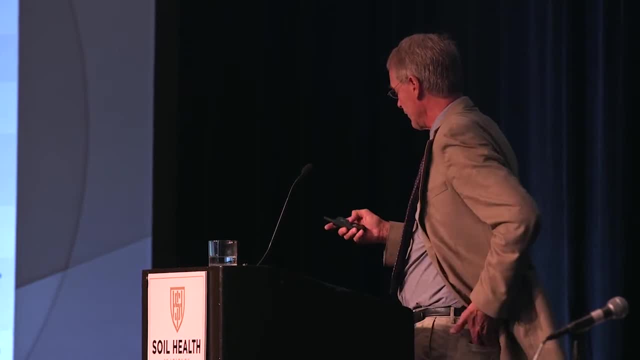 a fair amount of consistency really. that suggests that, gee, our estimates say, you know, somewhere on the order of three to five billion tons per Hector per year for some period of time- would be achievable as a technical potential. and then if we add some of these Frontier Technologies, it could. 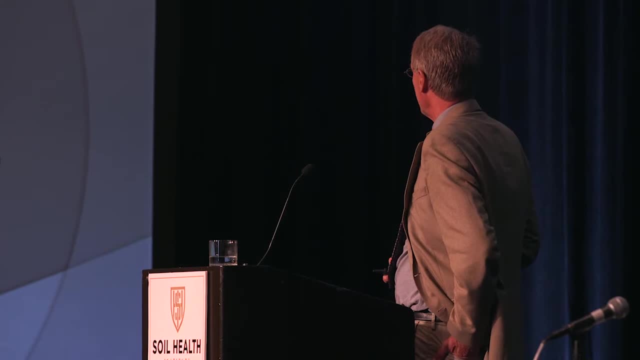 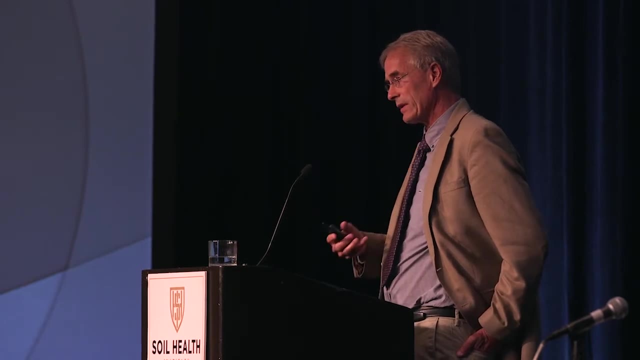 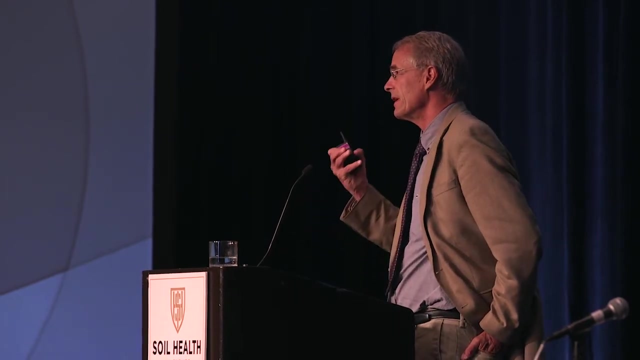 be, even be higher. so I think that's the a little bit. the bottom line is that, uh, you know, we have probably a pretty good idea of what the, the actual technical potential is. uh, and it's enough, it's enough that that we can say that soil carbon sequestration can play a. 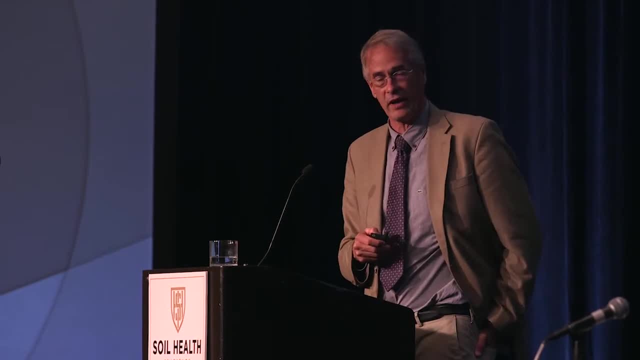 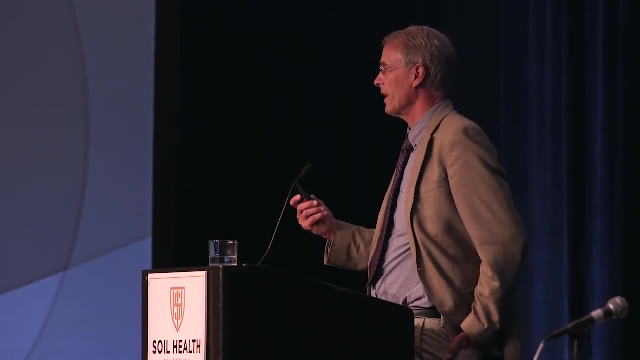 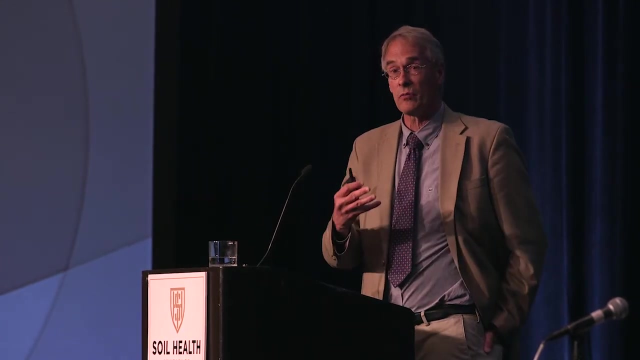 major role in this, uh, global greenhouse gas mitigation story. uh, and, and I would even say that this technical potential is is pretty well characterized. we don't, you know, we have a pretty good idea of what it is, but the biggest unknown is: what's the adoption rate? how? 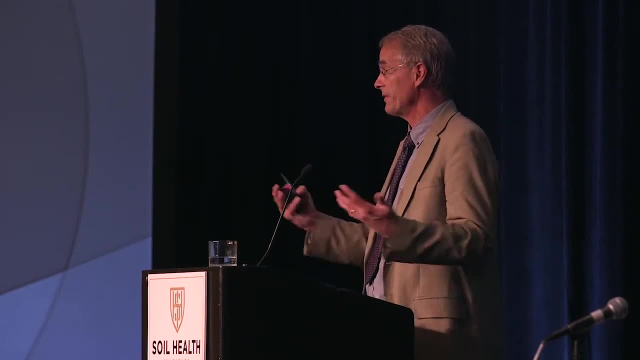 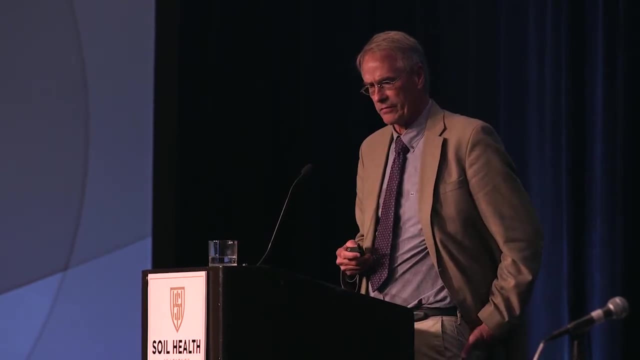 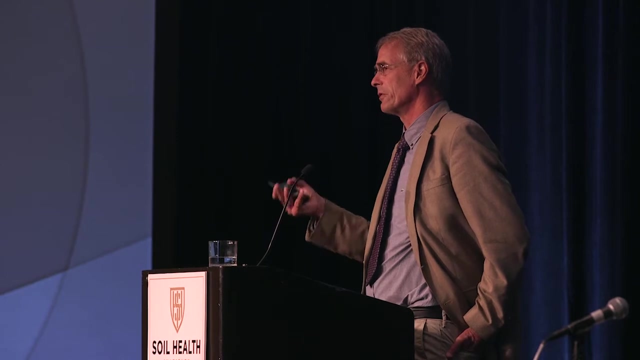 are. you know how much land can we really get to adopt these kind of practices? because that's really where it's going to to add up, uh, you know, to the final story. and and in order to do that, we've really got to understand how do we incentivize producers, farmers and ranchers to 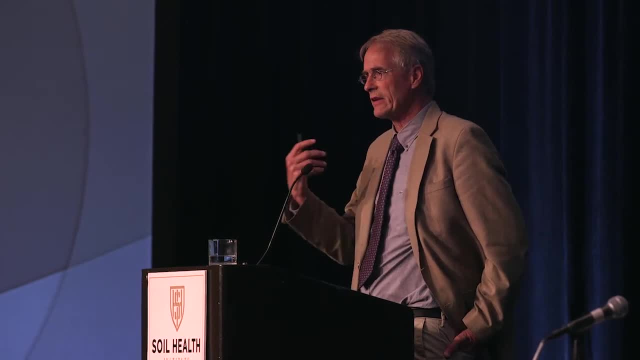 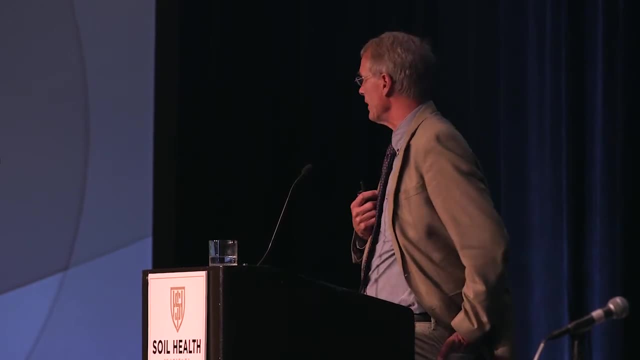 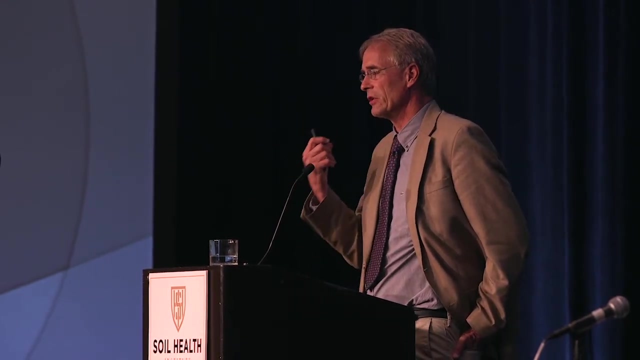 adopt these practices, the things that Wayne was talking about, and I think as as going forward, what we'd like to do is- or what we need to do, I think is to- is to really implement a kind of a two-stage strategy, and that is. there's things that we know now. we have a suite of best management practices. 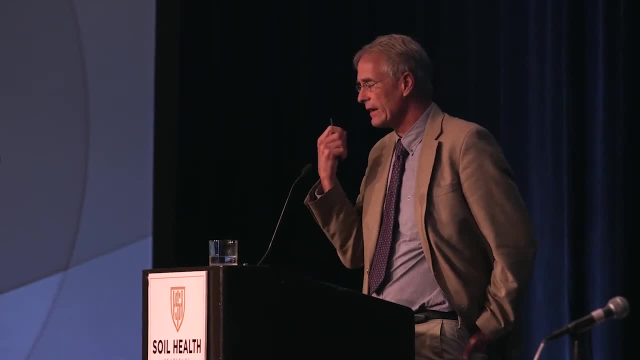 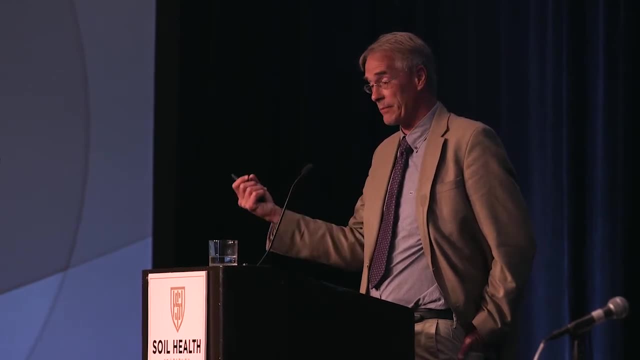 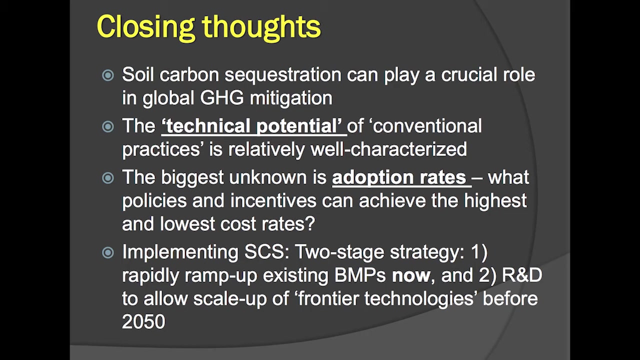 that we know work that sequester carbon in the soil and how. you know that that is really just an issue of policy and and and economics and incentives to ramp that up. and we've got some other things that might be game breakers. they may be, you know, perennial grains, or or. 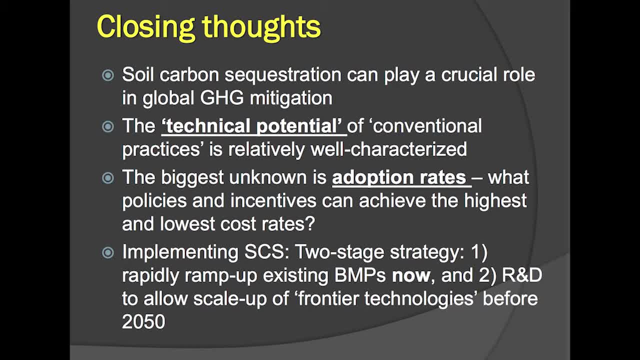 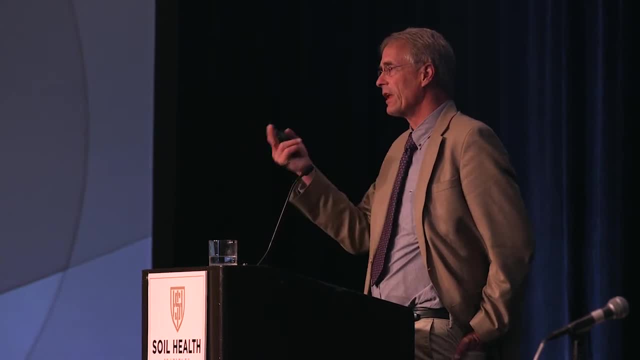 annuals with deep root systems or biochar or other kinds of amendments, or or you know many other things that I haven't talked about. we need to continue the r? d to allow this potential scale up of those Technologies because, according to the- you know the estimates I showed in that first- 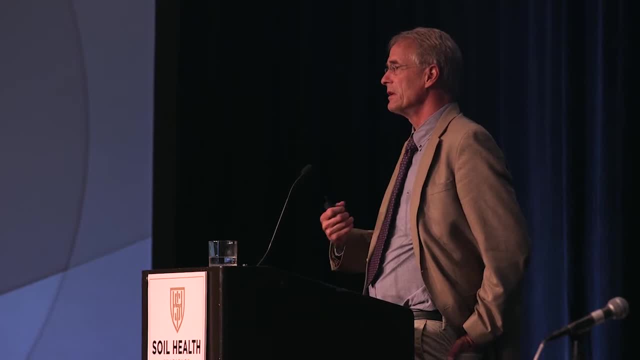 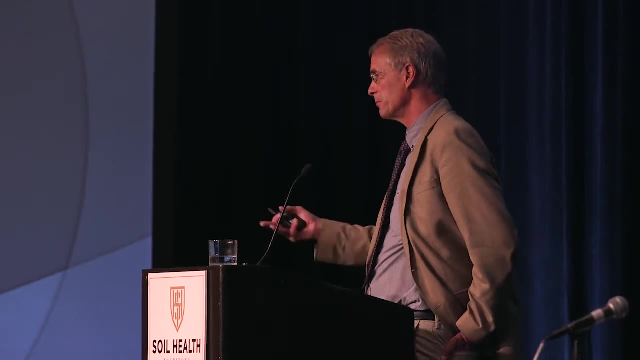 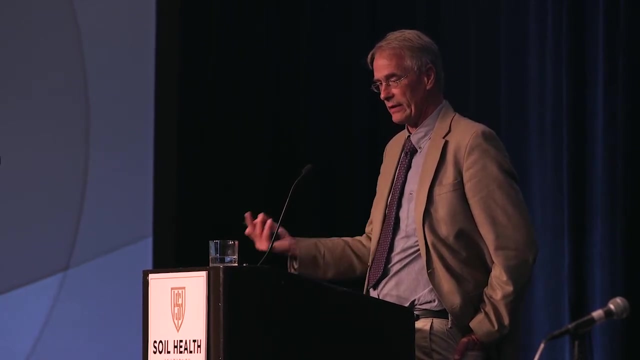 slide. we're going to need somewhere on the order of 15 billion tons of CO2 equivalents, of carbon removal by some mechanism, you know, before the end of the century, to to stay on this desired pathway of greenhouse gas reductions, and it certainly looks like so. uh, soils have a crucial 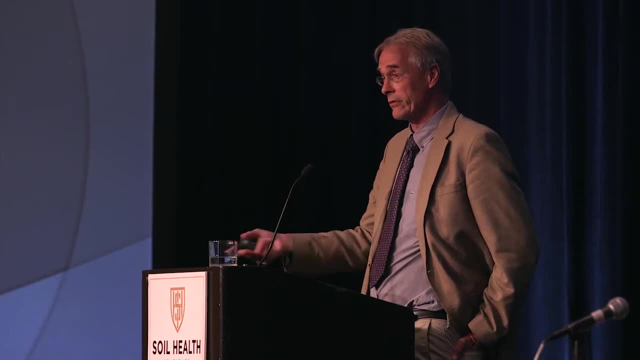 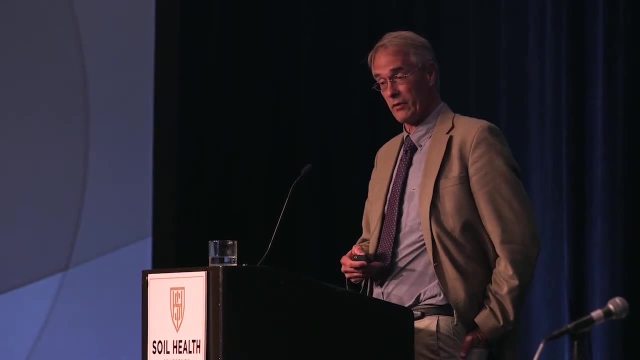 role to play there and we really need to. you know the work of the Institute and and others here in this room can can contribute a great deal to that. so I think I'm done. I'm a little bit over time, but not too bad, all right, thanks. 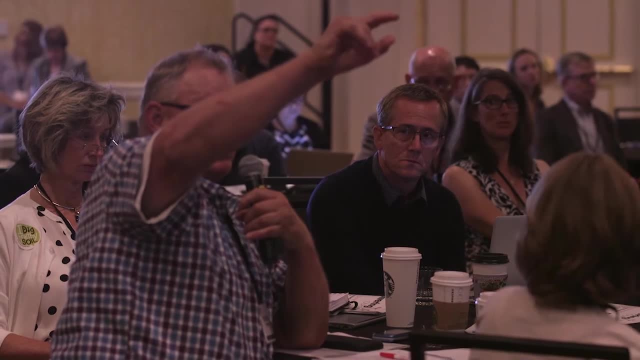 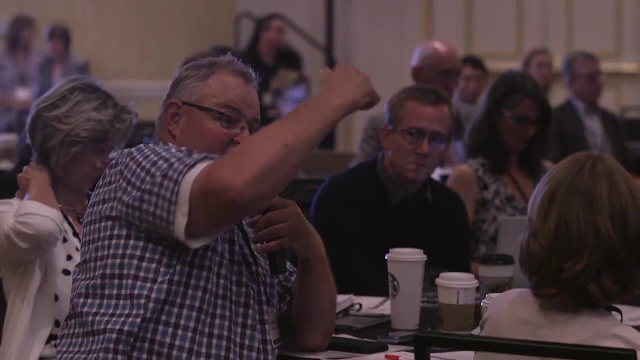 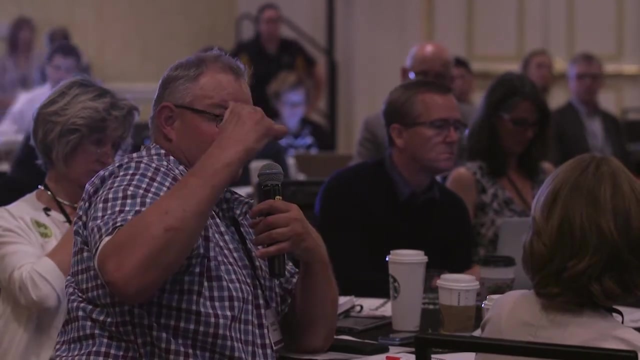 talking about the carbon sequestration and pulling that back into the soil and building that. is there a balance between a respiration sequestration- because you can have a net loss from two respiration, when you think of soil health and one of the metrics being soil respiration- and 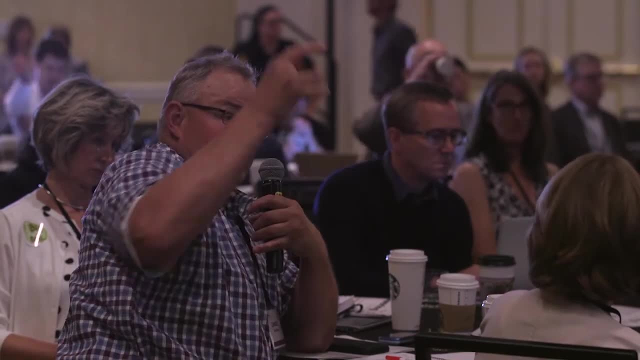 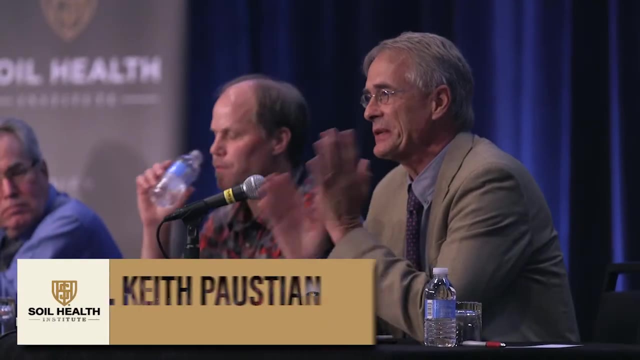 having a very high rate. good carbon cycling, nutrient mineralization. is there too much respiration? it's going to be too much and I think Henry Jansen, a really good uh paper. a few years ago we talked about this conundrum of you know: do we, do we hoard it or do? 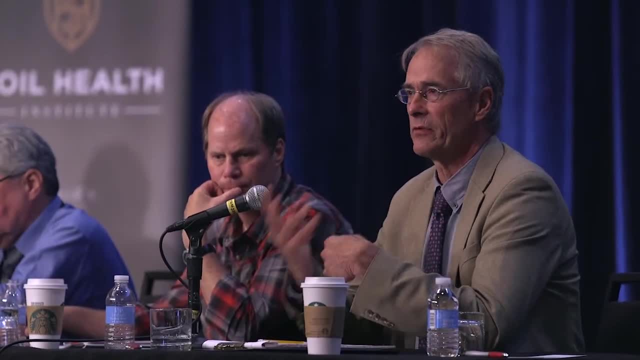 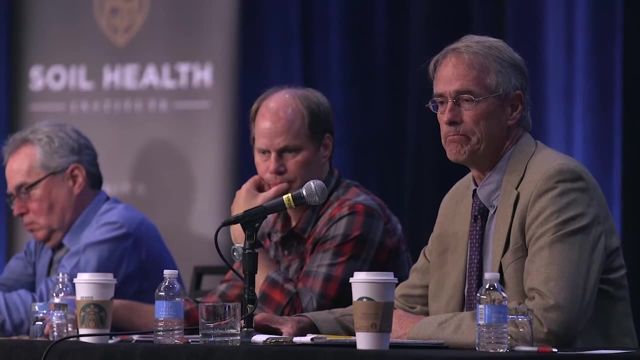 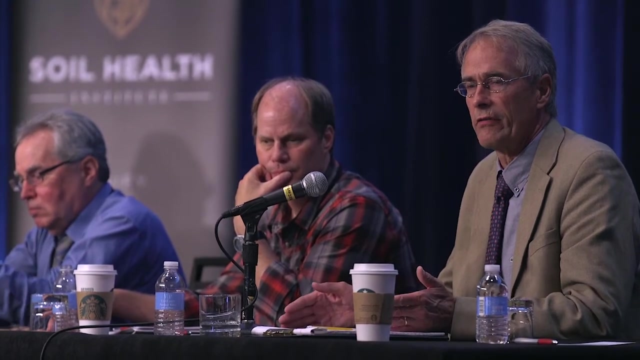 we use it because as we, as we metabolize that organic matter, that we're in crop residues and things like this, this is what fuels the- uh, you know, the soil biota and I- I guess I would say that you know we're the increasing your soil carbon stocks is is a transient kind of a behavior. 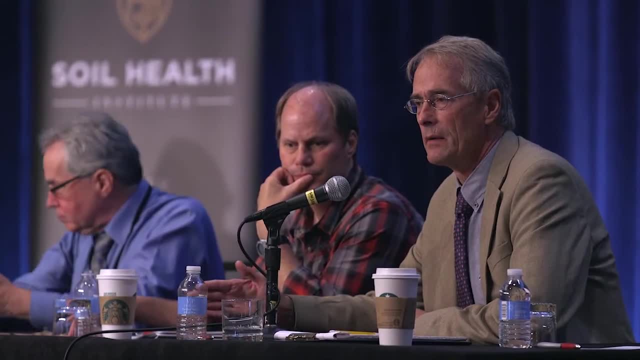 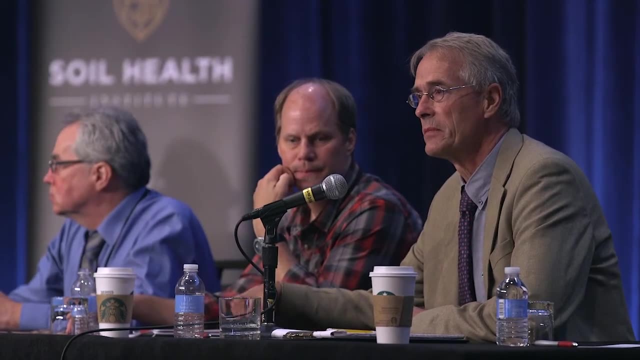 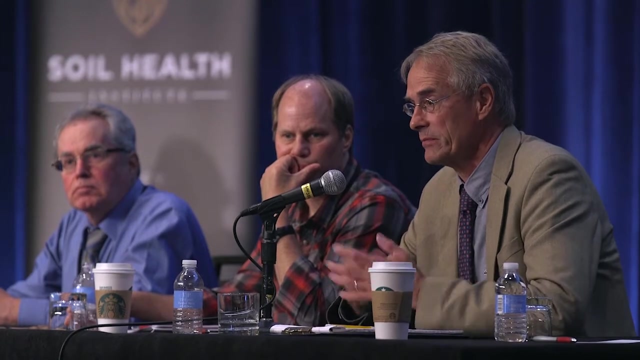 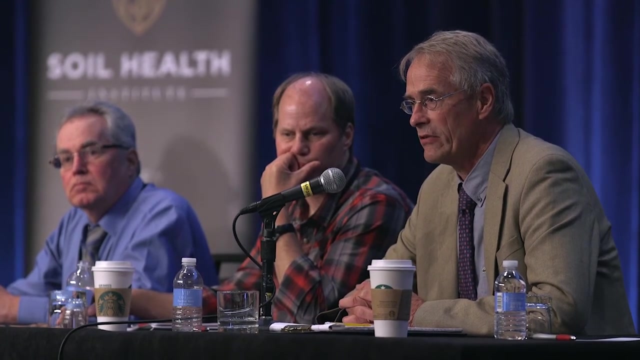 that that happens over some period of time, um, and then it's going to again reach that new equilibrium. at that new equilibrium, you know you, you, you want to attain a, a, you know a high level of of a biological activity. you want to have that, that soil functioning. you know, I, I guess, I think, you, you, 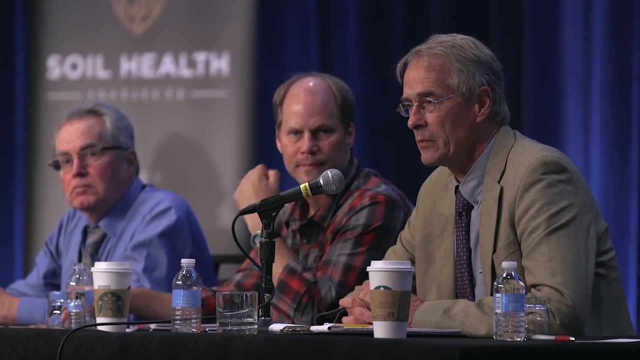 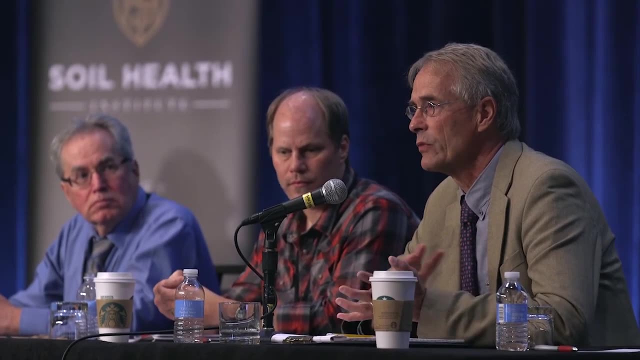 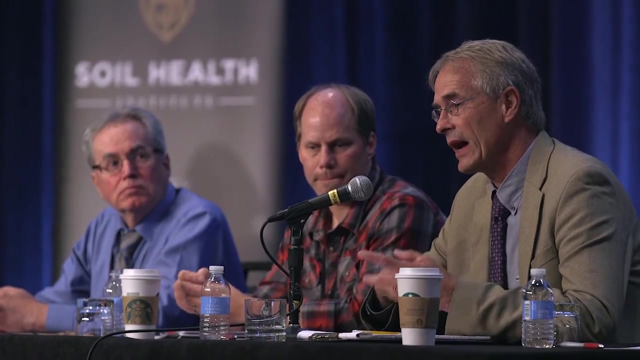 sort of do both. you know, I think you can increase uh carbon inputs and and you can do things like uh, like, for example, uh tillage, the. the way in which we think reducing tillage intensity increases, so carbon stocks is not on the carbon input side, but it's rather, you know, not breaking up aggregates and and not disturbing the. 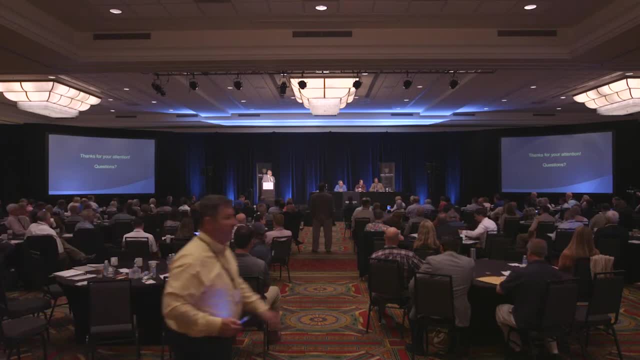 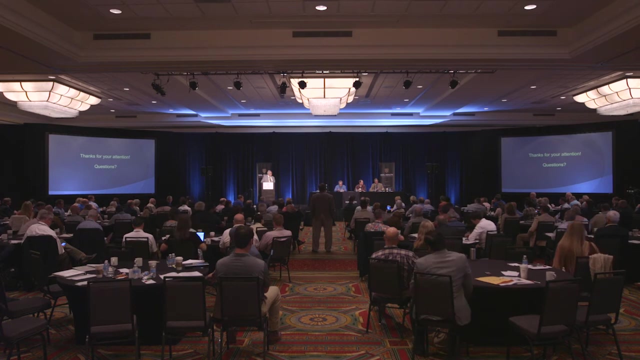 microbial Community and and reducing the protection, if you will, of organic matter in in, you know, the physical protection in a way that that then, uh, you know that organic matter is is quickly respired. so I think you know you, you sort of want uh both in a way. you know you want respiration and and healthy soil activity, but but you want to. 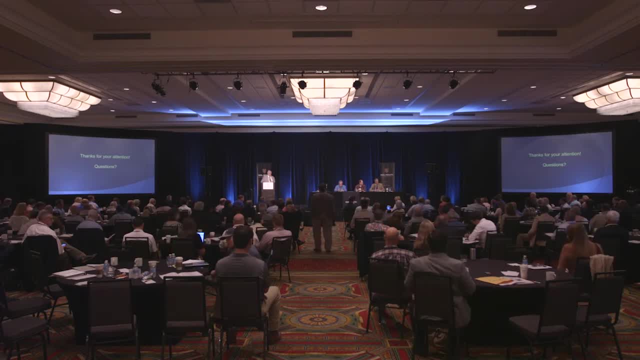 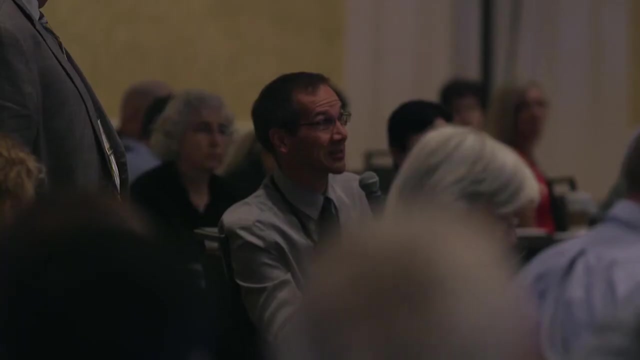 manipulate that balance to to increase the stocks? okay, one over here, tom brosno, the international plant nutrition institute, and again a question for dr paustian. he showed some impressive rates of soil carbon sequestration. my question is, i guess: can you achieve that without increased net inputs? of nitrogen, thanks, we do need to increase nitrogen. i, you know, i certainly go along with the idea that the stoichiometry of of organic matter in soils is such that you, just you know, with the exception of, maybe, biochar, you can't, you know- have soil organic matter increasing. 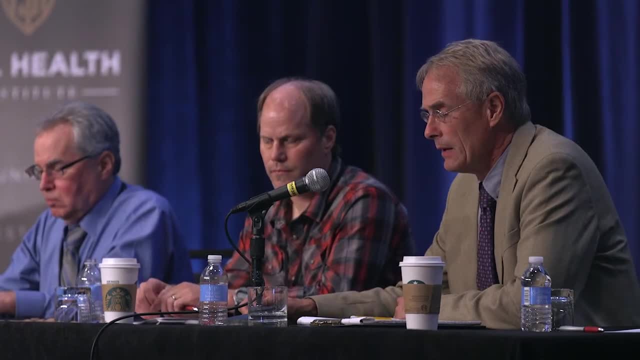 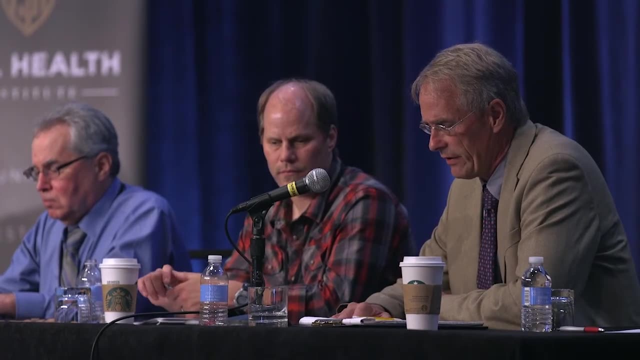 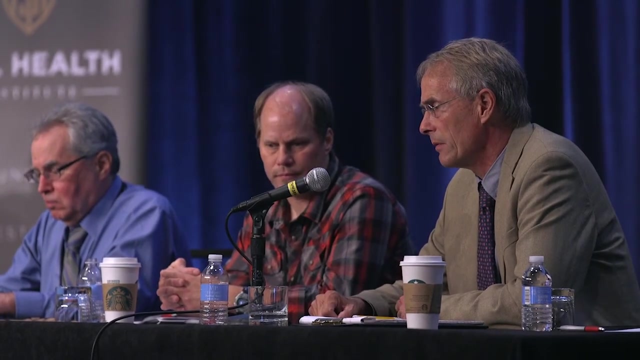 without having soil organic nitrogen increasing as well. i think, however, that that the the concerns about that are are a little bit overblown. i think that, particularly if we're, if we can use, uh, legume cover crops and things like this, if we can manage our 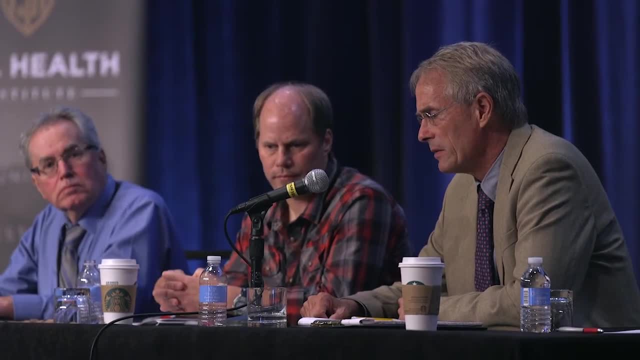 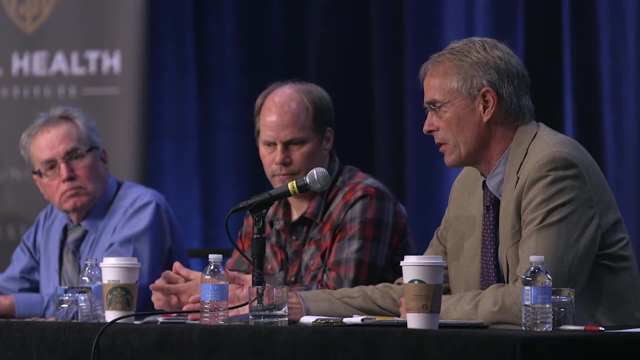 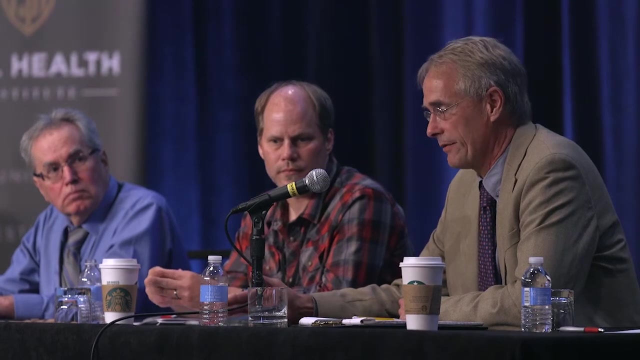 soil or our rotations. well, that we can meet the nitrogen requirements to a large extent. you know, we certainly if, if, if, in order to have high rates of soil carbon sequestration, we need a lot more inputs of of mineral fertilizer from haber bosch process, that's. that's a big problem, but i i would. look to to 2, 3, 1. i think that's that's a good way to put it. it's it's a good way to. i think it's a good way to put it. i think that's a good way to put it. i think that's a good way to put it. 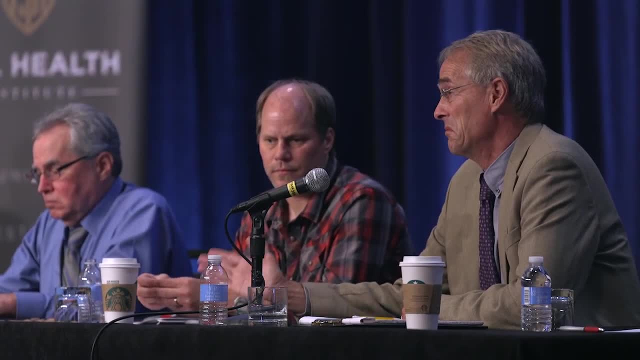 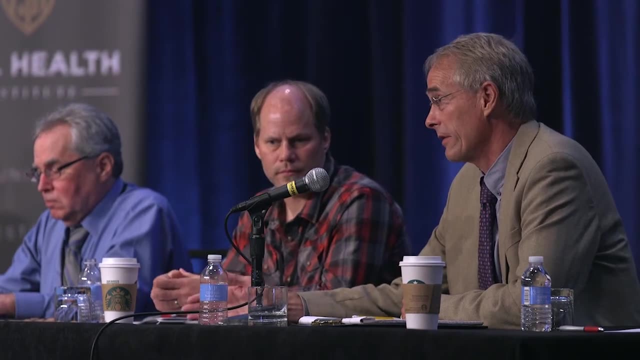 things- nitrogen fixation and you know, really important for this crowd. we lose a heck of a lot of nitrogen to leaching and to other kind of gaseous losses If we can reduce those. you know we've got a lot of nitrogen sloshing around in the system. 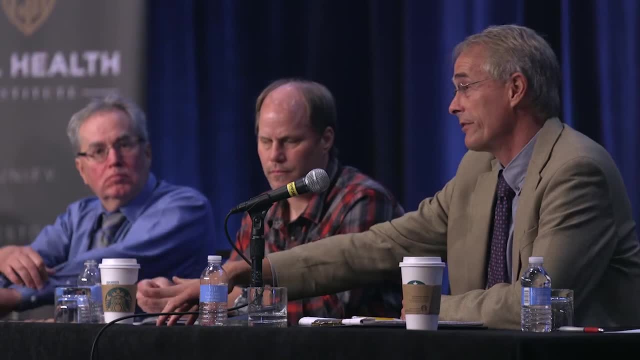 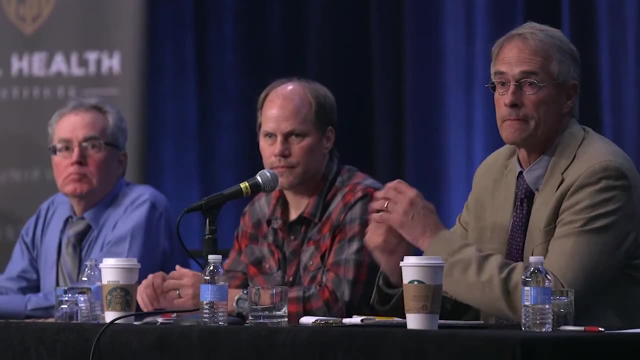 Let's get that nitrogen out of the Gulf of Mississippi and let's get it into soil, organic matter, And I think that's what we can work on. Male Speaker 2. Another question: Female Speaker 2. Then you're talking about this genetic index. 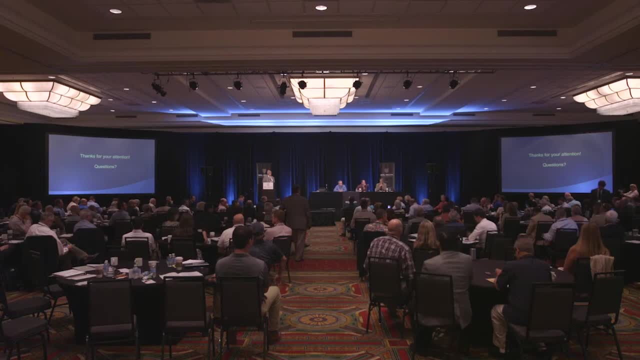 And I have actually kind of a three-part question. The first thing is that we know that gene, existent or present, doesn't mean expression, And you said that there is kind of a talk about doing using DNA instead of RNA. We know that the expression and presence is different with both methods. 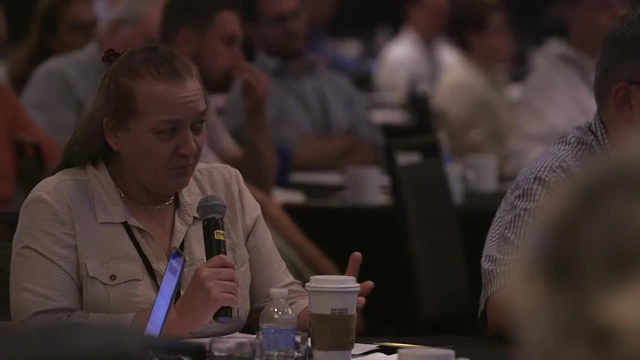 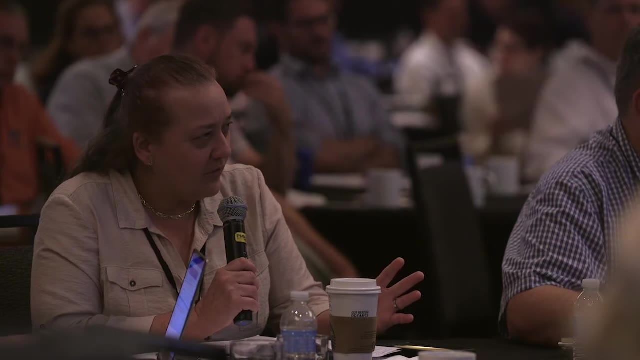 So are they using both to give you data, to prepare that? So that would be kind of a little bit of comment. The second thing is that you didn't want to insult people. That's what you said about not using the weather or the climate, but the soil. 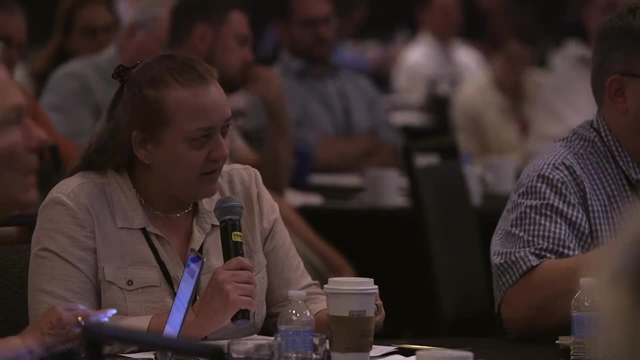 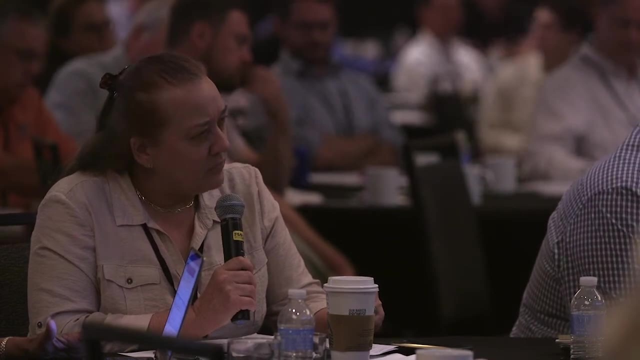 But there's one concept that says epigenetics, And you know that that is coming hard and heavy And that will influence totally your results or how you, I would say, explain your results. And the third part- and it's also related with this- is if you have any standard methods. 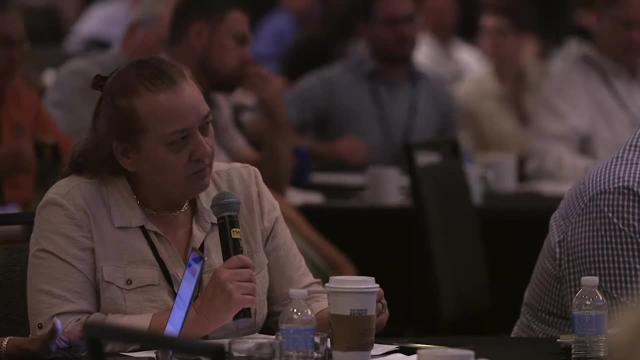 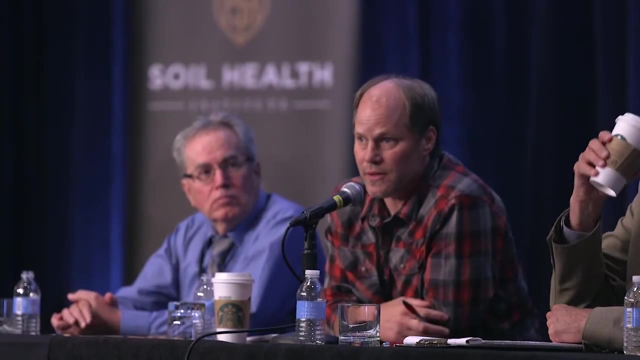 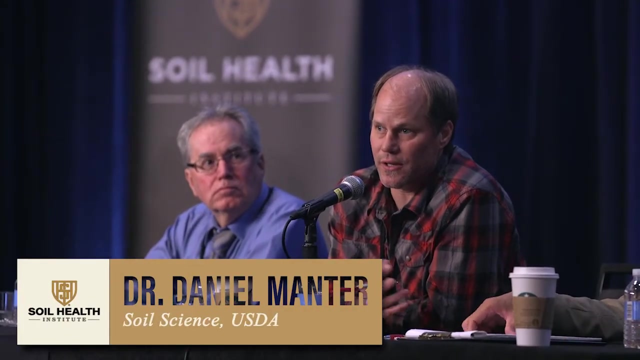 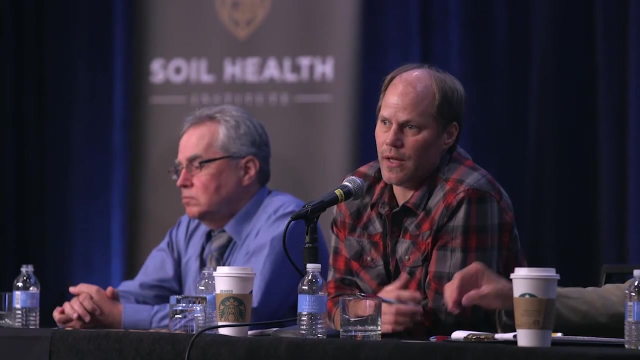 that you're recommending people to give you from the field to the lab. Male Speaker 3. You're right. You're absolutely right that gene expression is important And under certain circumstances, will give us a better answer than others. I think the biggest reason we've avoided that at this point is cost. 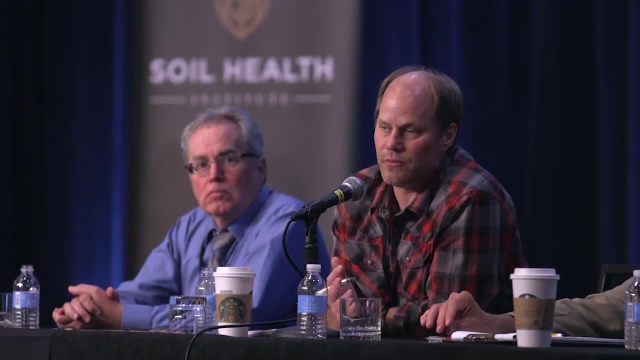 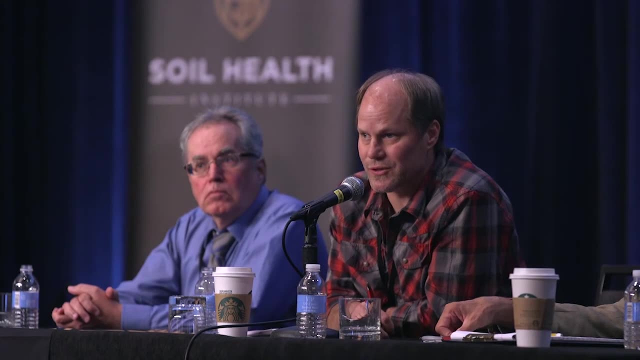 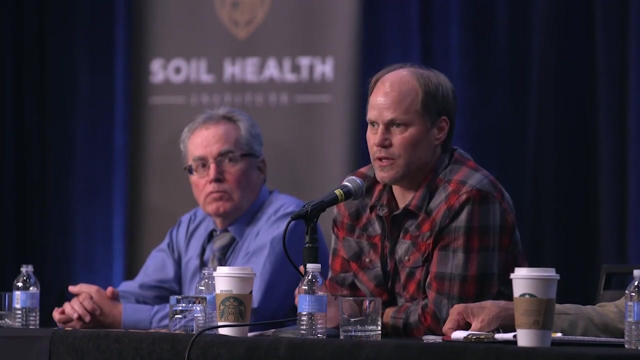 In order to do the same technique with gene expression, our cost goes from about, you know, $50 a sample to, you know, $2,000 a sample. So, and then, what we've tried to do is we're looking at general patterns. 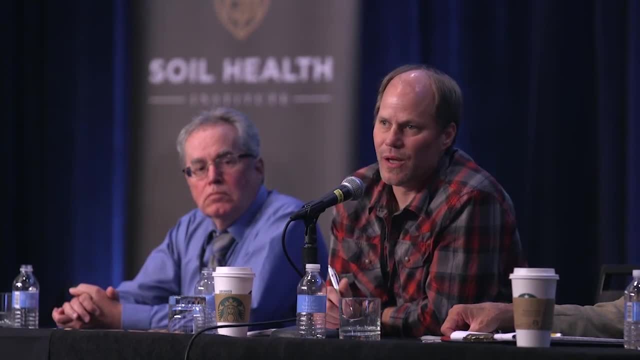 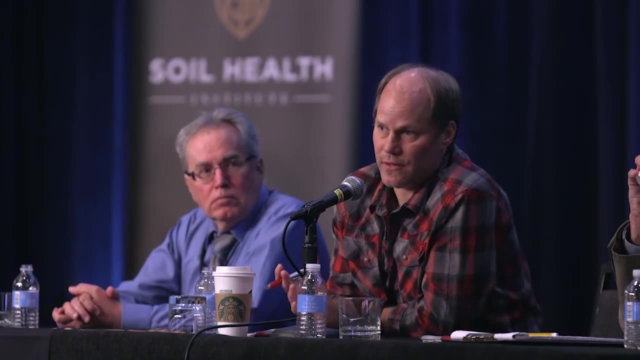 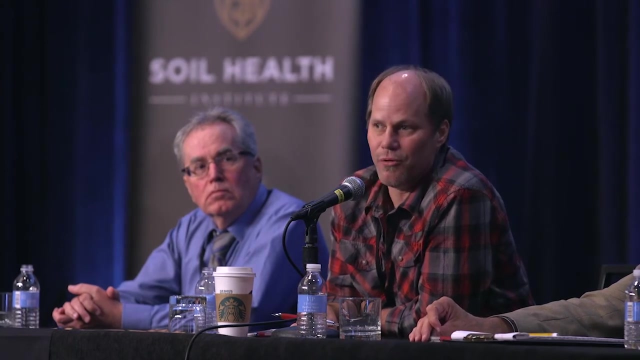 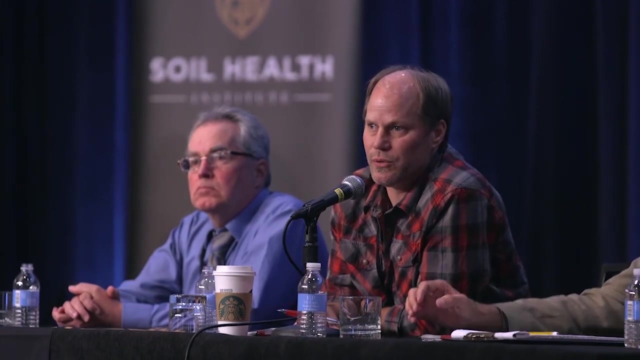 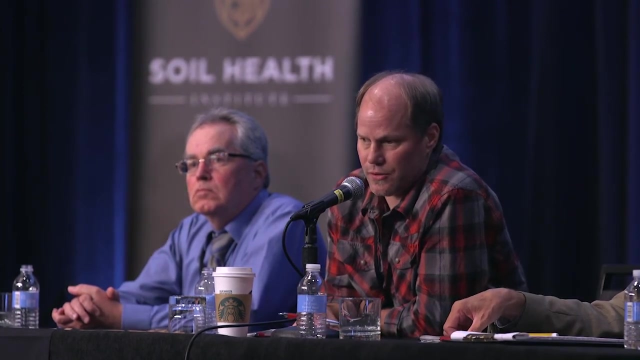 So in general, maybe the whether gene expression is worth that is, I don't know. Epigenetics: That's a great question. We know so little about its role in microbial communities or populations. at this point We're just sort of scratching the surface with individuals. so 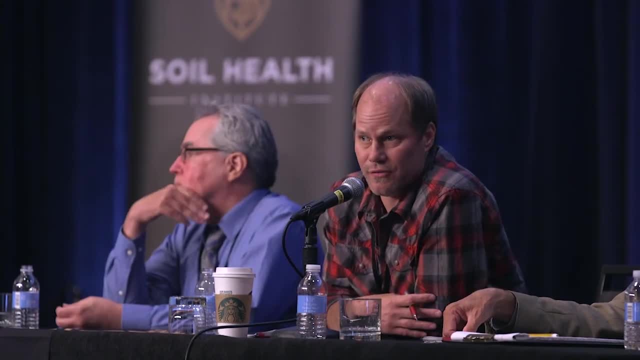 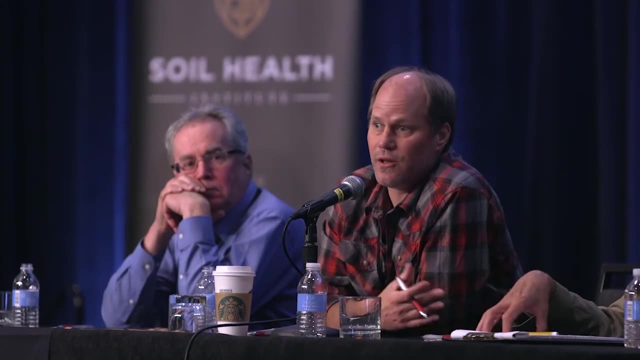 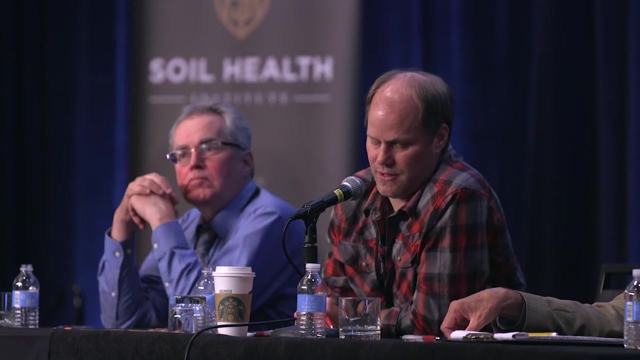 But you're. but we do know that, yeah, environment is going to affect epigenetics, And so that has more again to do with technical, technological limitations at this point. And then your third question. I didn't write down. 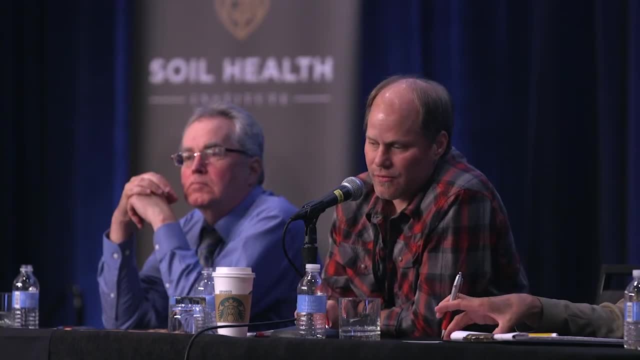 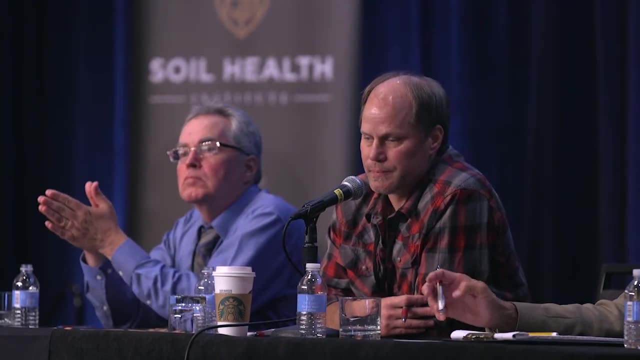 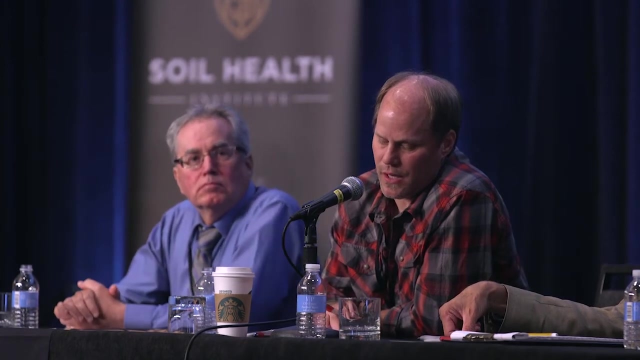 So for that, that's one of the reasons we've stuck with DNA too, because it's much more stable. So- and there's still a lot of debate- There's some, really a couple of good papers that, and work we've done too, where we typically 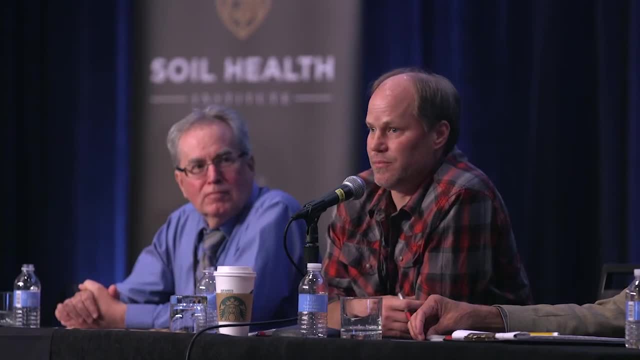 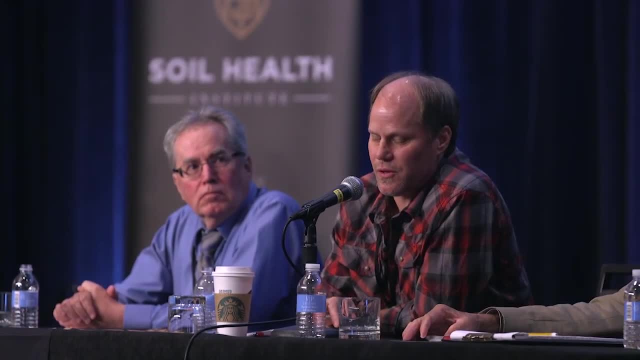 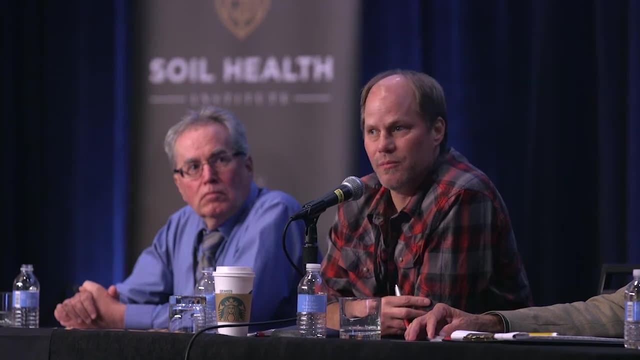 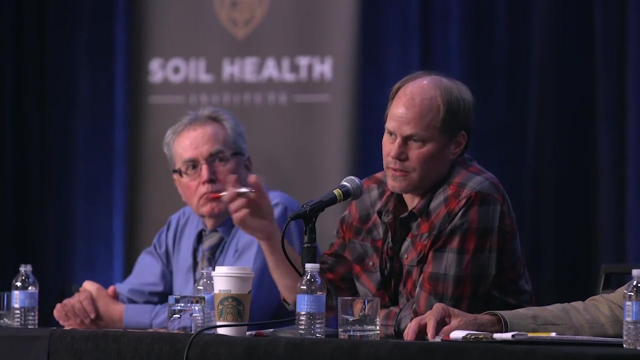 it on dry ice, But there, I think, in order to just get the general characteristic of that community, we may not have to be quite that careful. So you don't want to leave a sample on the dashboard of your pickup truck, but in a cooler. 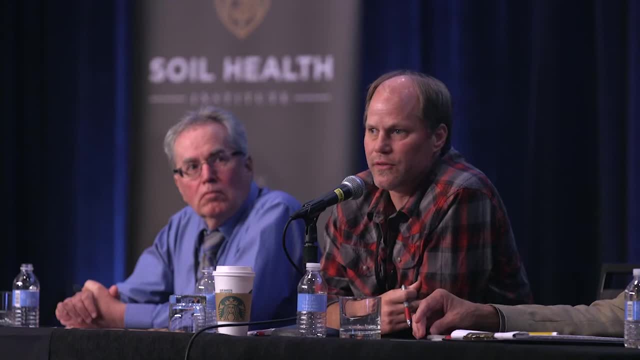 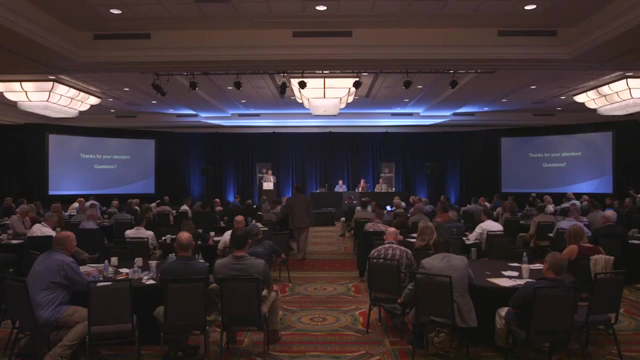 and scent on a cooler. you don't want to leave a sample on the dashboard of your pickup on a blue ice, and then we process it as soon as we can and when it gets in. can you hear me? yes, hi, my question is for Bob. yeah, my work is in the world of 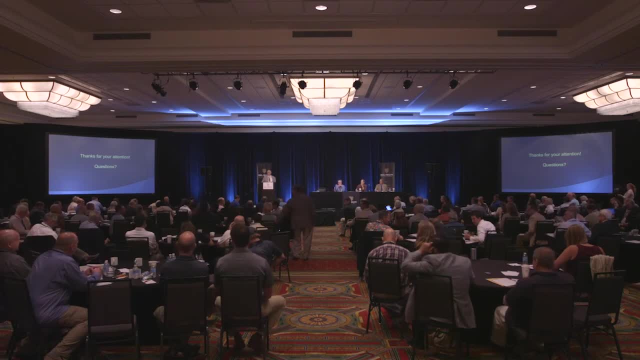 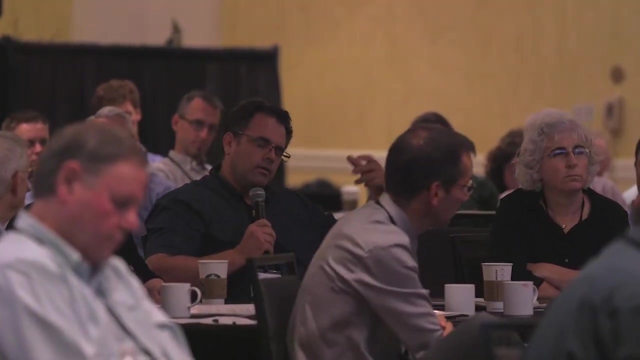 building these extraordinary public parks and landscapes at universities- and we usually have projects- will require us bringing in 100, 200, 300 thousand yards of design soils to make these landscapes with. we've gotten to the point that we've got the owners to give us a six-month lead time and we've gotten 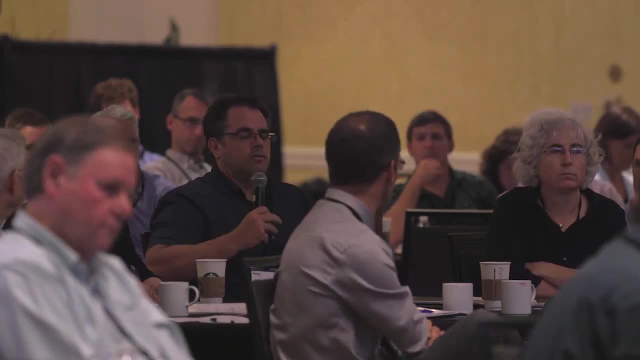 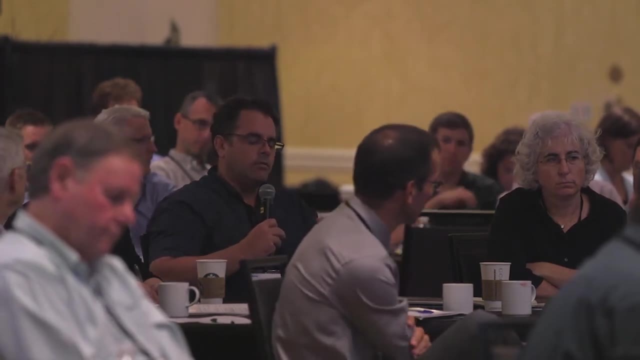 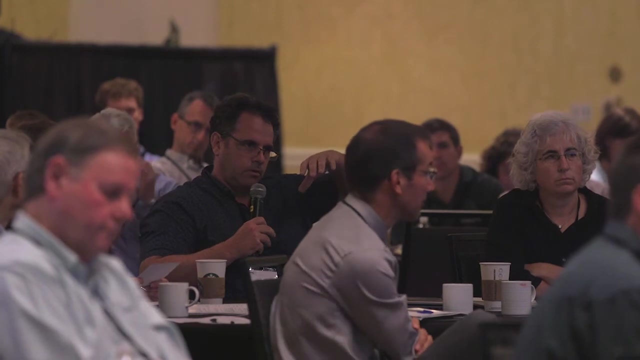 to the point where we know that black-eyed Susan's produce large volumes of BAM spores, so we can inoculate. our soils are ready with the BAM spores going in, so the plants and everything can grow. I was curious if we expanded that time frame longer and we did your disease suppressive work. cover crop two: years ago and we did your disease suppressive work cover crop two years out and they did a soil improvement program the following year with the soil improvement. have any negative impacts on the disease suppressor program that we would do originally? you know like, as you transition from disease suppressive into a higher, more organic type soil would have any negatives? generally not. you know, each system is a little bit different and and so it's hard to totally generalize, but in general a lot of these kind of things that that are developing disease suppression programs would have any negative impacts on the disease. 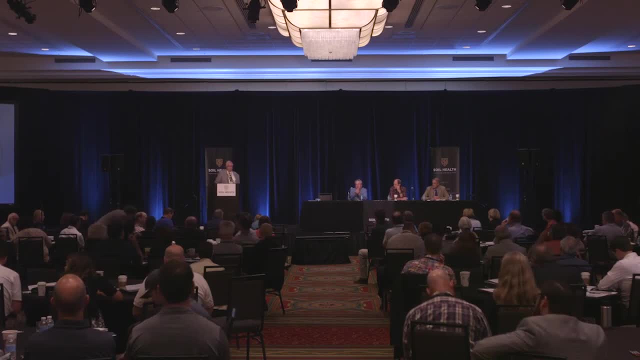 suppression the kind of organisms that are that are selected for or that that are useful for the disease. suppression a lot of times a soil that's got more healthier profile or or some of these characteristics that that that we strive for in soil: health, like increased organic matter, net, those kind of properties a lot of times help those kind of organisms survive better. so I mean it's it's it in most cases, if you have a healthy soil to start with you, you've got more of a favorable environment for some of these organisms to to survive and thrive, and better one. one aspect of that that we see a lot is 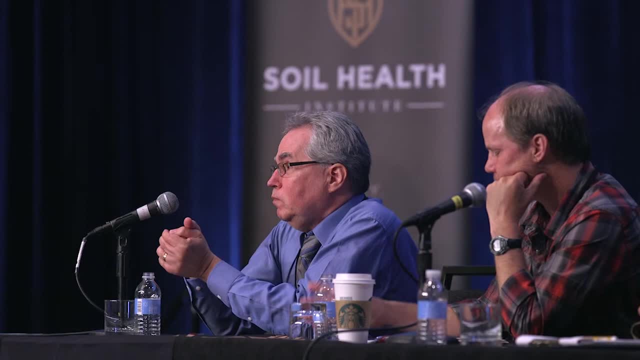 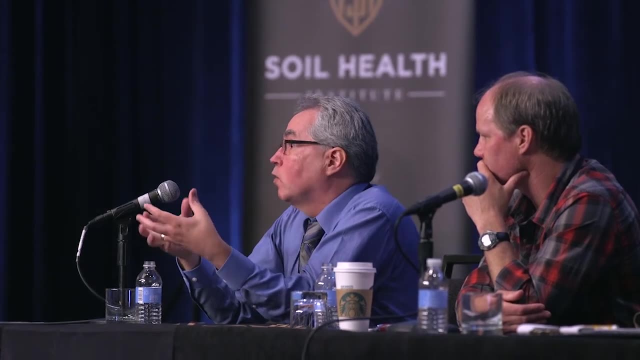 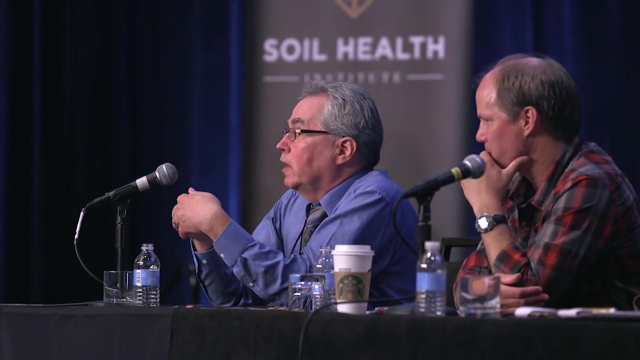 like in like use of biological controls generally. if the use of biological control in a poor soil does not work to improve the health of the soil, work very well because they aren't able to survive in there, but those same organisms put into a soil that's got a better rotation, a healthier system, and they work well. And it's a similar kind of thing with some of the disease-suppressive organisms. So there are—it is possible, though, that some of the practices could interfere with the specifics of some of the disease-suppressive things, like with the brassicas and some of. 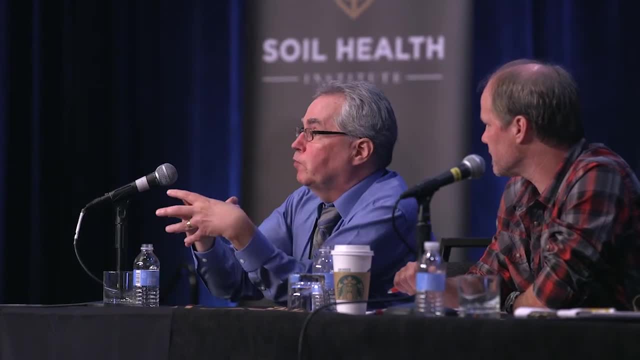 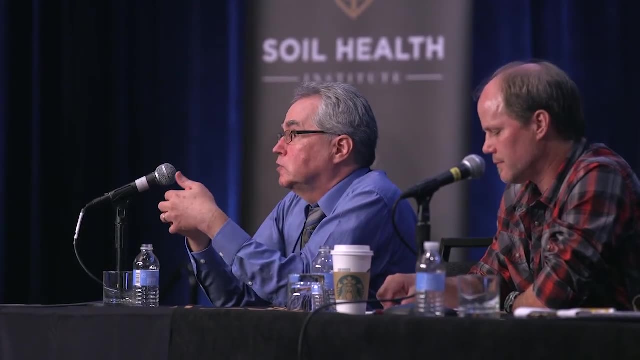 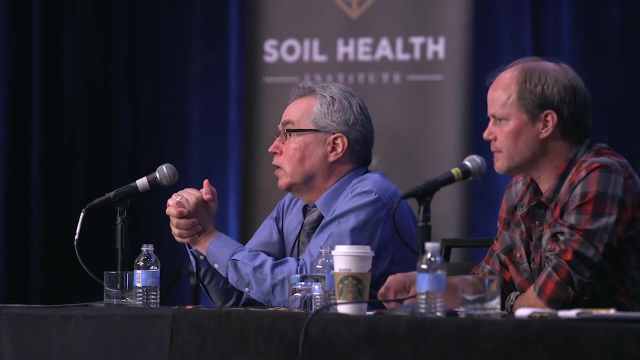 the things like that that are kind of shifting population to a particular group of microorganisms that are important for disease suppression. There are things that may disrupt that and shift that so that they no longer are there. But I would say in general that the healthier the soil is to begin with, the more supportive 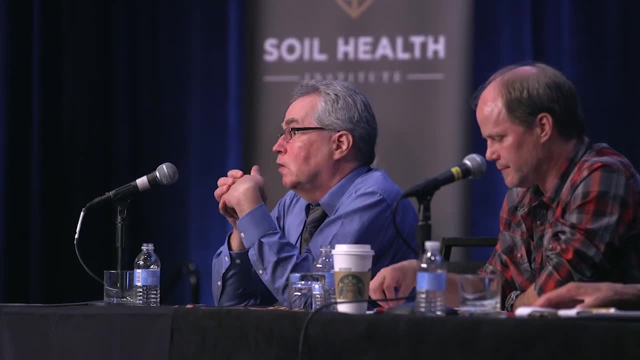 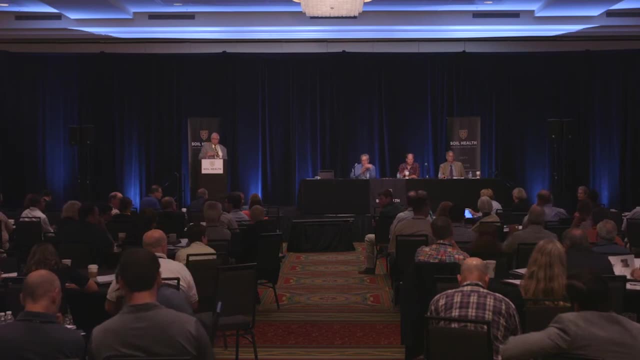 it is of some of these other practices that can lead to disease suppression rather than undo them. Male Speaker. 2. Next question over there. Male Speaker. 3. Male Speaker. 5. This is for Dr Postian Mulvaney from the University of Illinois came out with a very controversial statement about. the introduction of synthetic nitrogen actually increases respiration, therefore decreasing soil organic carbon or soil organic matter, to the chagrin of the corn folks in Illinois. But I'd just like to have your input, your thoughts on that. Male Speaker 4.. 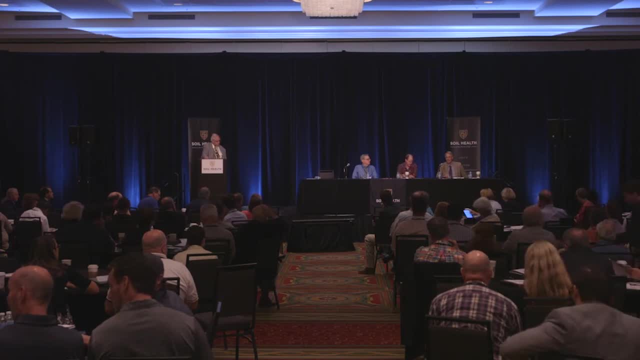 Yeah, been a lot of discussion around this. I guess I've also. back when I was a post doc, I remember I did a lit review and if you look at long-term experiments and comparing crop rotations at different fertilizer levels- a good example down at the University of Kentucky- they have some long-term no-till versus. 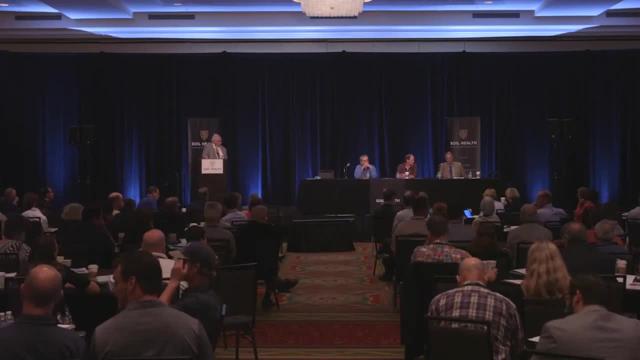 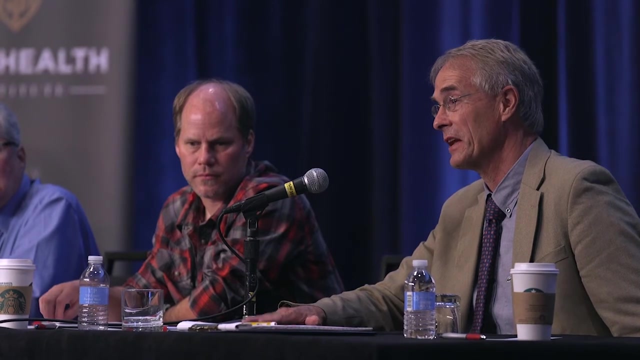 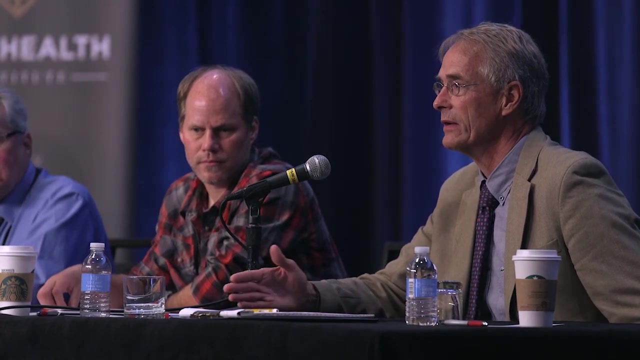 conventional till at four different fertilizer levels. and there you, you know, you see, as you increase nitrogen inputs, fertilizer, you increase soil carbon storage, not a big mystery. you get a lot more productivity, a lot more residues, a lot more root growth, a lot more carbon inputs going in. so from that standpoint, 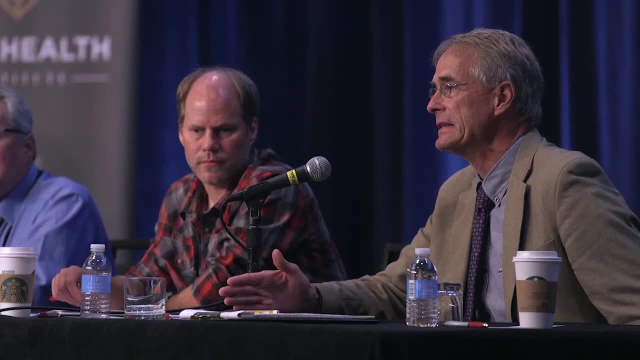 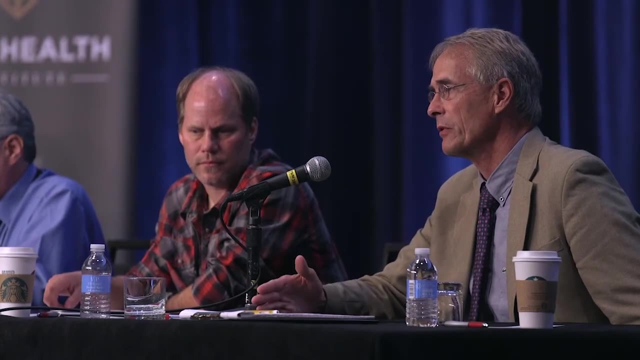 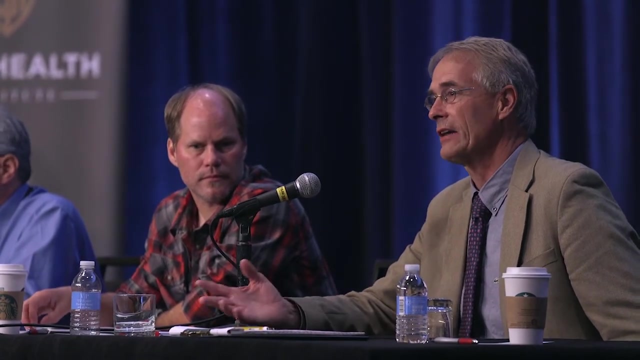 you know, I think on the input side- you know, you, you- there's good reason to say that the opposite occurs now. that being said, it's not that you would say, gee, in order to increase our soil carbon, we just need to put lots of nitrogen out on the environment. right, that's the way to. 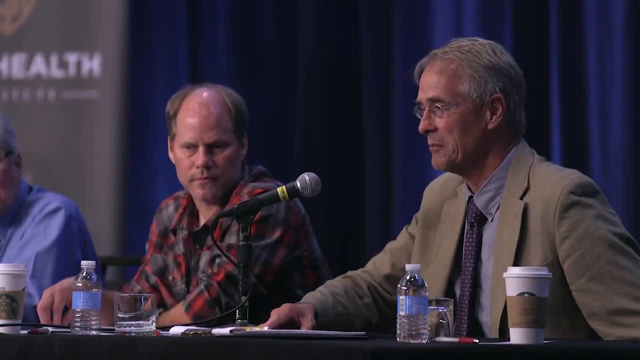 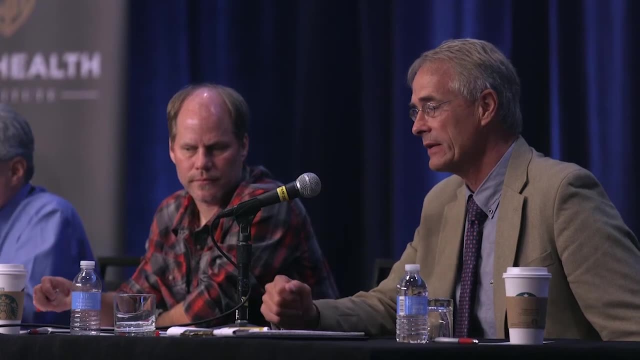 sequester carbon. well, it's not, because some soils, you know, don't need any more nitrogen than they're already getting and some maybe need less. and, of course, the big issue with nitrogen is really nitrous oxide emissions, which is probably. a big issue with nitrogen is really nitrous oxide emissions, which is probably 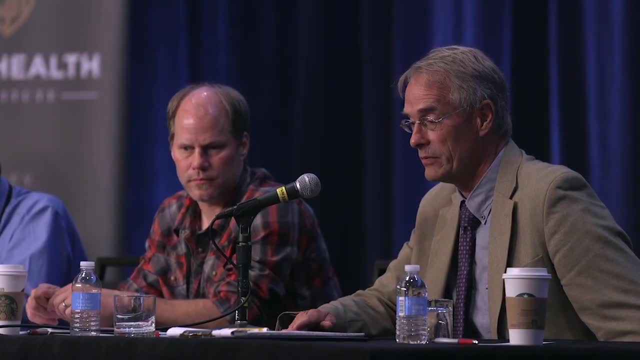 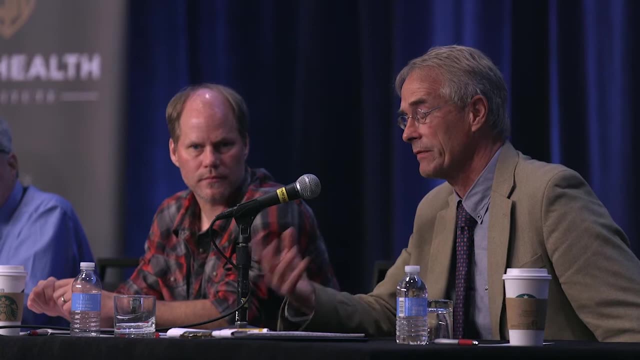 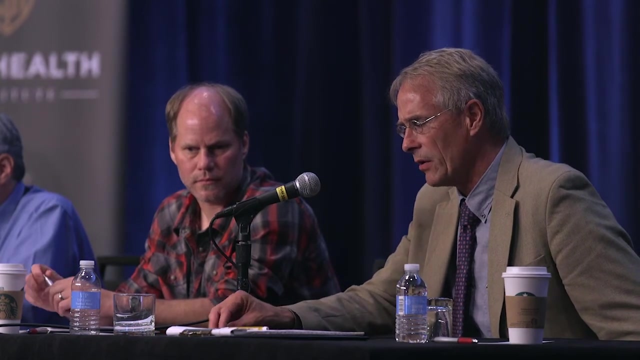 most people in the room here know that. you know, nitrous oxide relative to co2 has about 300 times the effect in terms of how it affects the, the radiative balance, if you will. so you know, I I guess, in summary, and I'm not sure I'm- 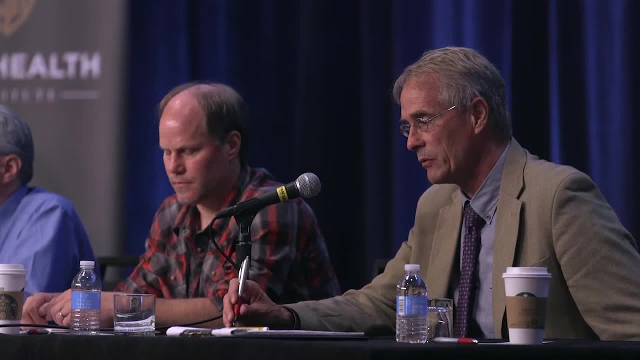 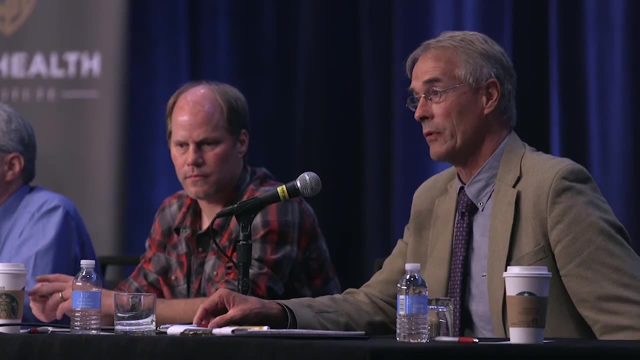 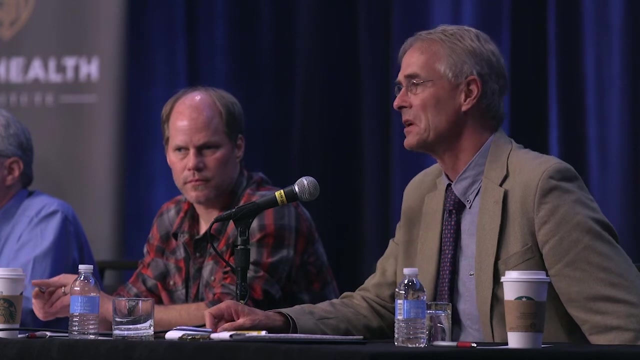 asking your question. but you know, nitrogen management is key. I wouldn't say that that nitrogen is bad because it, you know, increases and you know increases increases soil respiration or something like that. In some cases it might if the microbial community is nitrogen deficient. but I would say in most ag soils, I would be a bit surprised to see that Nitrogen is needed to maintain the productivity. so it has a plus, but I think it boils down to you need to use nitrogen in a way that maximizes crop productivity for the system. that you're using and minimizes losses. If you do that, you're probably going to get your most bang for the buck in terms of carbon storage and you're also going to get the least amount of nitrous oxide emissions directly, as well as other nitrogen losses that contribute to eutrophication. 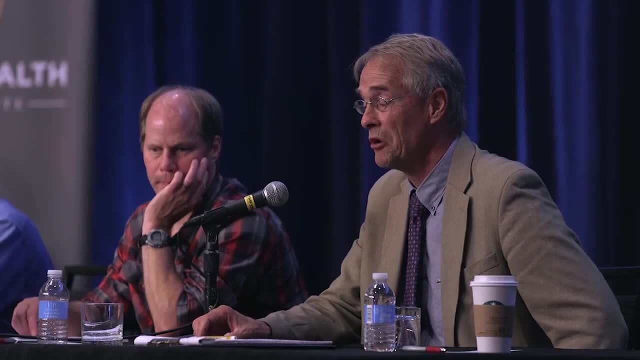 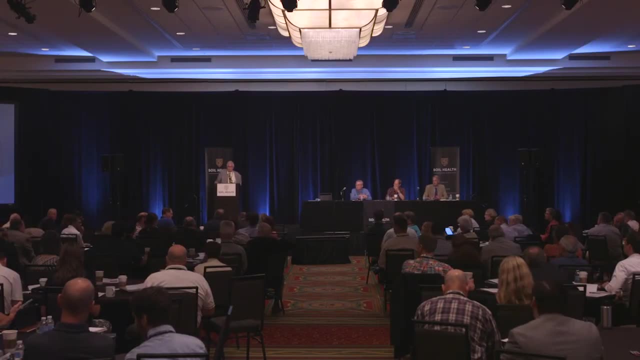 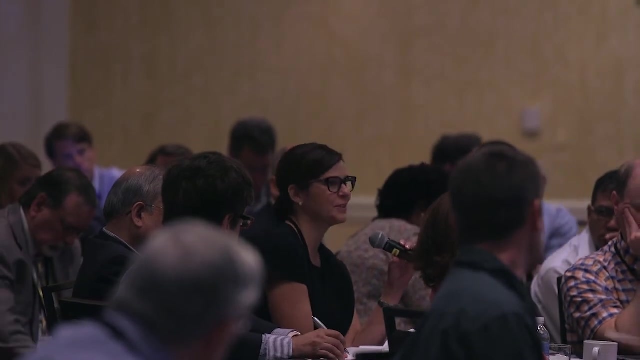 It's all about how you manage that system. Another question over here. Hi, I'm Christine Morgan from Texas A&M University and my question is for Keith Postian. It's a really simple unit conversion and spatial interpolation question and it has to do with 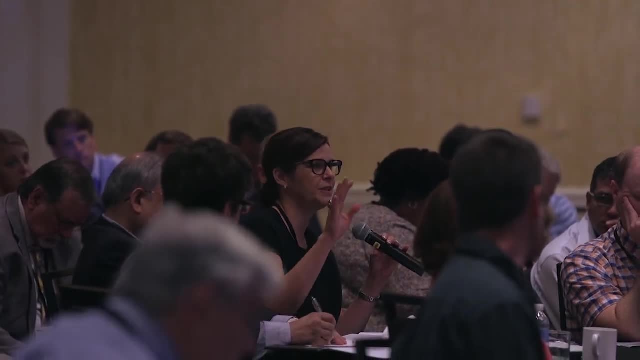 some of the work you've done in looking at carbon sequestration in managed agriculture. If we were to take that sequestration amount and put it in a different way, how would that work? How would that work? How would that work? 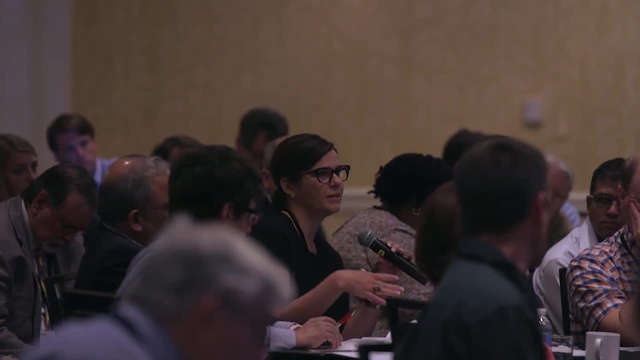 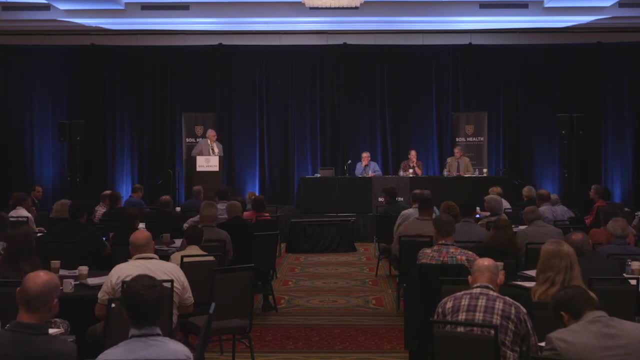 Does the cat per mil fall within the range of some of your estimates? Yeah, sort of The four per mil or the cat per mil is kind of at the upper end of that And you know there's certainly a number of our whole industry has been doing this. 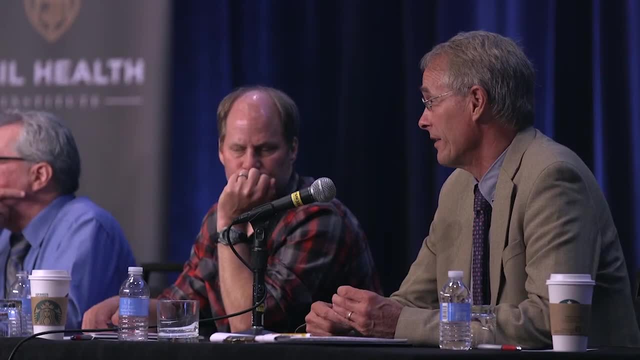 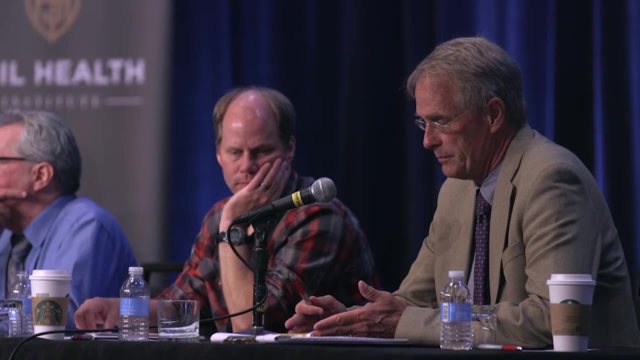 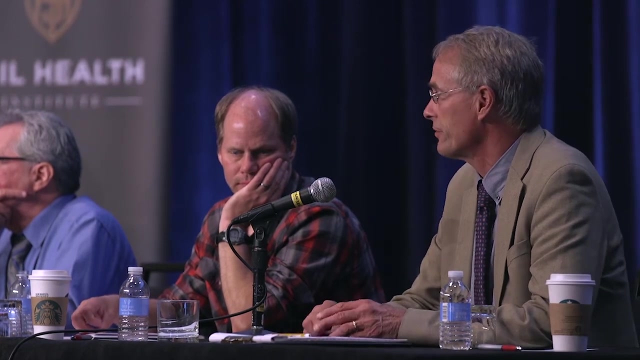 of very prominent scientists that know, that have been working in this area for decades and that are- you know that are, have signed up, if you will- to say that this is an attainable goal. You know, potentially I think it. personally I feel it's kind of at the upper end, but 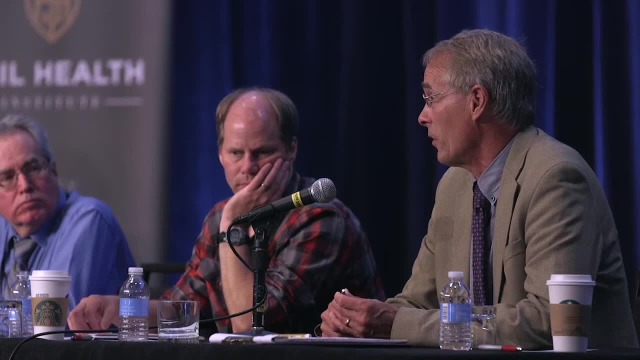 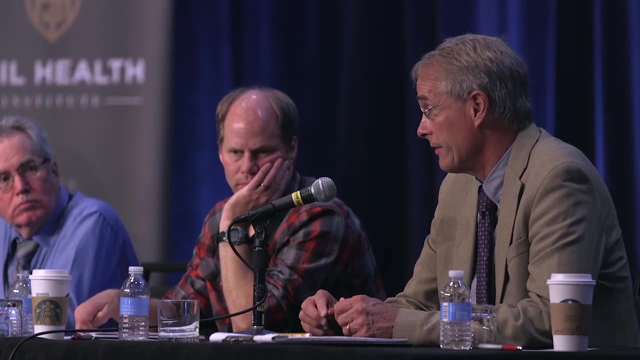 again, I would characterize it, and most of the scientists involved in that as well as I. well, I can't really speak for the policy makers, but I think that people have expressed it as this is a, you know, an aspirational goal. 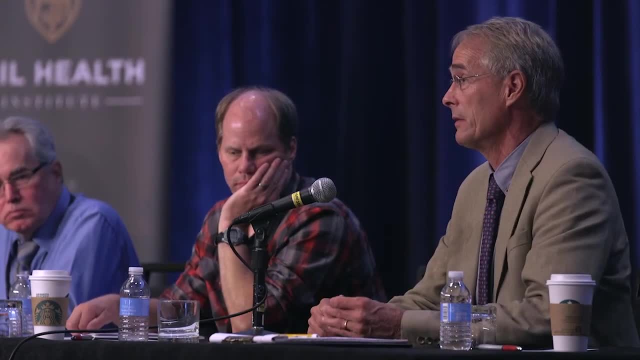 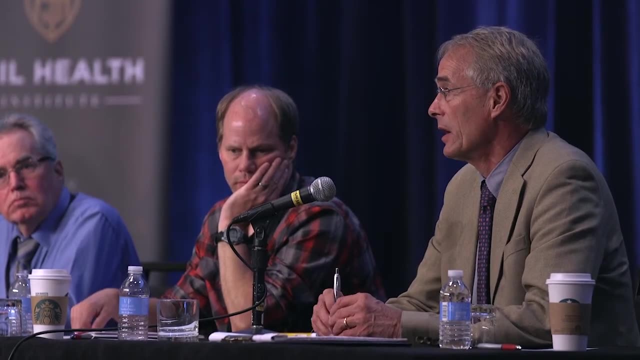 This is, we want to set the bar high and really see, you know, can we, can we, can we get close to that? And I, I don't really have a problem with that. And I would say also to me right now, and what I try to point out with this, you know, 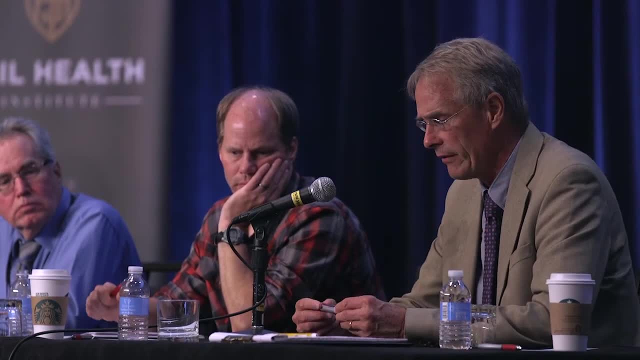 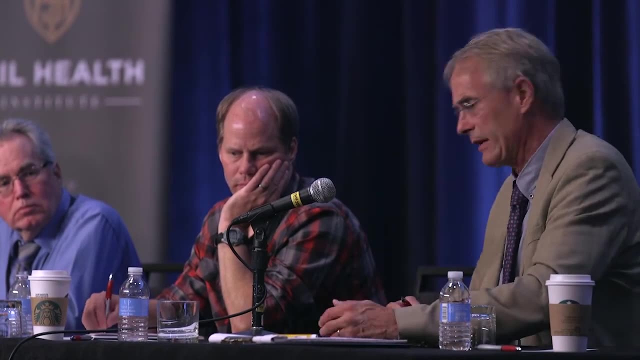 looking at the, at the studies that have really been done over the last 20 years, the bottom line to me is: Is that okay, different? we've come up with different estimates and I've done estimates and and Deb Basio and different people have have gone through the numbers and and they're. 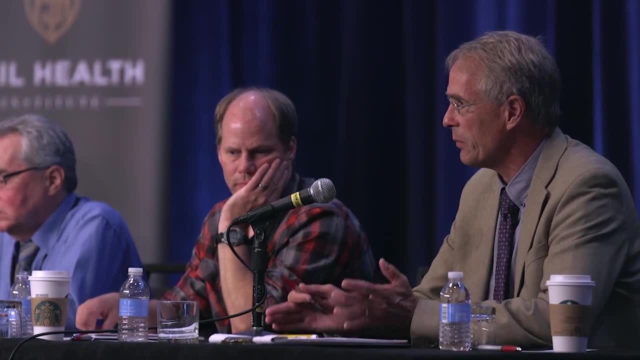 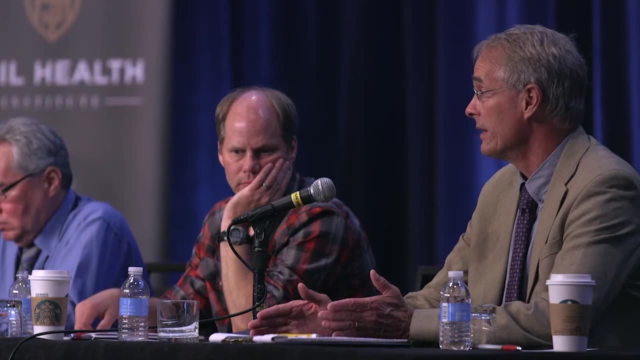 all a little bit different, but they actually kind of converge and and the bottom line to me is: hey, the numbers are big enough to matter, So and- and we don't really at this point need to know much more than that- 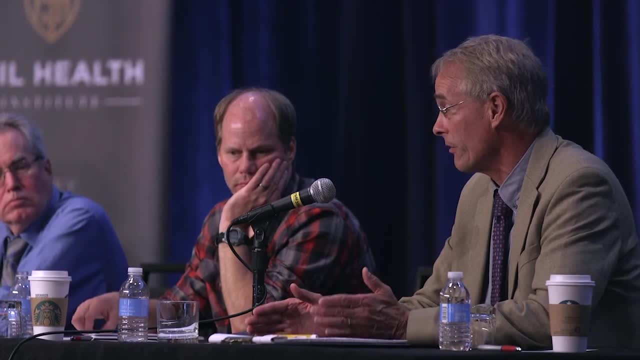 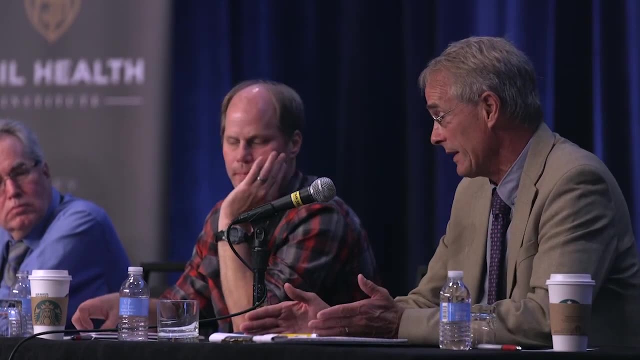 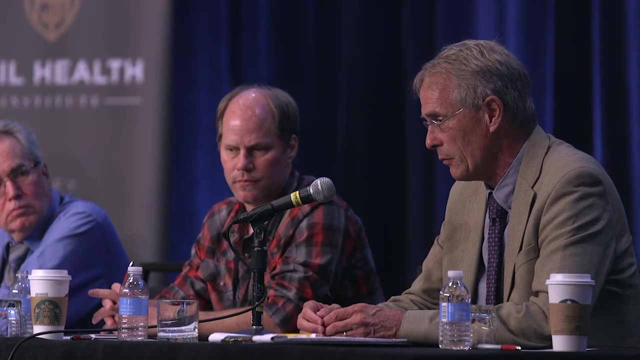 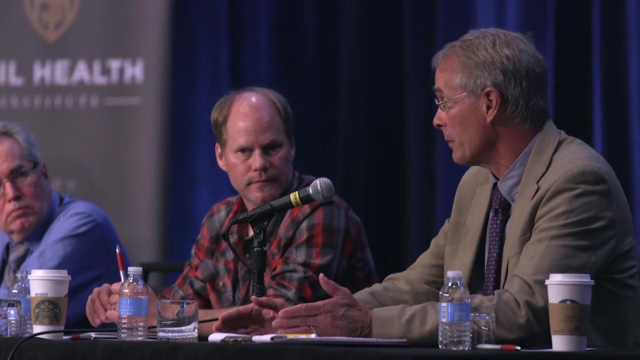 What the crucial thing is, though, is that you know that's the technical potential. So, yeah, What's the, what's the you know, what's the economic and policy potential, what you know. how do we incentivize farmers to get really wide adoption of these practices? 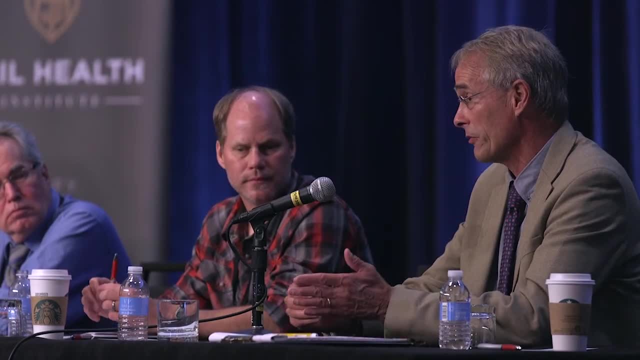 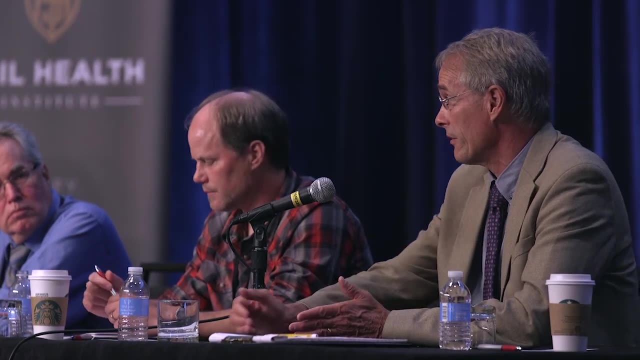 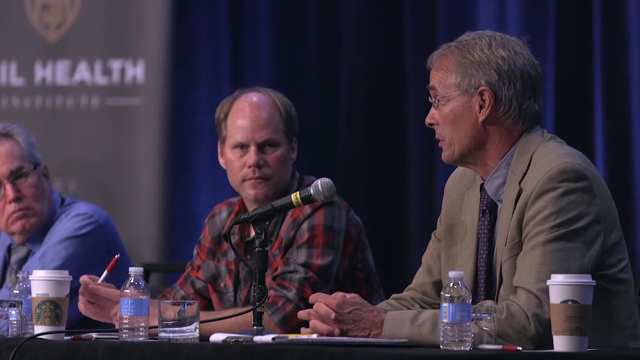 Because that's what we're going to need. You know, we can have these great technical potentials, but if we don't get the folks on the ground to do the best management to, you know, increase their soil carbon stocks, then then we won't have really anything to show in terms of of carbon removals into. 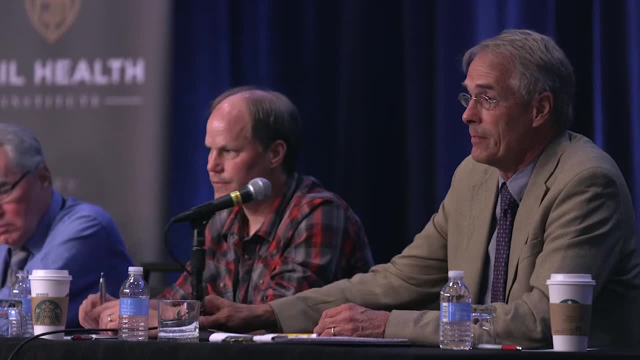 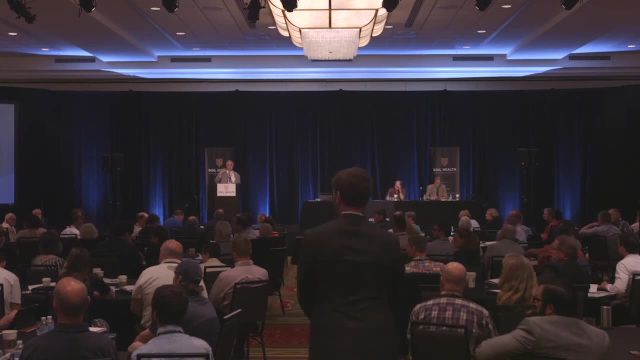 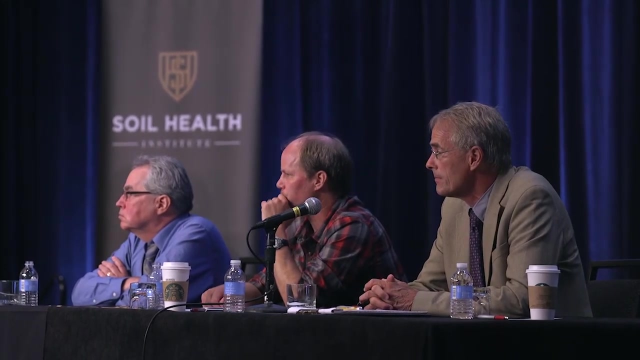 bio into agricultural soils- Question over there. My name is Chris Fennig, with MyFarms, and I wanted to open a question for the entire panel, Anybody that would be willing to share Any strengths or weaknesses that you found in using any of the soil, carbon or GHG models. 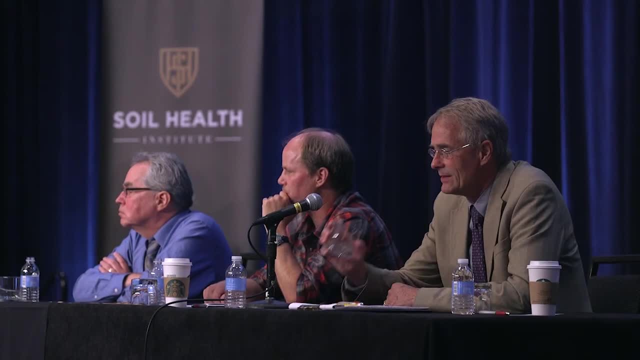 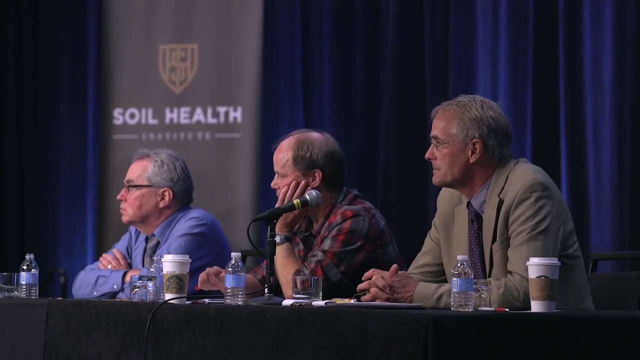 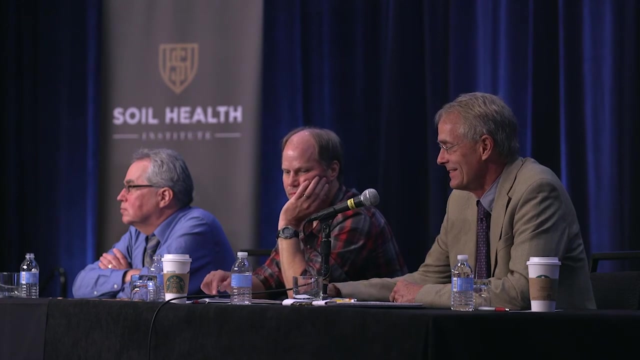 that are available. specifically, the USDA has the comet farm tool currently in production and the century model was, I think, published back in the 90s. So any any strengths or weaknesses that you see in your experience using either of those two approaches. 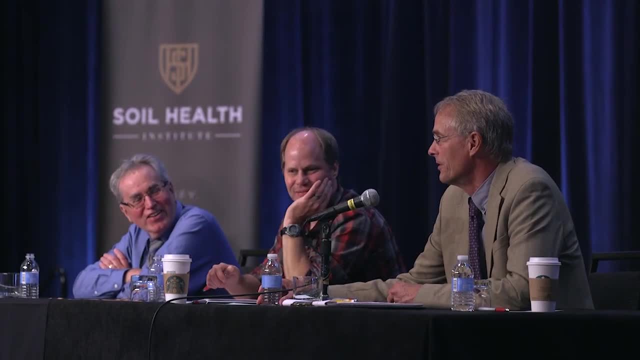 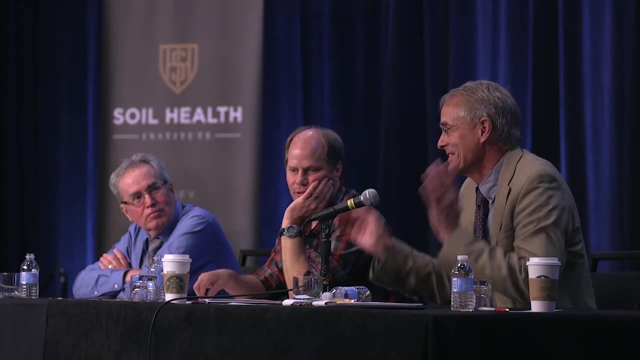 I'm going to recuse myself from both those, Okay, Because I've done quite a bit of work on those, So I'll let anyone else say what they want and and it's all right. So if you have bad things to say, let's hear them. 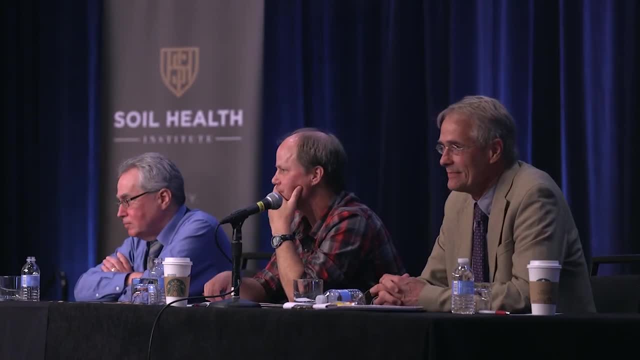 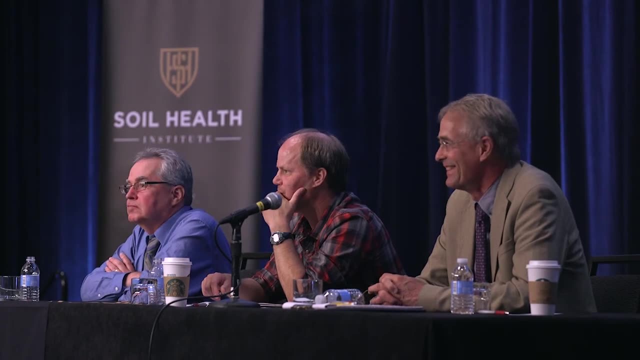 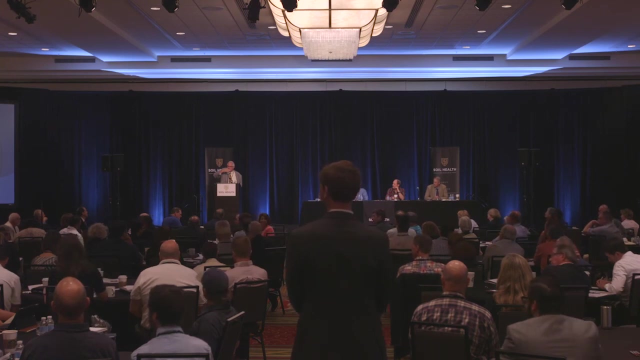 Looks like we'll have some comments from the audience perhaps. Nicely done, Keith. Well, I'll just toss in that your question is right, Jermaine, if you're looking for another participatory conference to go to next month, and that is the Tri-Society's. 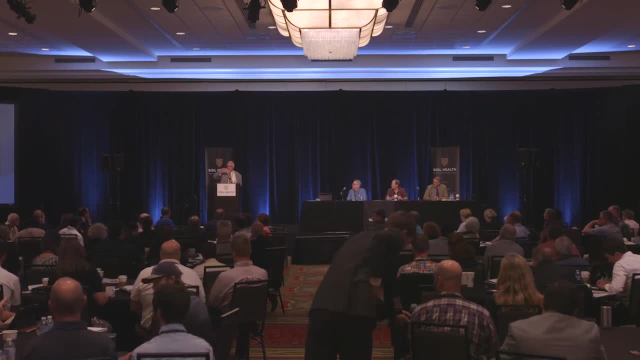 agronomy, crop and soil science society are hosting a workshop in Sacramento to really address the interaction between carbon intensity, life cycle and other modeling estimates and soil organic carbon storage And the goal from the Tri-Society perspective again, which is another partner with the Institute. 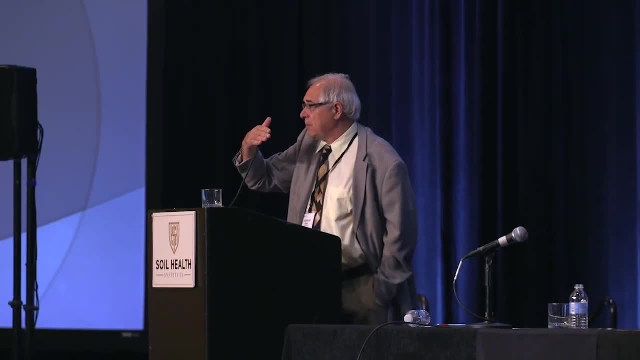 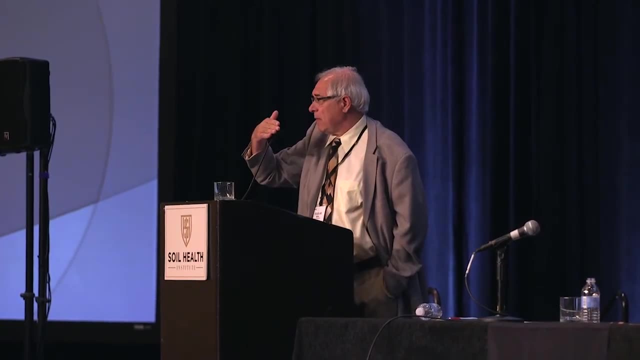 is to Okay. So come to, hopefully, a consensus of paper, looking at the at all the extremes, all the opinion, to see if we can bring science to bear on the question of what model? what are the weaknesses, what are the strengths? where, where should we go? 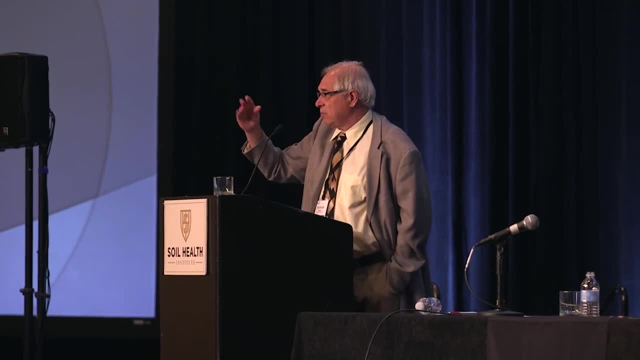 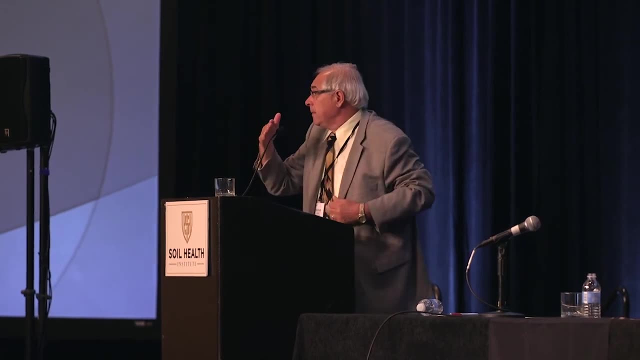 So I mean, it's another, it's another area, It's related to soil health, in my opinion as a generalist. so it's another opportunity for you. So let me, Can I, can I? I recuse myself and I won't say anything specifically about those models, but I'll say something. 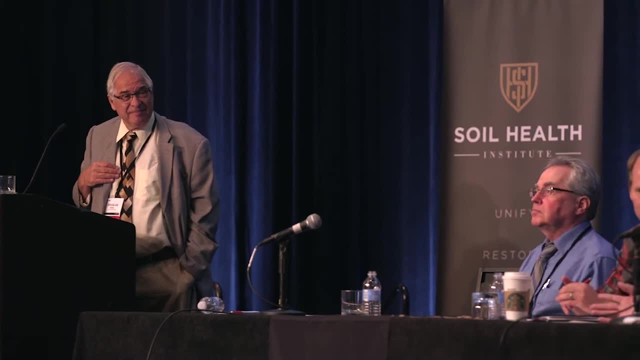 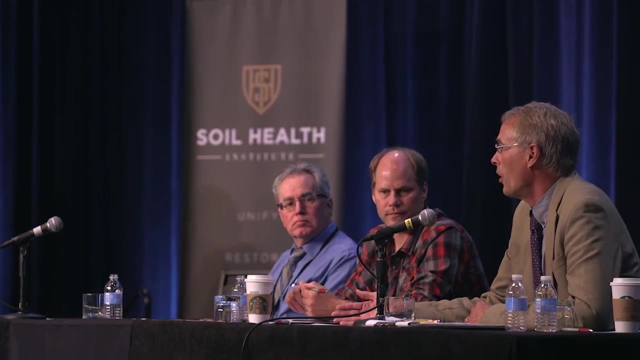 maybe in general. And that is, I guess, a couple of things. First as a modeler and a soil scientist. but you know the famous saying is that all models are wrong. some are useful. you know is kind of true, right. 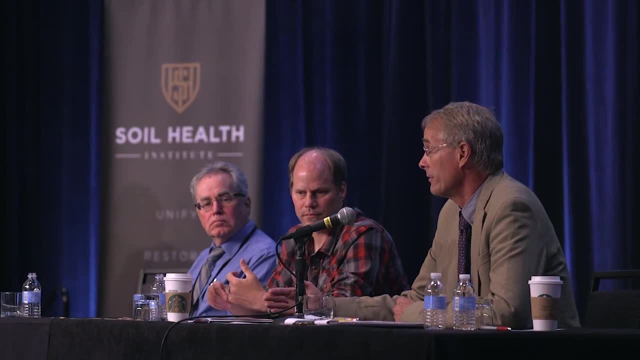 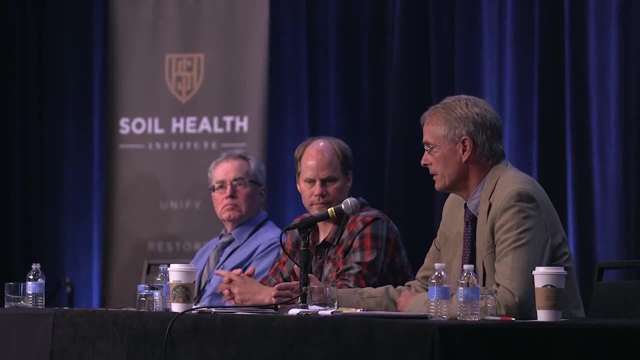 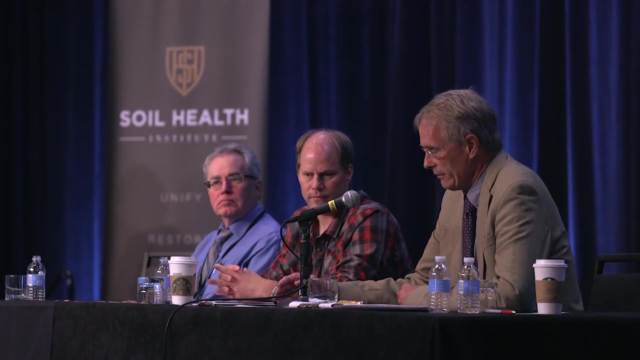 So we know our models are imperfect, but I would say this: you know, sort of on behalf of the entire community, I think we've made tremendous progress in terms of developing models, particularly process-based models. We have models that predict soil, carbon emissions and and certainly things like N2O emissions. 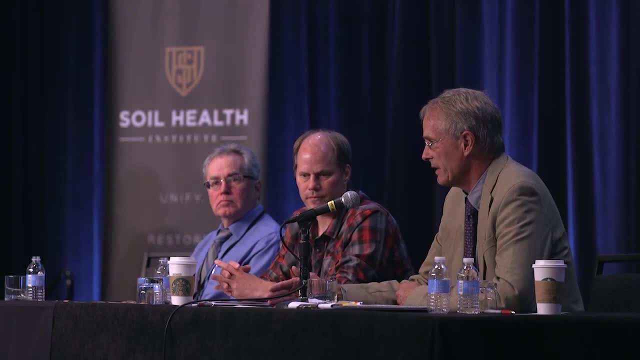 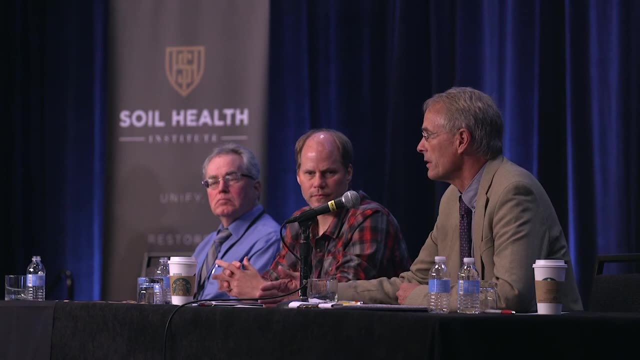 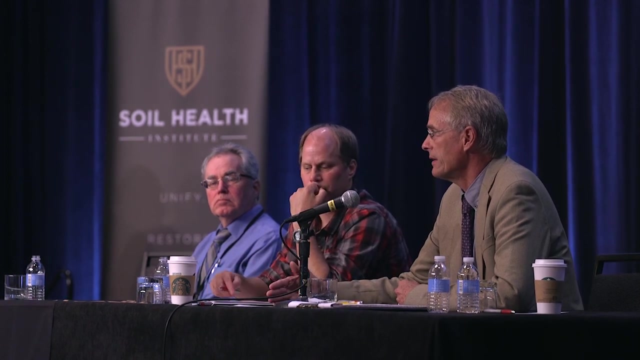 is a little bit tougher in my mind, but I think we've made tremendous strides there. We have models now that are quite useful for prediction and for for policy, for, you know, for quantification And going forward. I I think models have a crucial role to play and, and these decision 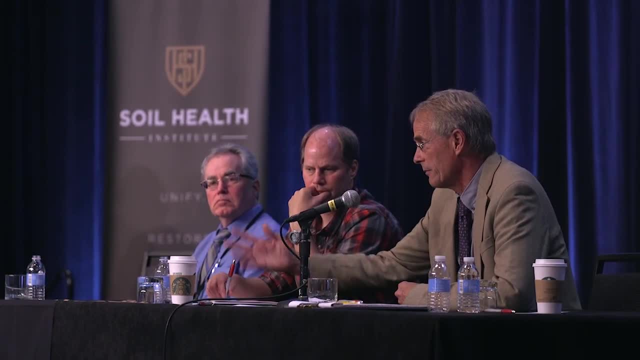 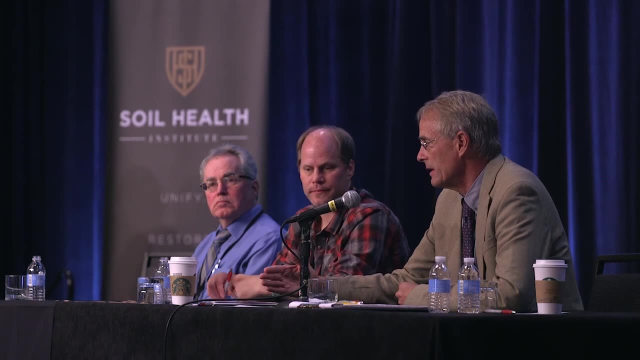 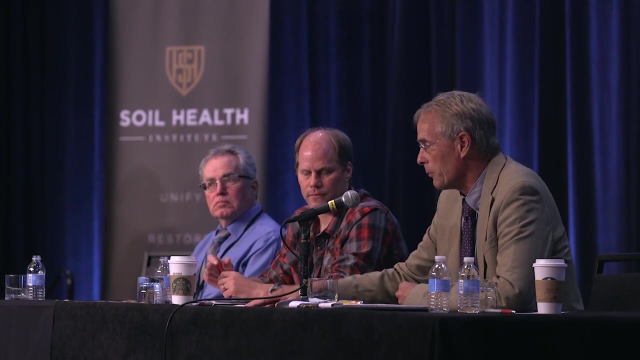 support systems that incorporate models like you know, like the Common Farm System, like it was mentioned, as well as some others, and that is that we are not going to, you know, if we're going to widely adopt practices and we're really going to try to track global. 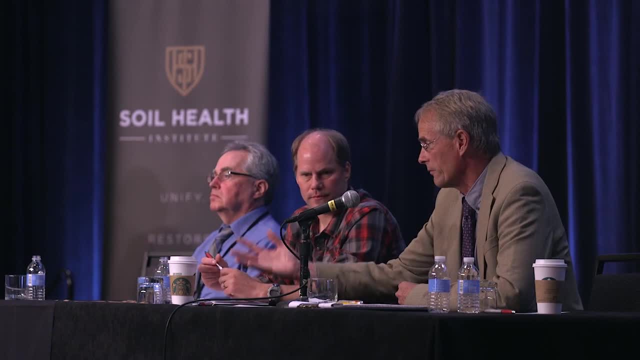 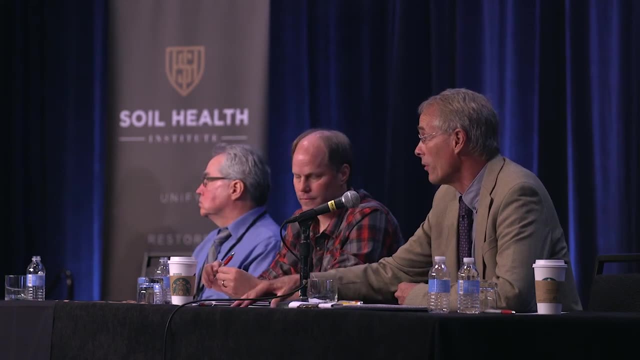 progress in soil carbon sequestration for for greenhouse gas reductions, but also if we're going to look at at, at management and and and monitor the health of our soils. as we adopt different practices, We're not going to. 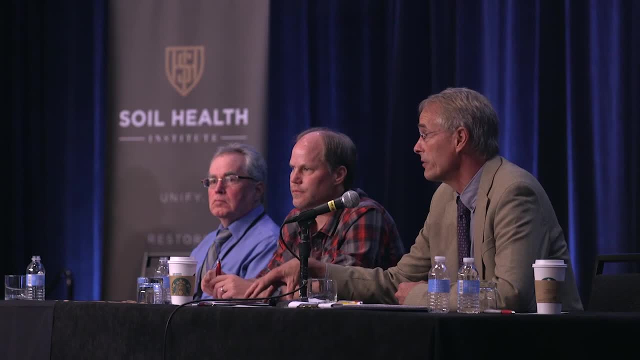 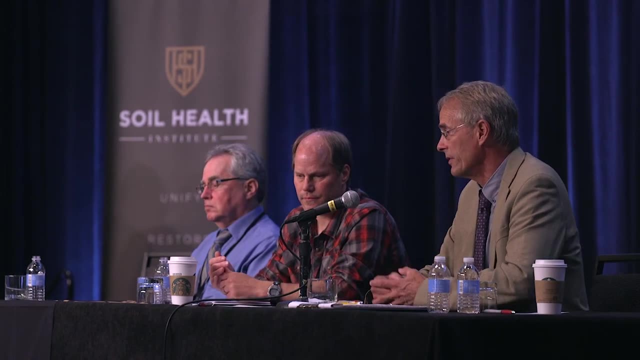 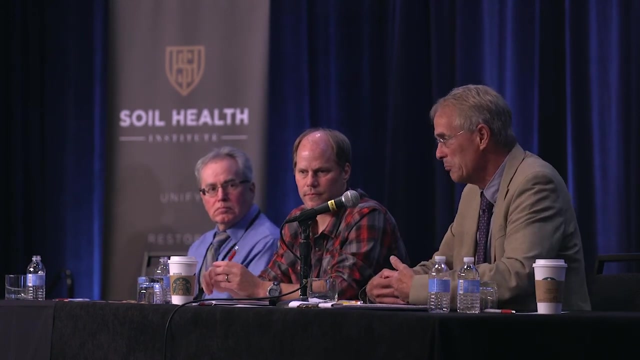 We're not going to be able to do that and and do direct measurements on every farmer's field every year, or something like this, or we're going to completely take all the the, the resources that need to go into this, into into, you know, billions and billions of lab.